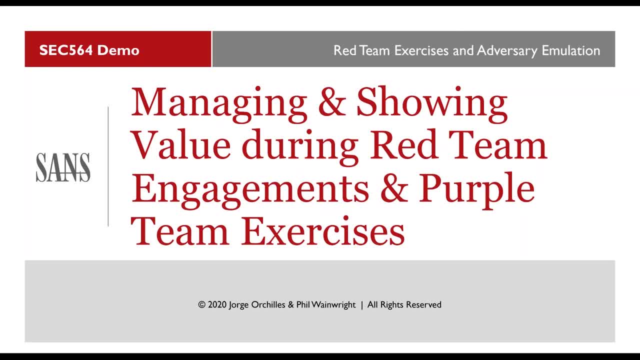 going to talk about managing and, more importantly, showing you how to manage and show you how to manage and show you how to manage and show you value during and after your Red Team Engagements and Purple Team Exercises. I'm joined by Phil from Security Risk Advisors, who we've been working together probably two years now on. 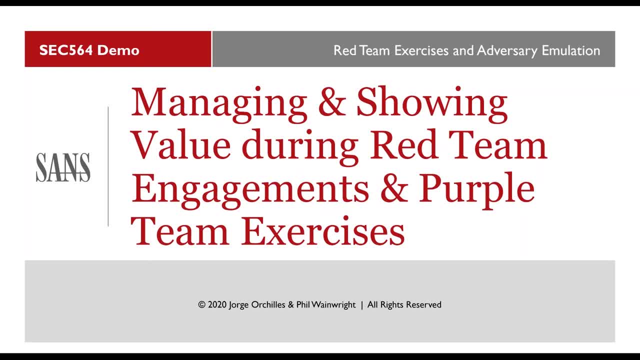 Vector and being one of the bigger users of Vector, giving feedback and really working together to make this even better for you. So we are very excited to be here today. We're going to talk about managing and showing value during and after your Red Team Engagements and Purple Team. 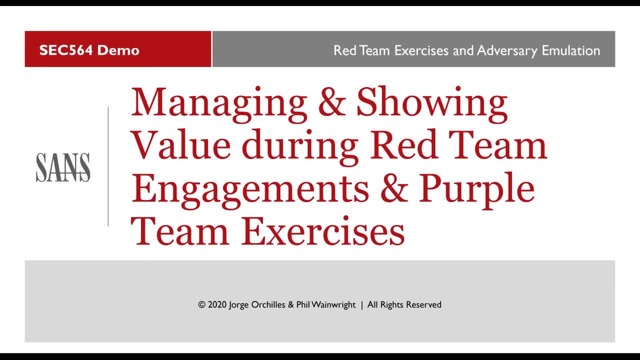 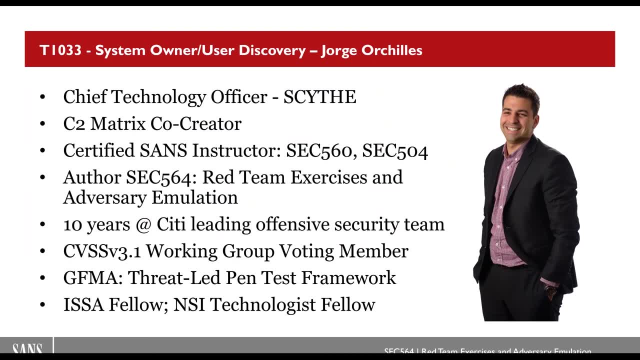 Exercises, So happy to share this with you, And we've actually probably been talking about this webcast for two to three months now, as a new version of Vector was released. So I am George Orchillas. I am the Chief Technology Officer of Scythe. I'm also the co-creator of the C2. 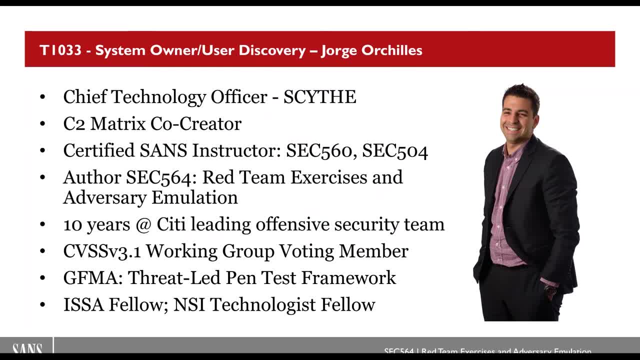 Matrix, which is the command and control matrix. I'll talk about that shortly. I am a SANS-certified instructor. I teach the pen test curriculum, so Security 560.. I'm also the co-creator of the 560.. Shout out to all of you with G-Pens and Security 504.. Shout out to those with GCIHs. I'm 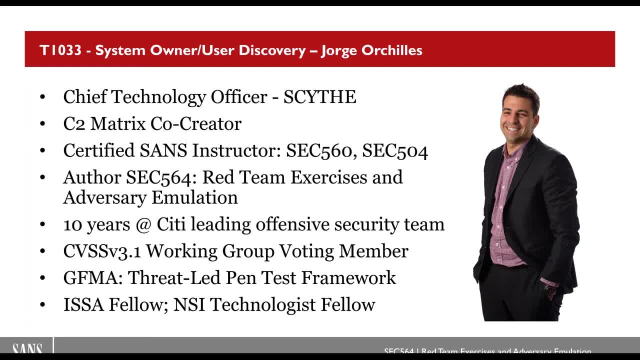 also the author of a two-day course: Security 564,, Red Team Exercises and Adversary Emulations. We're actually going to be giving a quick demo of that. A few slides straight from the course. and the course also covers Vector, So you will see a lot there. I was a 10-year veteran at Citi. 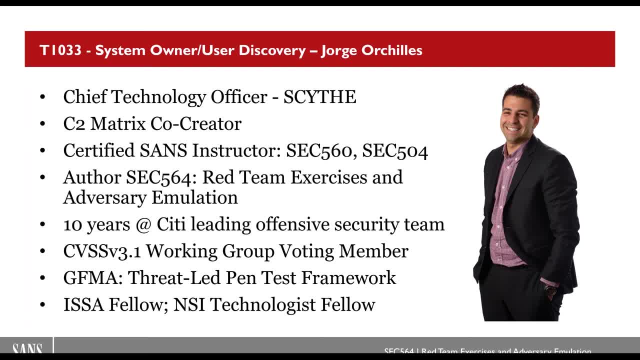 leading the offensive security. I worked as part of the Common Vulnerability Scoring System working group and also a voting member for version 3 and 3.1, which is the most recent. I helped co-author a framework for doing red team engagements. It's called the Threat-Led Penetration Testing Framework for regulatory use. 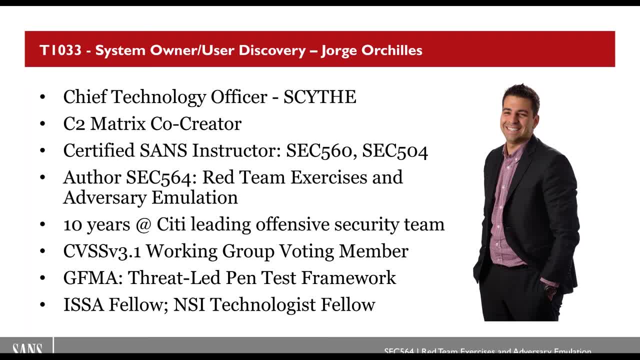 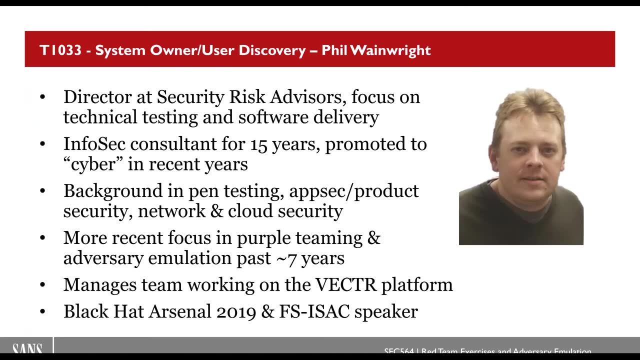 in the financial industry space. Also a big fan of ISSA, Shout out to all the ISSA members out there. I was privileged to get the ISSA fellow designation just last year. I'm also an NSI technology technologist fellow And with me today I have Phil. How are you doing, Phil? 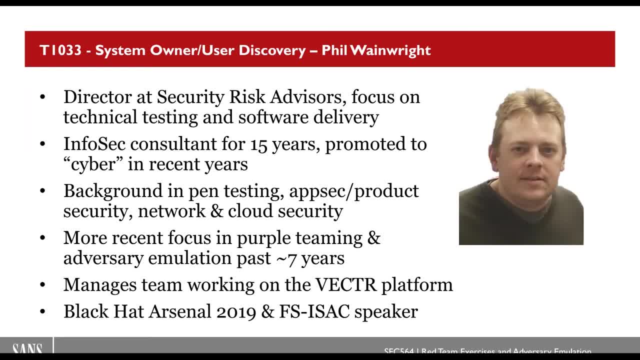 Doing very well, George. Yeah, great to be here talking about Vector today. Just in terms of overall background, George, it's been a while since we had a chance to actually meet in person back at the SANS Purple Team Summit in 2019.. So that was you know, really. 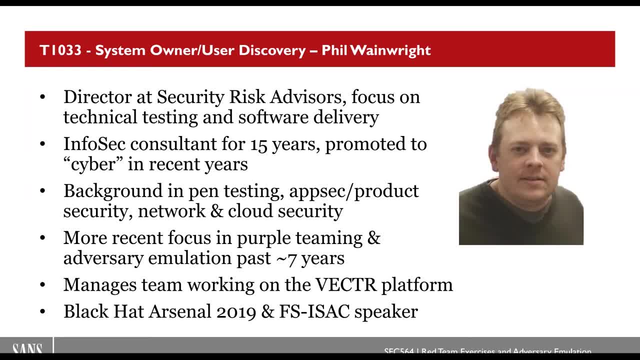 really excellent event, Looking forward to this year's, whether it's in virtual fashion or physical, but yeah, really great event. So, in terms of background, hi everyone And thanks SANS for having me today. I'm a director at Security Risk Advisors- My main focus. 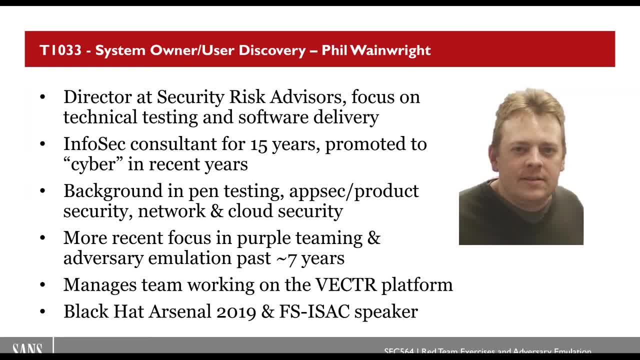 I've been doing information security cybersecurity consulting for roughly 15 years. My background is mostly in pen testing, red teaming, application security, cloud security, Other areas. as of the past- you know seven or eight years- I've been getting more into the. 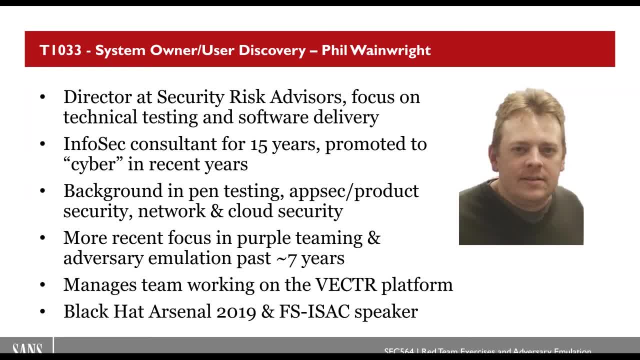 concept of adversary simulation and purple teaming, you know goes by a couple of different names which you've probably heard George talk about quite a bit. And really this you know, back in really not too long ago, really this was happening more in spreadsheets. It was fairly 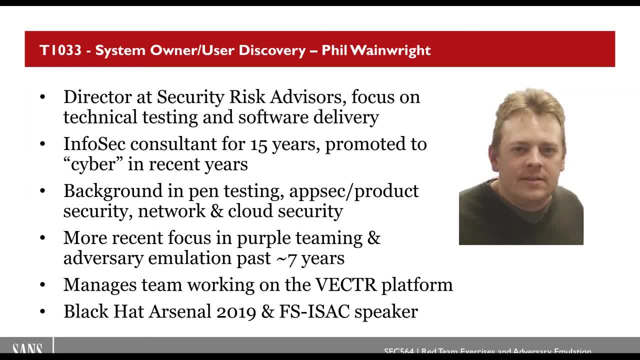 not super well managed And we certainly learned a lot- gave us inspiration to really start building a platform that allows better collaboration, Better sharing, better planning and metrics. So I also actively work on the Vector team. I work with a very talented group of developers, you know, working on the platform, continuously adding. 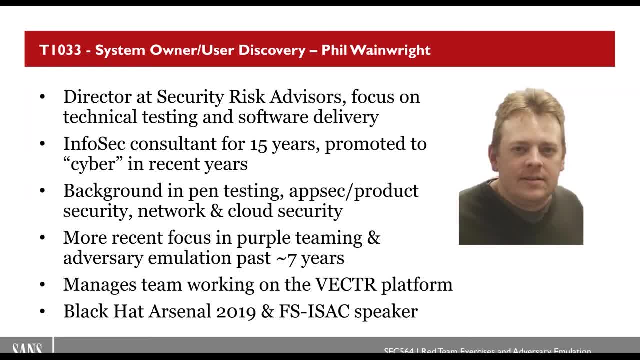 new features, taking feedback from the community and our own team. So we're really excited where Vector is going, Hopefully. you know we want to make this, make today really interactive with the demo And we also have more information in the slides as more of a lead behind. 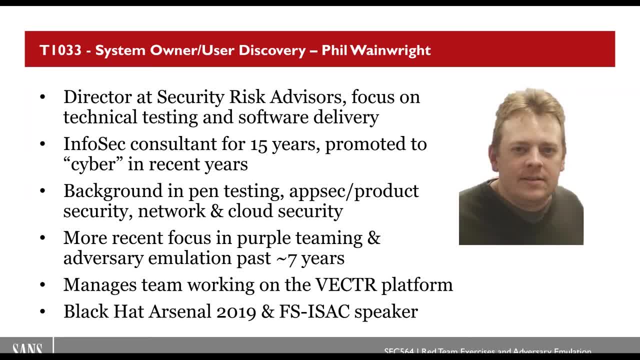 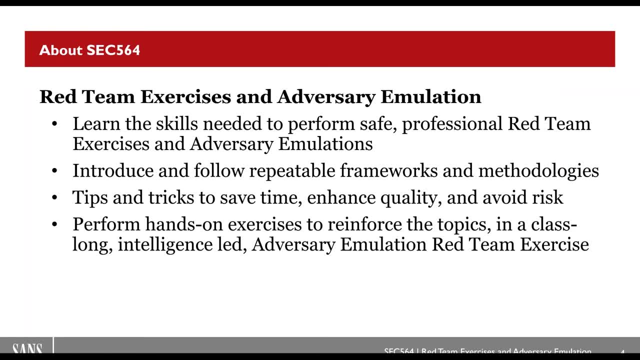 Awesome. Thank you for being here and taking the time. So just real quick, I'm going to do. the way we're going to do is just cover the course a little bit, because Vector is featured in the course. It comes in the virtual machine. 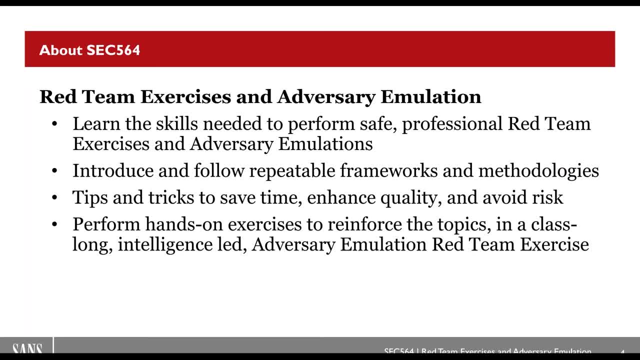 That we give students. We give students a Windows virtual machine and a slingshot. If you're familiar with the SANS Slingshot, it now has Vector, which is great, And we actually cover this in the course course. so this is really a demo of the class where you learn how to do. 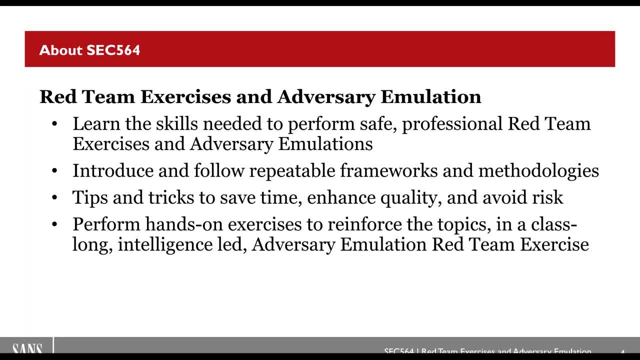 professional red team exercises and adversary emulations. it's 50% hands-on and 50% lecture, so we spend quite a bit of time actually doing a class long adversary emulation. we emulate APT 33, we gather cyber threat intelligence around them and we go against a target organization. there's eight virtual 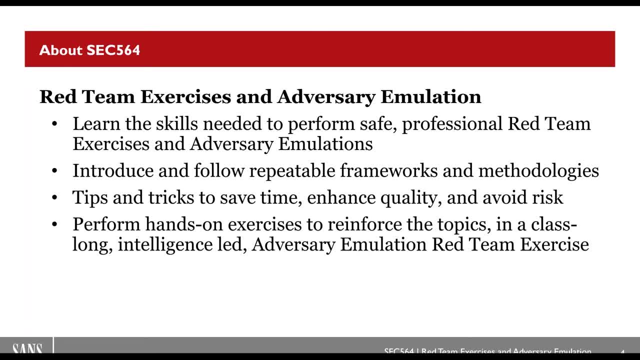 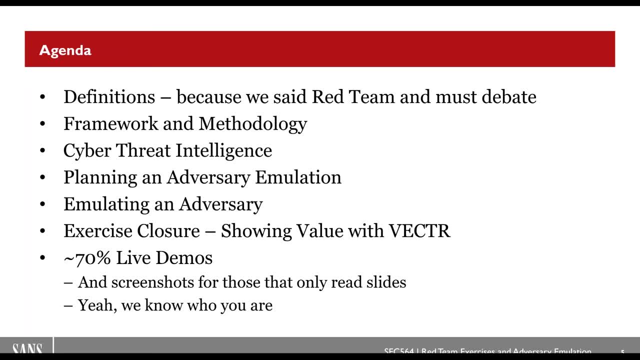 machines. so it's a. it's a jam-packed two days, the famous sans firehose effect. so real quick. what are we gonna do? I'm gonna talk for about 10 minutes, just kind of introing. if you've never done red teams or never done purple teaming, 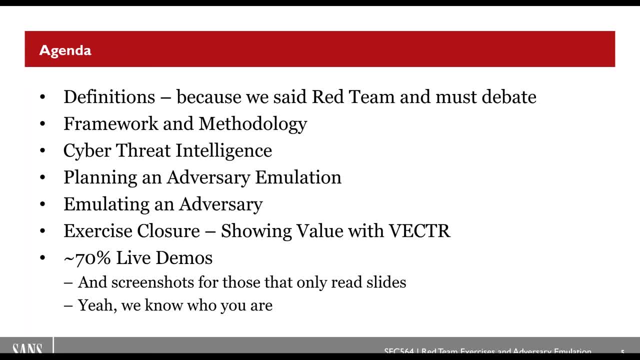 I'm gonna cover what that is and then we will spend the rest of time with Phil showing the latest version of vector and doing live demos. so, like anything, we'll start with definitions. just make sure we're all talking the same language. we'll cover frameworks and methodologies if you are going to build. 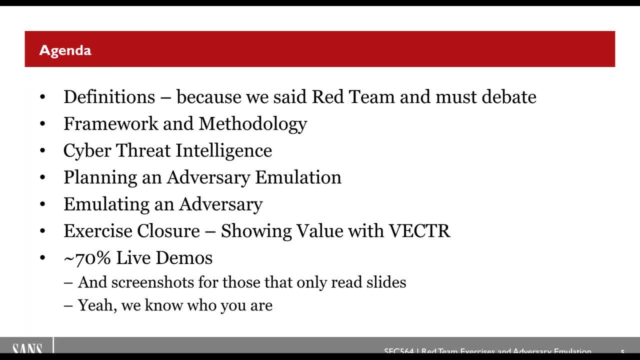 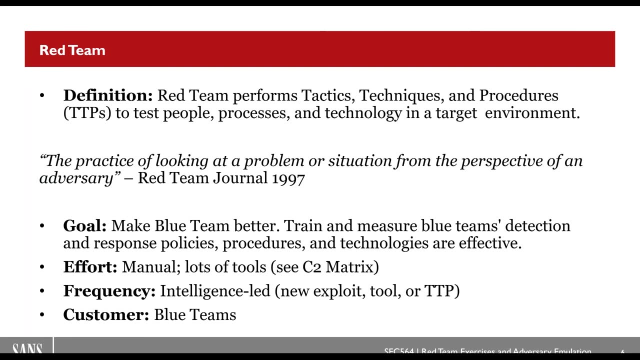 this professionally. you should follow a methodology. we're gonna cover the importance of cyber threat intelligence planning an adversary emulation- actually emulating an adversary- and then showing value, and that's where I'm gonna hand it over to Phil. so real quick here. we can't have a red team talk without debating. 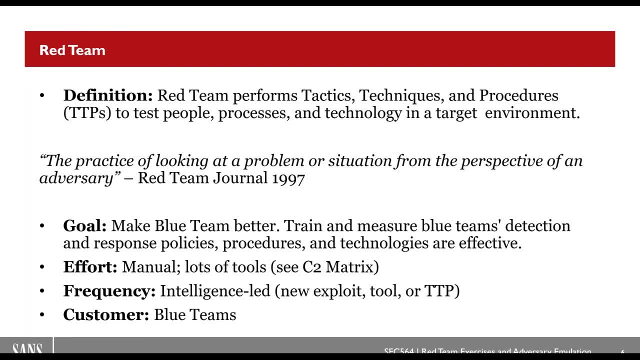 the definition of red teaming- and I like the red team journals definition, which is that Red Team is the practice of looking at a problem or situation from the perspective of an adversary and really the difference here from other types of offensive and ethical hacking type of assessment is that we are 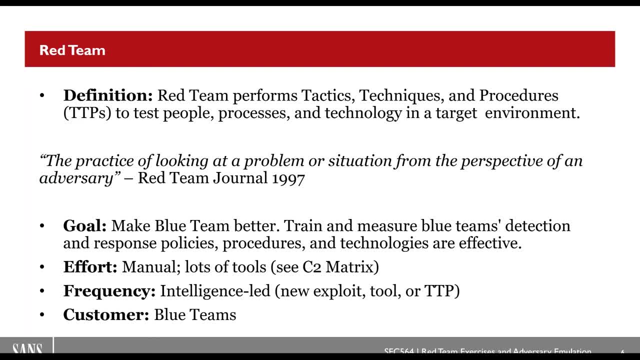 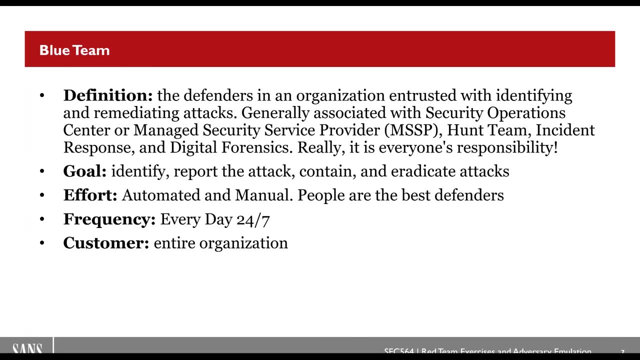 testing not only technology, but people, process and technology. our customers also different. we're not really finding vulnerabilities on products. our customer is blue team. and what is the blue team? well, the blue team are the defenders. we love our defenders, we want to work with them and really block attacks and stop attacks and generally in an organization. 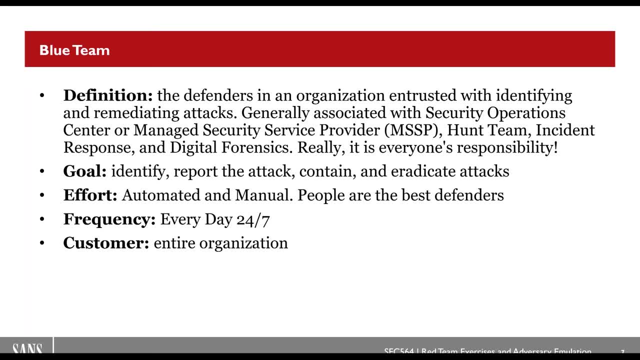 you have a security operations center or maybe a managed security service provider. you may have a hunt team, you might have an incident response team or forensics. really I'll debate that. anyone in organization is really the blue team, because if you get an email, even if you're in accounting- 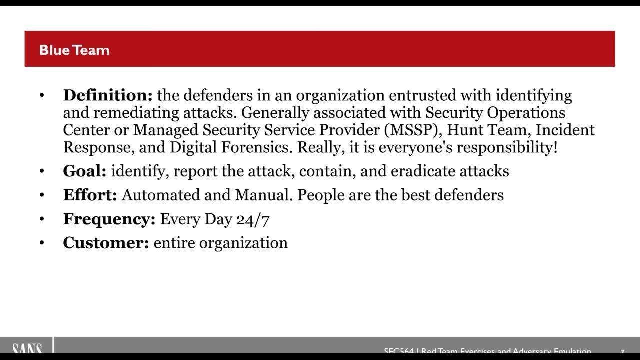 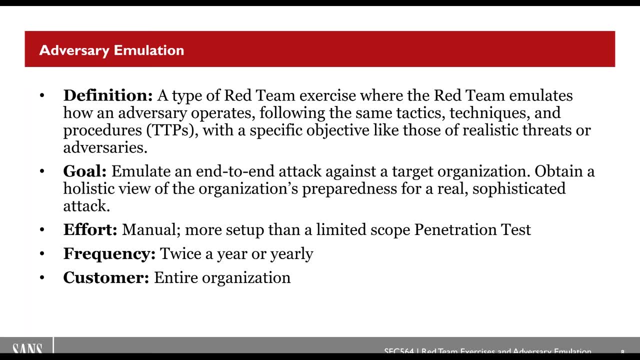 you should report that email and humans are the best sensors. so that's the blue team. adversary emulation is a type of red team engagement and there are many types of red team engagements. adversary emulation is the one where we understand how an adversary operates. we map to the same. 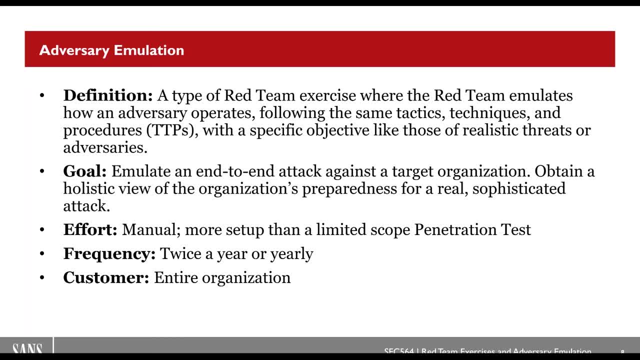 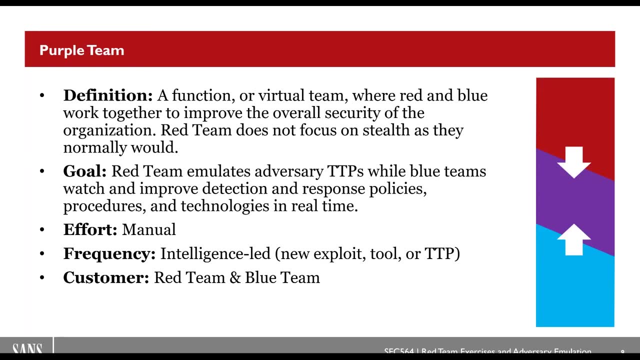 tactics, techniques and procedures they, you, they do and we emulate those. that means we actually go out and try to do the same thing against a target organization. this brings a lot of value to that organization because it can measure if they are ready for a real attack. and lastly, here on definitions, we cover the purple team. I know we're very creative in. 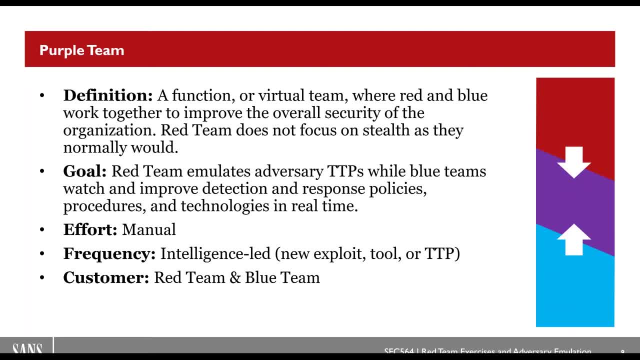 information security right. where did the name come from? well, you mix red and blue and you get purple right. and a purple team is a function or a virtual team where the red and the blue team work together. see, a lot of red team engagements are what we call zero knowledge to. 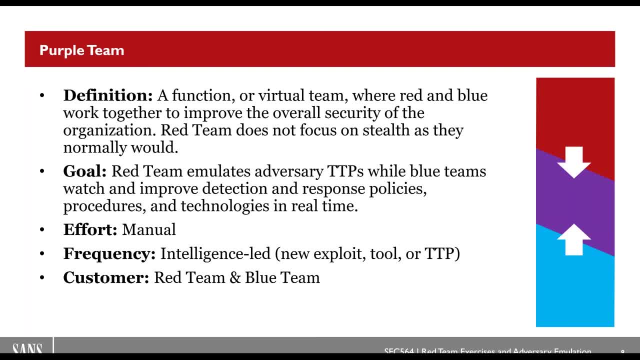 the blue team. the blue team isn't aware of this. in a purple team engagement they are, and what we do is we present a particular attack chain or scenario and we emulate that in front of our defenders and from the blue team, and then they can go more efficiently and tune their security. 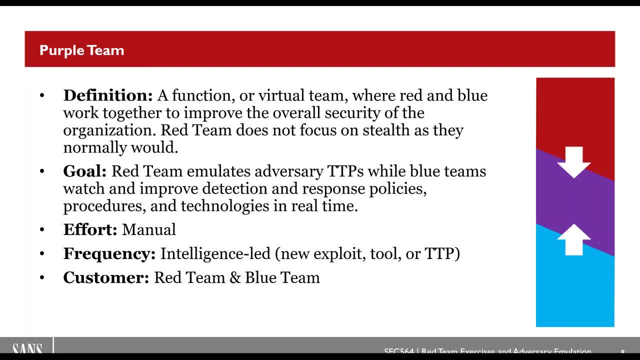 devices to make sure that they can catch those particular TTPs when they come together. so purple teaming is fairly new. Phil mentioned that. tell me what we met was actually the inaugural purple team summit. so SANS did that last year, we're going to be doing one this year as well and of course, we'll invite all of you to. 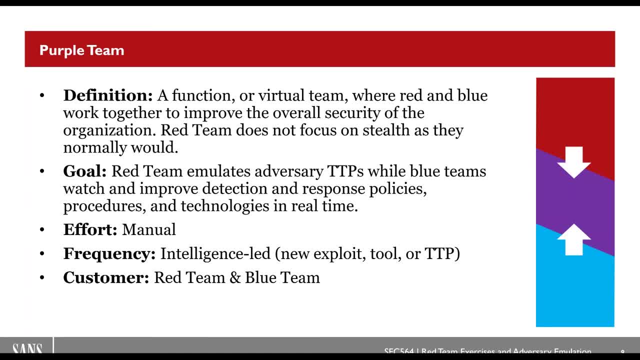 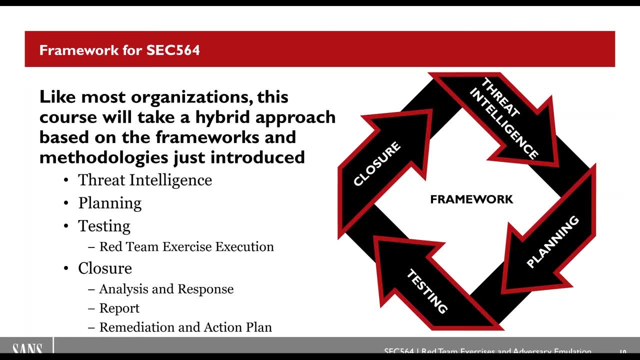 that because it is very valuable and just shows how our organization and our industry has matured. so for the course, there's a lot of frameworks. I cover a lot of them. I personally co-authored one of them, but at a high level we learn about threat intelligence. 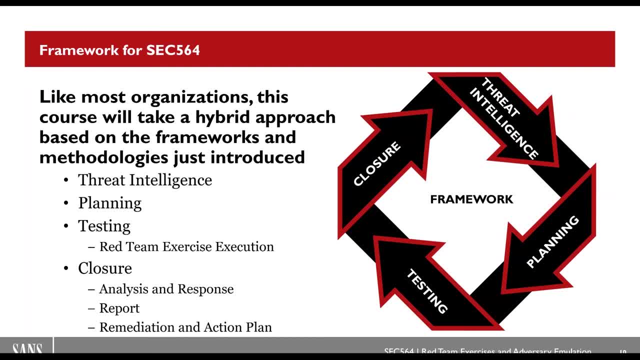 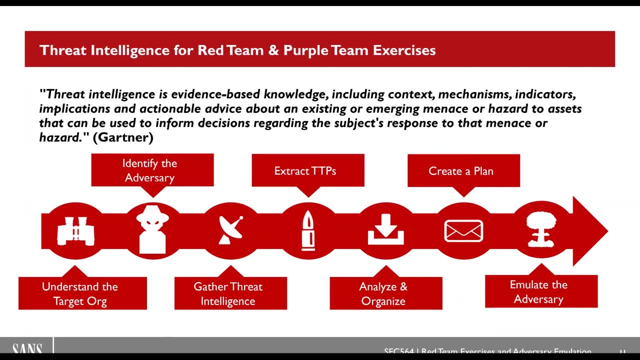 we then plan the exercise, we test and then we do exercise closure, which is really going to be most of our focus today from a threat intelligence space. we do need to leverage that in adversary emulations. we want to understand the target organization, we want to identify a adversary. 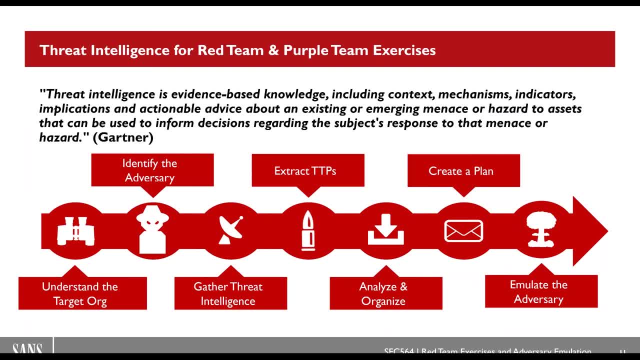 that has the opportunity, intent and control to do that. so we're going to be doing a lot of that. and capability to attack the target organization- and every organization is different. we then gather threat intelligence, we extract the tactics, techniques and procedures, we analyze and organize that and then we create an adversary emulation plan. so this was derived actually from another. 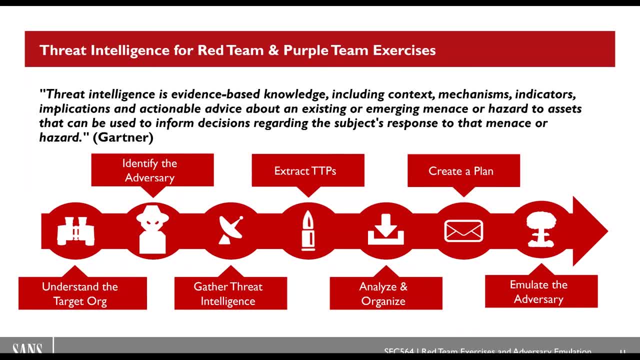 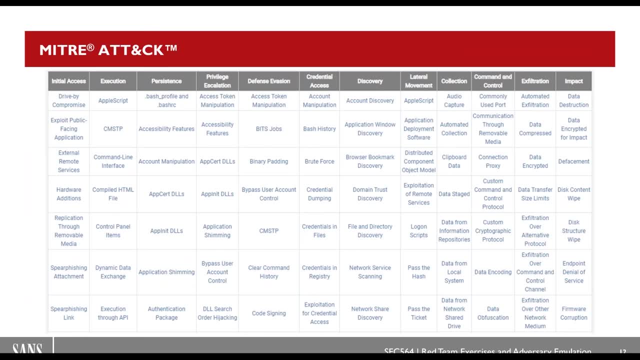 SANS summit where Katie Nichols and Cody Brown, who were both at MITRE at the time, published this. so thank you to you all and we have continued to use this process that MITRE created and MITRE, of course, mandatory MITRE attack matrix slide where we use: 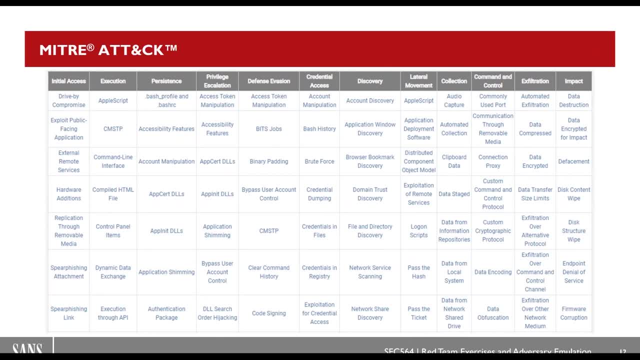 this as one of the main frameworks, at least the testing framework, because it is a common language. it stands for adversaries, tactics, techniques and common knowledge and allows cyber threat intelligence- who's providing us information about an adversary, the red team who's emulating an attack on the blue team that's defending? to all speak the same language. so in 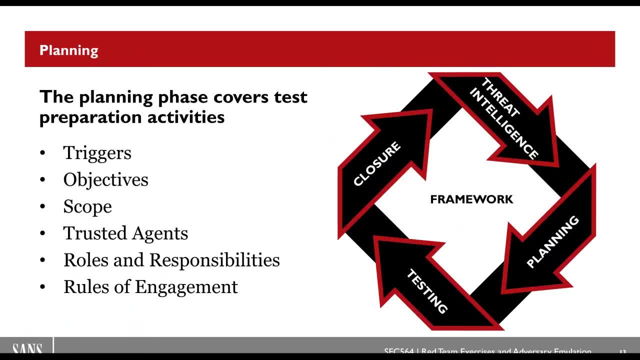 the planning phase we covered a lot of things. we cover what triggers and exercise. what are the objectives? because, just like adversaries, your red team engagement, our purple team exercises have objectives. you have a scope, you have trusted agents. if you're doing a zero knowledge assessment, then, while the blue team and responders on the ground do not know what, there's certain people in the organization that shouldصل可能erman. 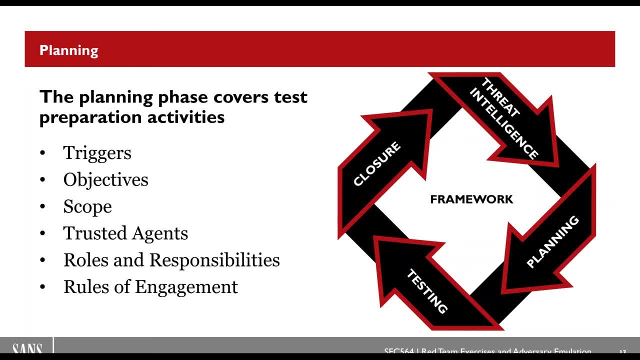 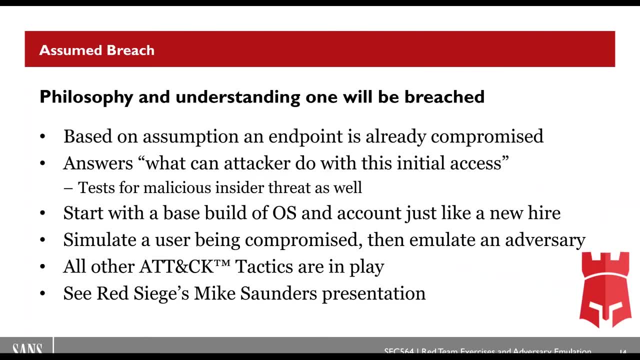 instagram. We cover roles and responsibilities and roles of engagement. One of the things I do want to highlight here is assumed breach, And that is a philosophy and understanding that your organization will be breached right. Eventually, you're going to have a vulnerability that you didn't patch quick enough. 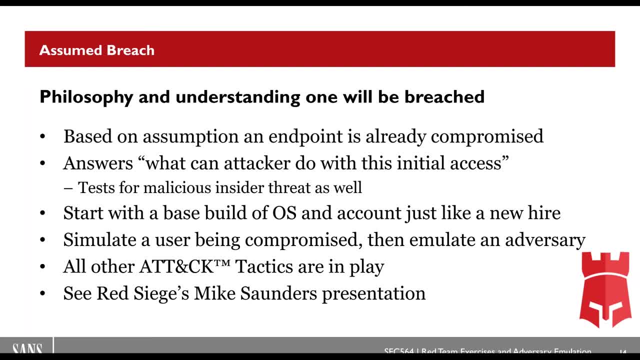 So somehow some new exploit worked right And we have plenty of classes on that. Same with social engineering. Someone is going to fall for some social engineering attack and might execute a payload. So one of the things that we're seeing more and more in consulting companies and even internal red teams, is operating under that philosophy. 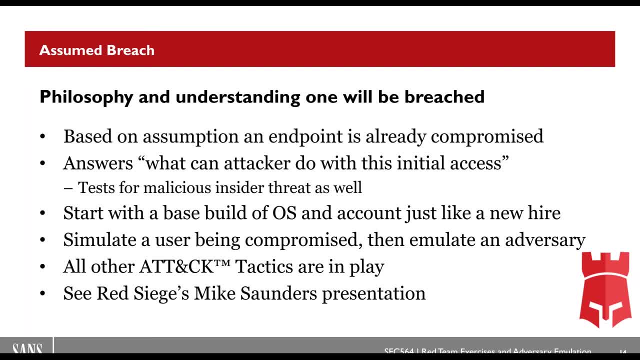 So, if you saw in MITRE ATT&CK, initial access is only one of the various tactics. We want to spend more time with what happens next. A big shout out to Mike Sounders and Tim Medin from Red Siege. They have an awesome presentation on assumed breach and I really think you should leverage that. 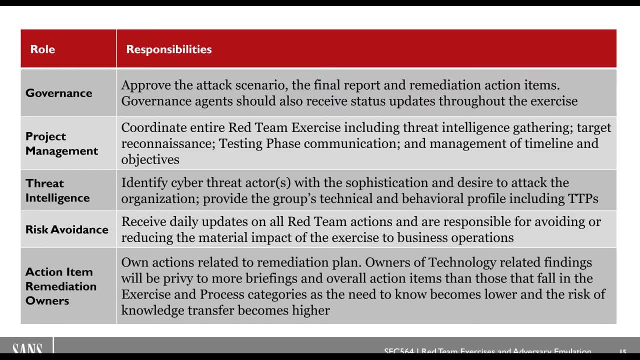 In your organizations. this is a quick slide on roles and responsibilities. Phil Phillip on Twitter asked me about this the other day. He's running or building a new red team And just a quick highlight here is to have a project manager or exercise coordinator. 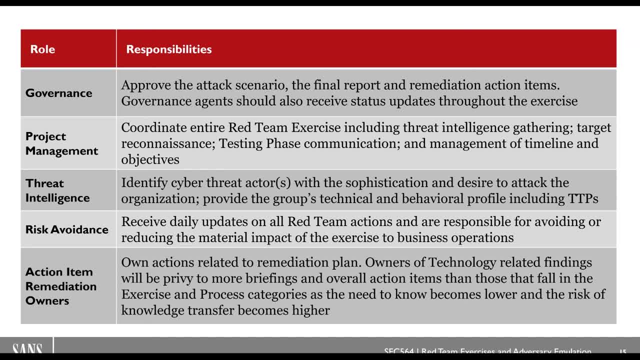 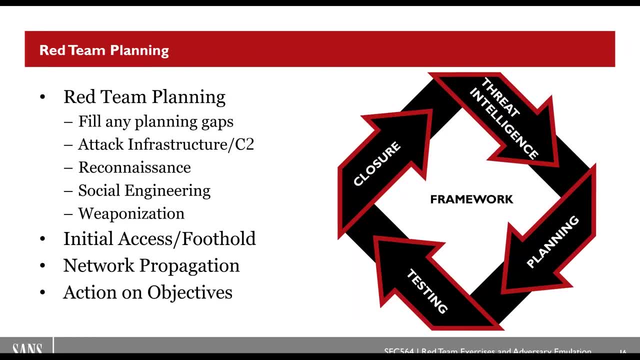 Most of the time, you're going to try to do this as a red team lead or red team manager. You should really have an exercise coordinator, because there's a lot of moving parts. Then, for red team planning, you need To fill all the gaps that the cyber threat intelligence did not provide. who are you going to fish? how are you going to fish them? 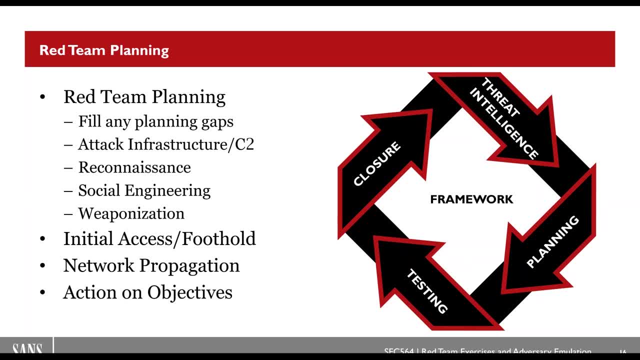 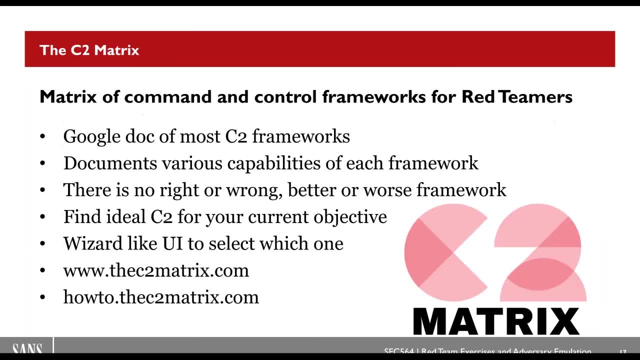 who are you going to social engineer? you need to set up attack infrastructure, set up command and control, perform that reconnaissance, weaponize and then you get to the testing. One of the things we cover is the C2 matrix is a command and control matrix. 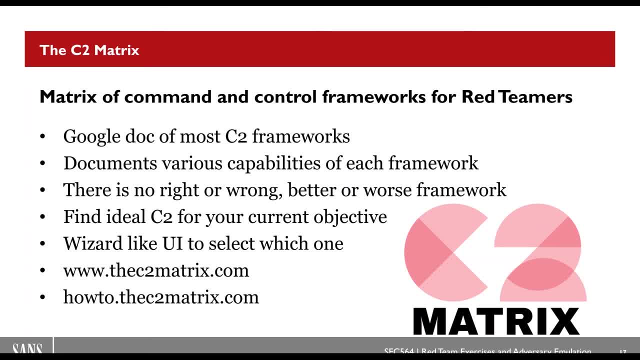 It is a list. There's 48 C2s documented there And really the reason we do this Is because you don't just want to test with one tool, right? You want to test with all of these, especially if they are open source or if they're freely available. you should definitely test the tools. 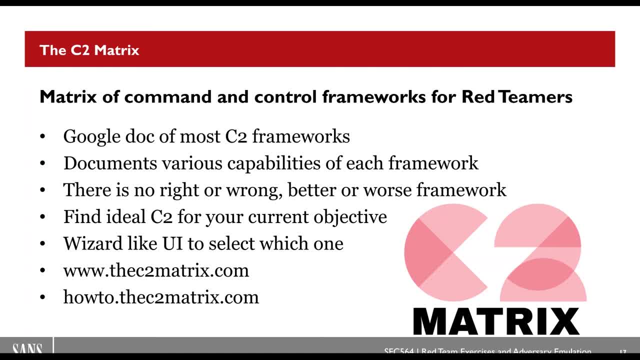 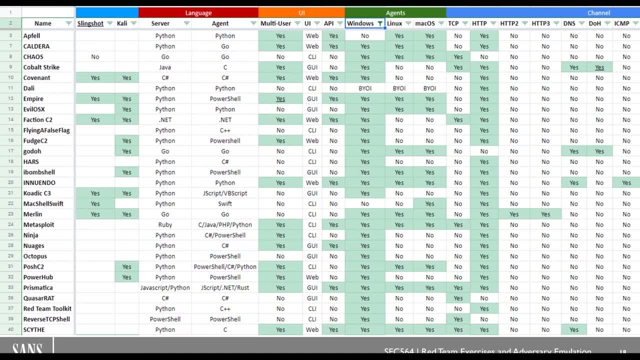 But what we really want to get to in these tests is that TTPs the attack behavior. So this is a quick screenshot of the C2 matrix. We have a sans slingshot C2 matrix edition that comes with eight of these C2s already installed. 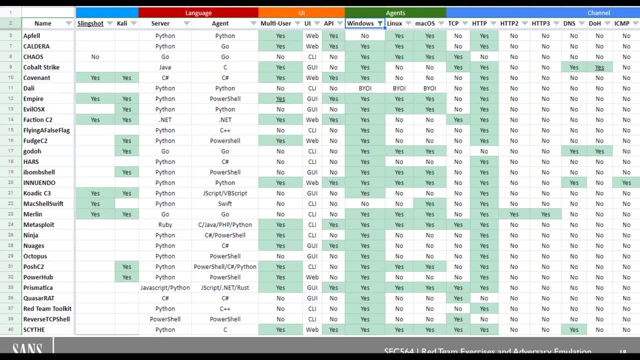 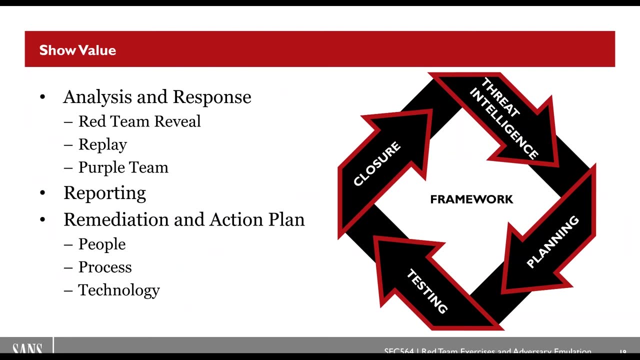 So you can actually download this VM. It brings vector as well. Believe that we have version 5.5.7.. So you can get started literally after this call and test some of these things in your lab. So with that, let's talk about showing value, which is the last part of the course. 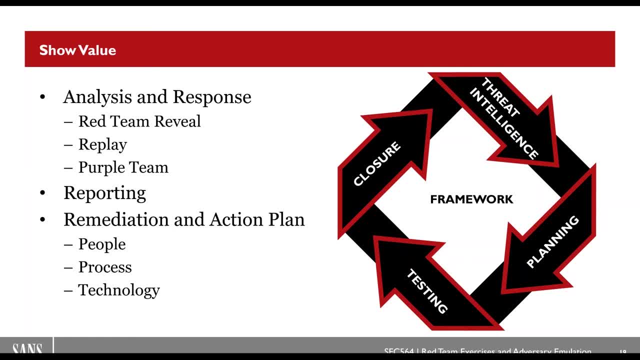 It's about a fourth of day two And we do spend a lot of time because the entire reason you're doing a red team or a purple team engagement Is to bring value To the target organization. right, We're not just going full cyber and breaking everything, getting in and leaving a report behind and laughing in people's face and leaving. 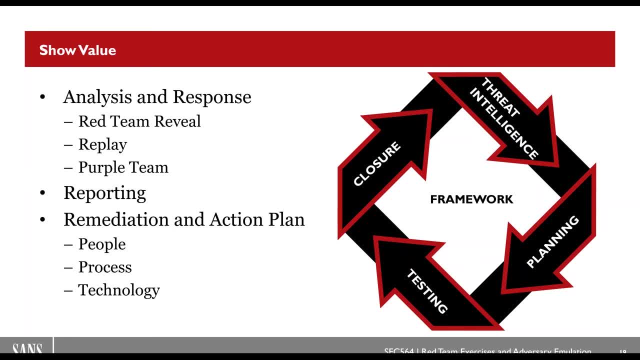 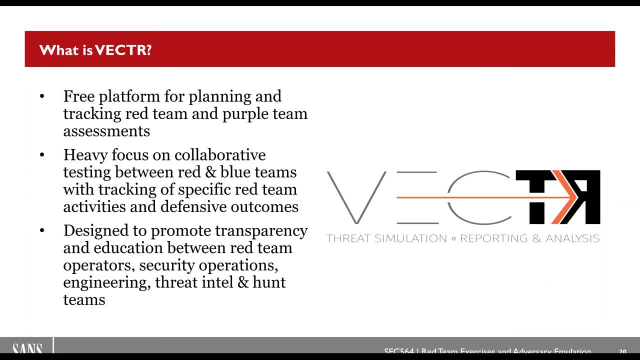 That's wrong. right, And I know some people do that, but that's wrong. You should not do that. You need to work together. We're all in this together. So one of the methods of doing this is with vector, And I'm going to turn it over to Phil to just cover a couple slides before we just do demo the rest of this webcast. 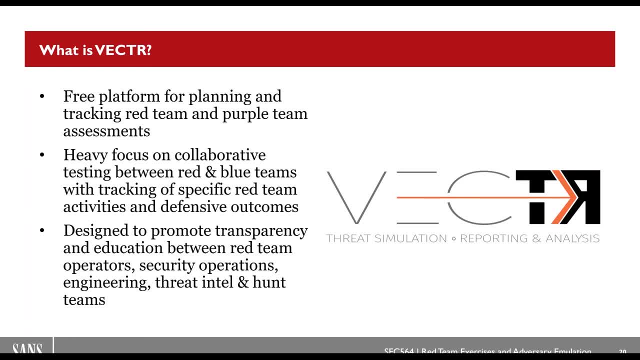 Hey, thanks, George. Yeah, so what is vector? vector is really a free core platform that you can, you can start using today for planning of both. you know: red team assessments, purple team assessments, adversary emulation, other custom types of assessments you might be getting into like, hey, how, what is our cloud environment look like? what kind of parity do we have between our on prem and cloud environments? 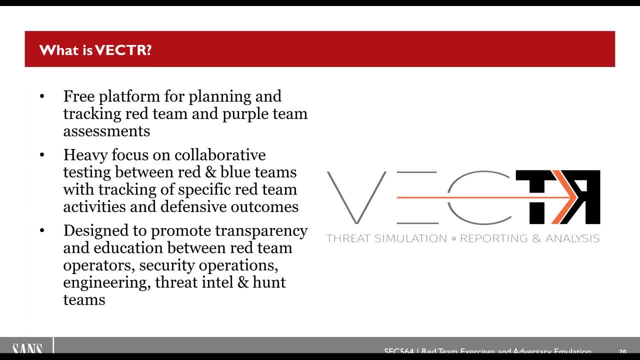 So really there's a big focus on on that purple team concept, True collaboration Between red team operators. you know pretty much anybody on your infosec team connecting all those roles, really promoting education. So you know, I don't know how many pen tests red teams you've probably seen, or just you know very red reports by the nature of them, with very little knowledge sharing on. 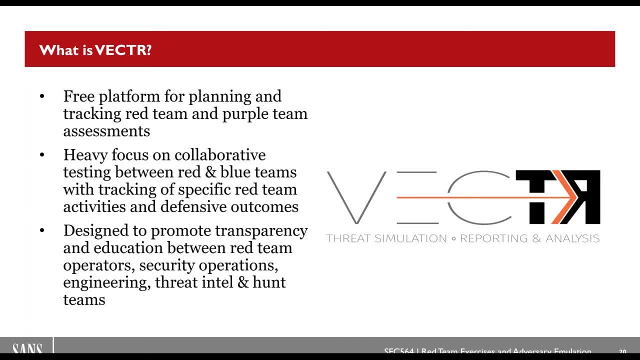 OK, what do the actual TTPs look like? What do the tools, what do the actual command lines look like? What should we be looking for in our SIM and our EDR tools and elsewhere? So vector is really meant to To provide that level of sharing and, you know, as much transparency as you can possibly do within your organization. 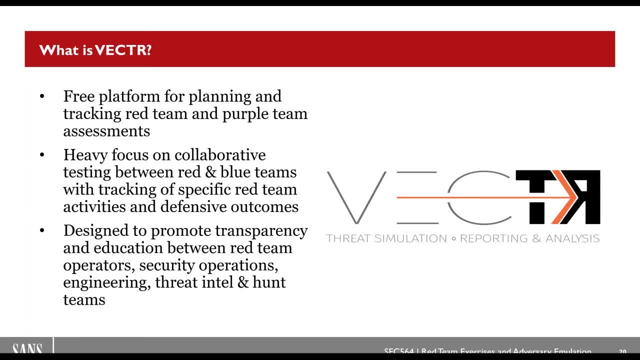 And we've also seen so originally. you know purple teaming is a major use case for vector. We've seen a lot of increased interest from threat Intel groups in particular- really different functions, And you know we're increasingly adding more, both red team planning, tracking capabilities, but also increasing the value of vector to blue teaming. 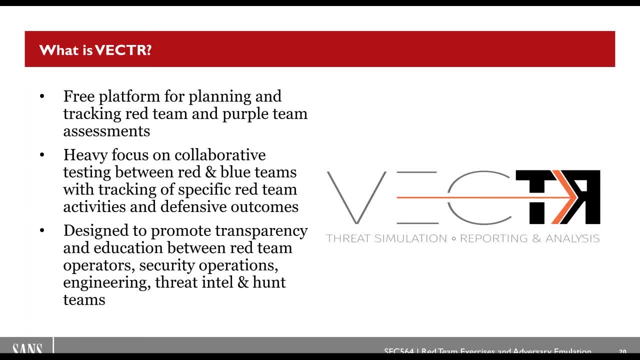 So providing more, more information, like: hey, what are some useful detection rules, analytics to get started with fixing some of these problems? So, based on the framework you outlined, George, I think you know the core concepts really tie in very well to vector and what we're looking to do. 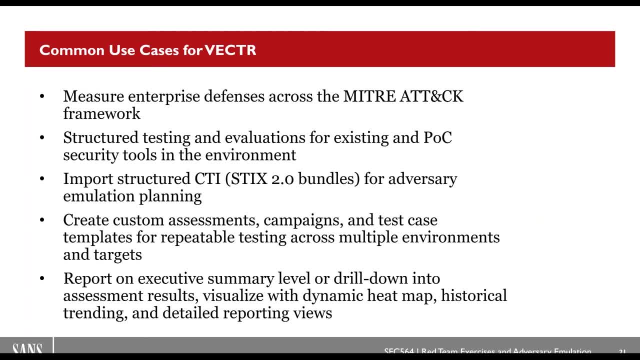 Go to the next one. So common use cases: alignment to MITRE ATT&CK Enterprise, the very big one. You know many of you are probably actively working on this or have been for some time. Some are still initial and getting started, but we want vector to have as much alignment to ATT&CK as a- you know, a common for common terminology: taxonomy for how you're tracking and measuring your progress across your organization. 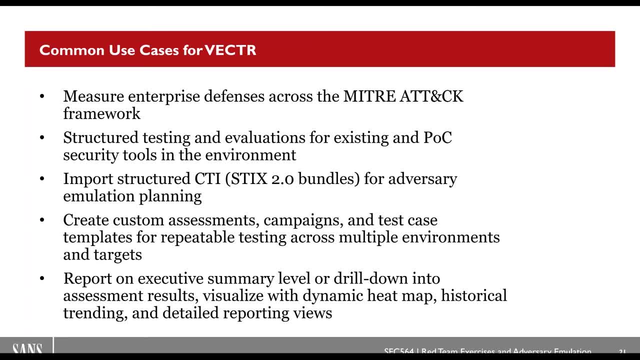 We want vector to really promote, you know, unlike a red team which is meant to be a lot more stealthy, really providing a structured methodology, So forcing some documentation as part of that knowledge share. We also use it a lot for just doing POC evaluations for tools. 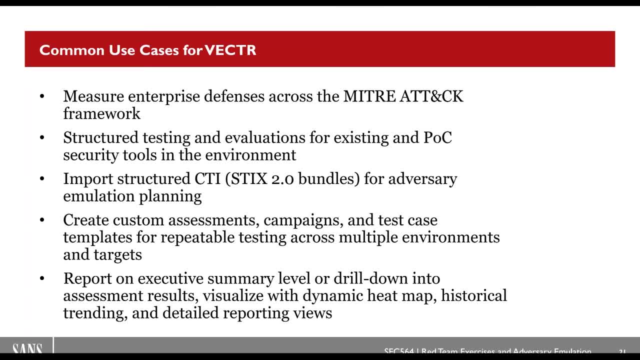 And, of course, by the nature of purple teaming, a lot of those tools are the live ones in your environment, Just looking to get a sense of: okay, how good is our sim doing? How good is our behavioral anomaly detection? 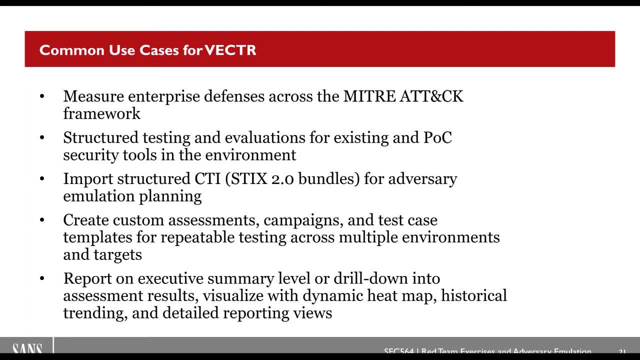 Whatever that detection control might be, Some other major use cases really using vector. It's really a CTI-backed platform, so a way to directly bring in great content from places like MITRE, Red Canaries, Atomic Red. It's a really great third-party open source project that you can pull in and start using right away. 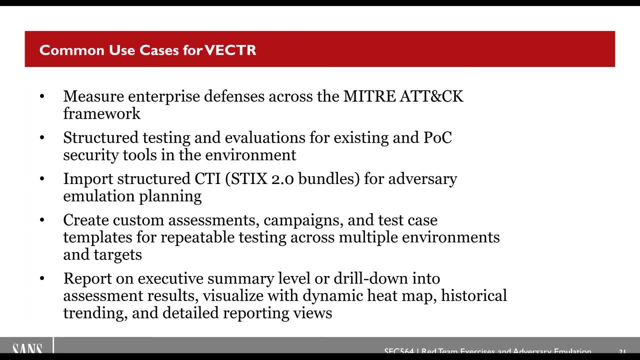 And another one here just the idea of creating good templates. So everything in vector is kind of organized. You can have major assessment groups, logical groupings of campaigns and then individual test cases that make up those campaigns. Really, what we're big on is making vector a very useful test case tracking tool that can be used for a lot of different purposes. 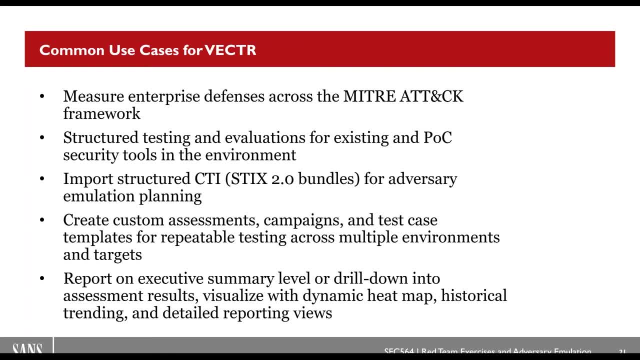 So being able to save off those types of templates, replaying those you know, across different business units, different geos that you have, So promoting really a repeatable methodology that you can continually evolve over time And, of course, reporting. 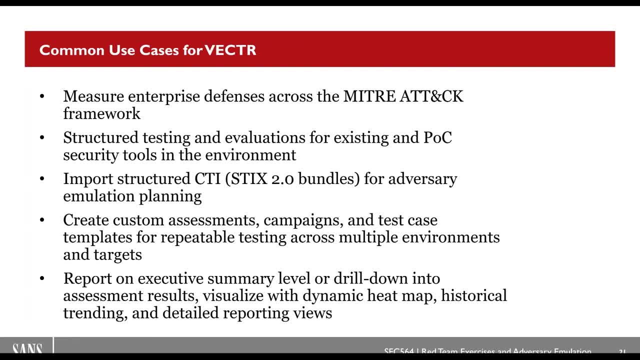 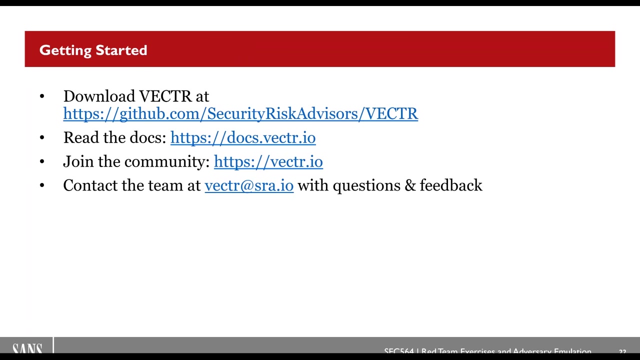 I will show you a lot of the reporting dashboards in vector Really showing: okay, we did this one red team exercise, but now we've done five purple team exercises, a bunch of other custom assessments. How do you visualize all that data? drill down into areas of interest to really prioritize and frankly show management what your program looks like, help to justify investments in- sometimes new or better- tools and personnel needed to meet your mission? 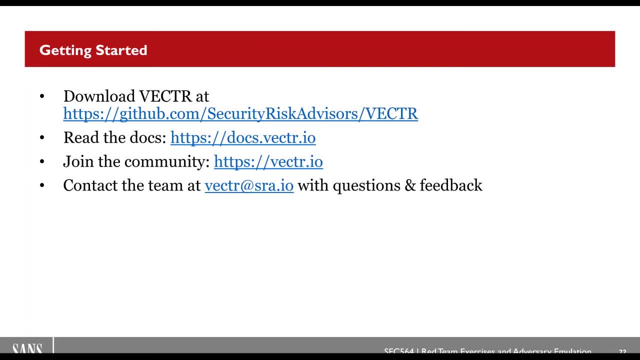 So, yeah, So getting started, this is the last slide I have. you can check out vector at our at our github page. also check out the the documentation site for additional guidance on installation and usage. You can sign up for the community. 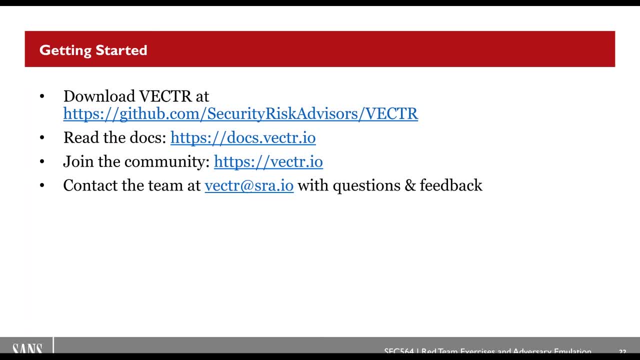 We have a mailing list where we're not too spammy here We we generally reserve that for major releases and to provide a preview of any major upcoming features that we're working on. And, as usual you know, feel free to reach. 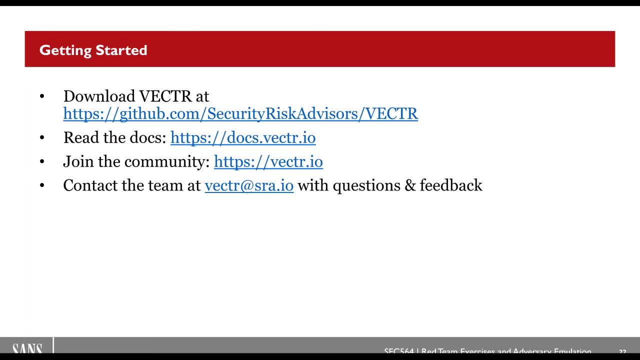 Any time at vector at SRA IO. we've really been very appreciative of all the feedback that's come in so far. with the community We have a great laundry list of items that we've added to the roadmap, So definitely contact us there if you want to discuss anything in more detail. 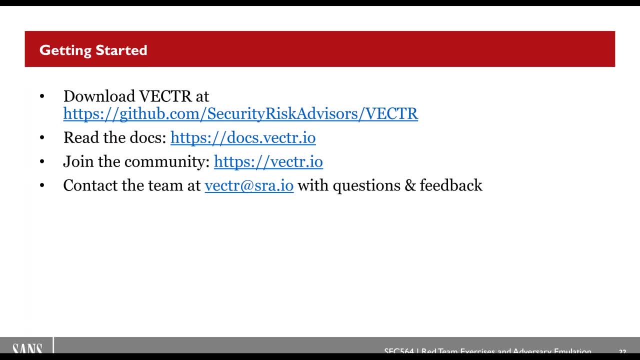 All right, George, so I can start presenting here. Yep, I'm making you presenter now And Just FYI, I am monitoring the questions, So you've actually probably already seen me respond to some of them. So, as Phil does the demo, feel free to ask other questions. 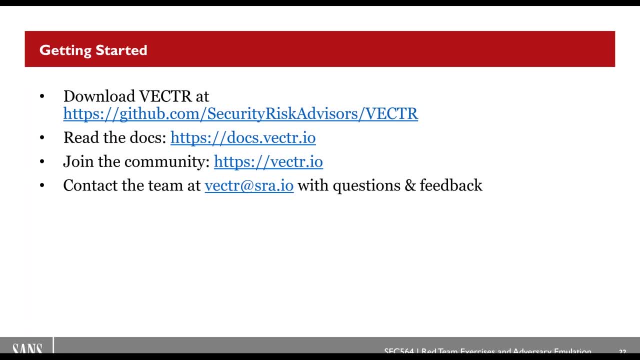 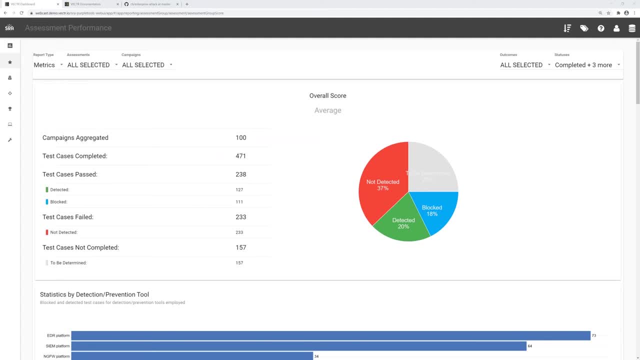 We will leave maybe five, 10 minutes at the end. if you have any questions for us- And we have one here that I actually don't know the answer to Phil, And that question is: is this the same Phil that authored the Oracle security publication? 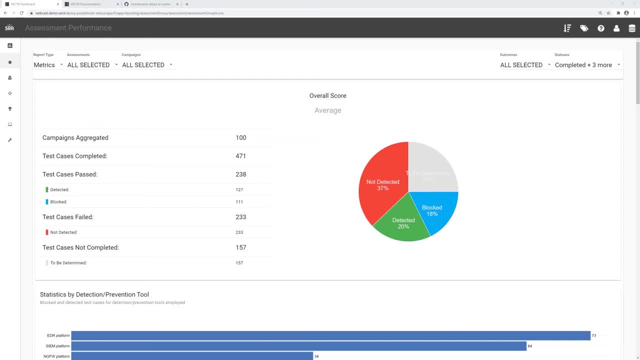 That's. that's not something I like to talk about, At least. But yes, yes, that was in another life. Yeah, Yeah, It was a Oracle 10 G. So if you ever, if you ever need some nighttime reading material, but I think a lot of the concepts are probably still pretty relevant to Oracle security. 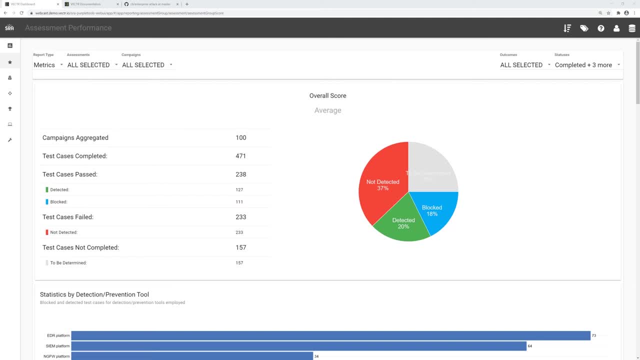 But yeah, that's the blast from the past. I'm not sure who, who, who raised the question, but Yep, That is funny, Awesome. So we can see your screen, So go ahead, We'll do demo now. 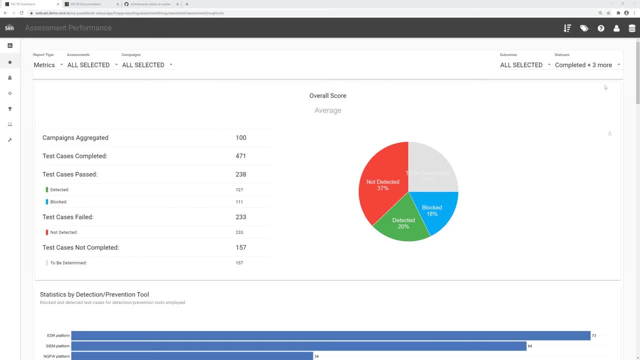 All right, great. So this is coming through. like I mentioned previously, you know vectors really made up of, really the. the main hierarchy is you have assessments which are a little bit more comprehensive. In this example, you're looking at the, the overall reporting dashboard. 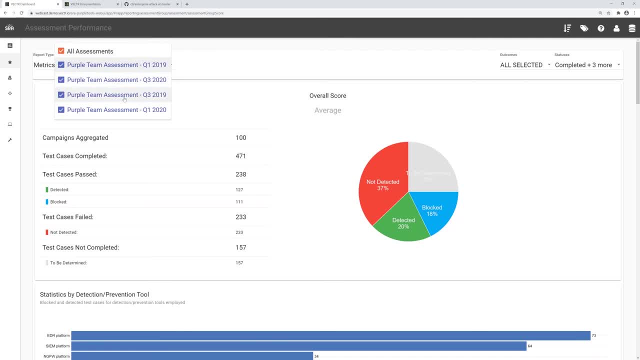 You can see we have four sample what we'd call major purple team exercises that are that are roughly six months apart. We also have a number of different report types that are here. So what you're looking at is Is the metrics view. 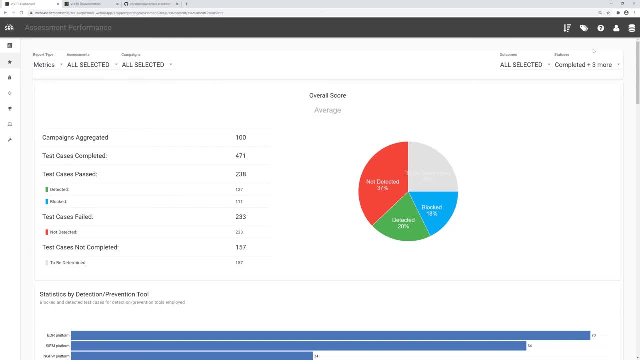 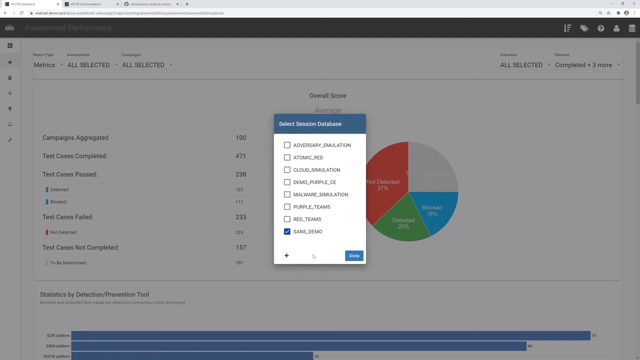 One more just conceptual thing to notice. We also have a number of different databases that we're going to jump into. So at the highest level of the hierarchy, everything in vector is organized in a database. So you can think of this as really the top level org unit. 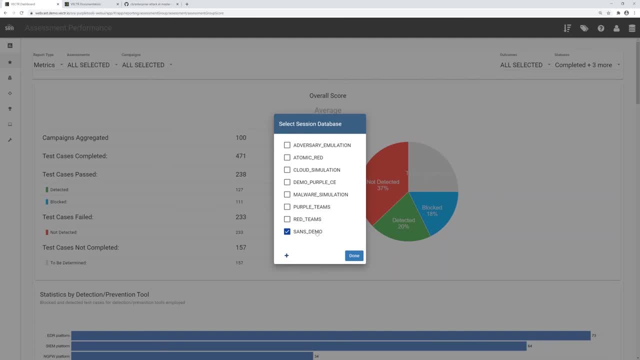 Some vector users out there have different databases for different team functions, So maybe red team threat Intel teams want to keep their assessments separate from a reporting standpoint. Some organizations just have a single database, that that is meant to house all of your assessments for more, more unified reporting. 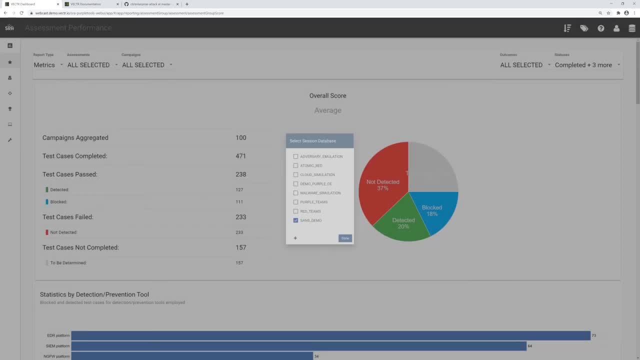 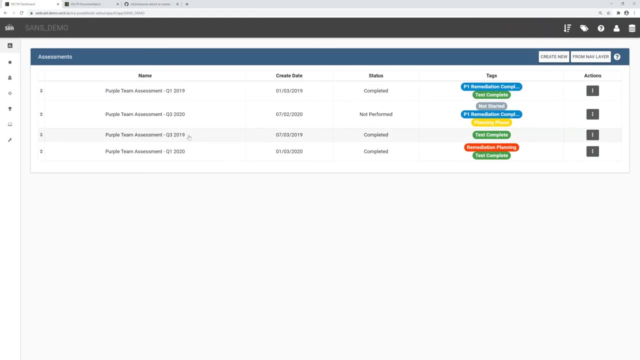 So we're in the SANS demo now. What you're looking at here: the assessment dashboard. you see these major assessment activities that we have going back to Q1 in 2019.. So everything in vector is. you know, you can generally just click around by by hitting a row and jumping right into that view. 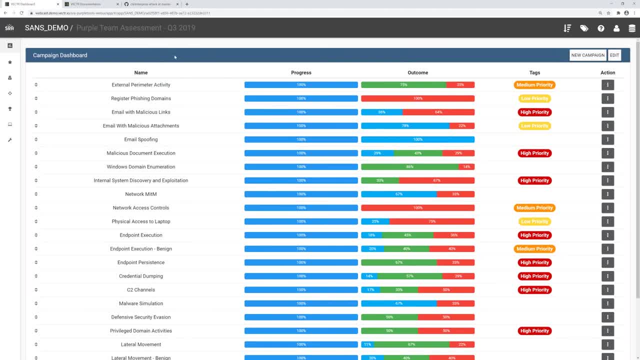 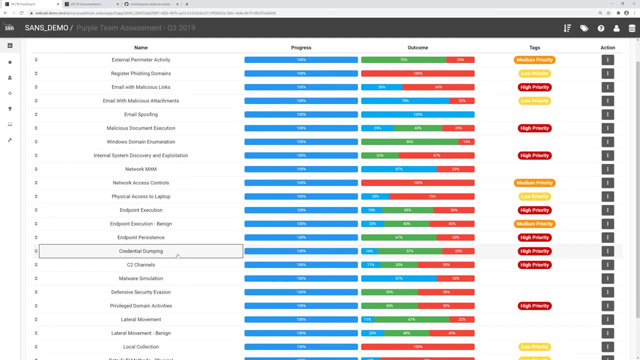 What you see here is is a sample purple team assessment. underneath of that You see a number of logically grouped campaigns. So these names are are pretty intuitive. but if you're looking to do very controlled testing of something like credential dumping, you know we've created a campaign for that, which takes you into the campaign dashboard. 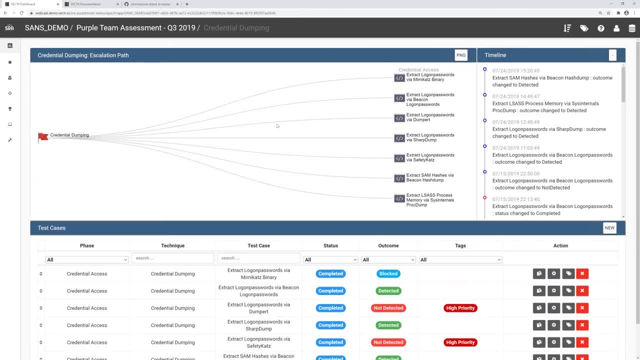 Here you see a nice, nice visual heat map, So this visual can be more useful. Yeah, So we, we, we. we have a two page view here And you can see that the demo test case is very successful when you're doing more typical red team style escalation path attacks. 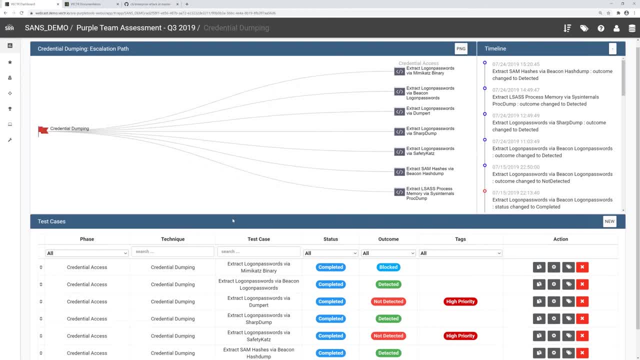 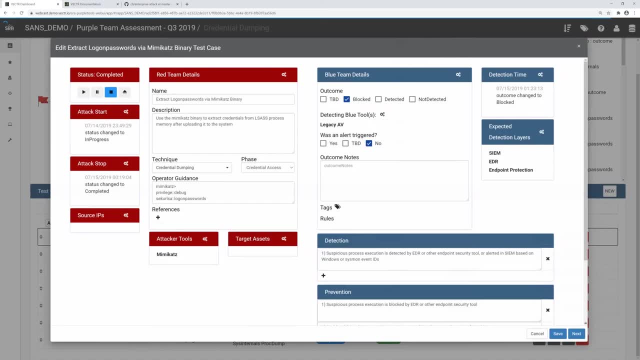 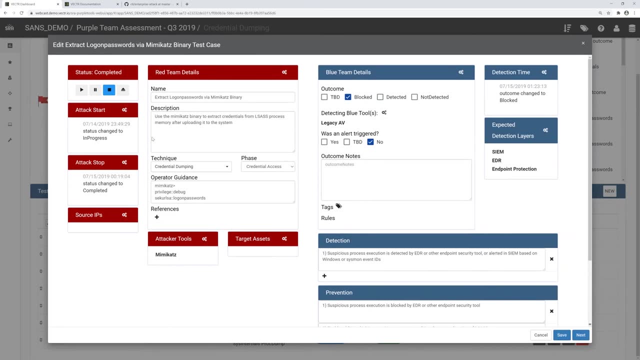 In this case we're really strictly just testing down the credential access tactic. So underneath of that, this is where you can load up the individual test cases. So those are easy to launch. You can just click on the row. This will bring up the detailed test case panel. 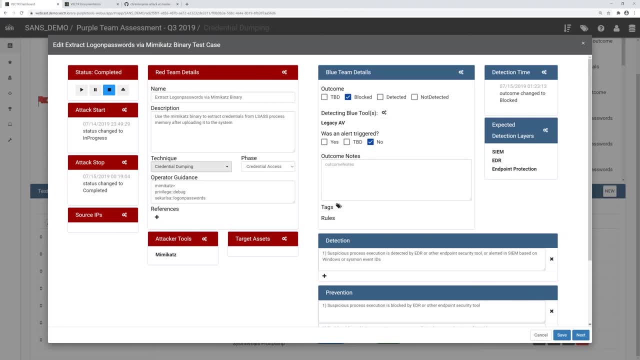 the left side is really meant to describe more of the red team TTPs. so attack. when did the red team actually start? stop and attack? what are the time stamps? what actual attacker source are they coming from? this could also be something like your external command and control infrastructure. if it's more of 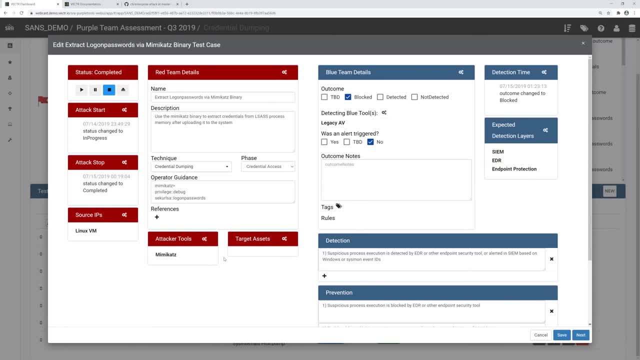 an external attack. what tools are we using so a very familiar one that you all know. I'm sure Mimi cats the target assets that we're actually going after. maybe it's a loaner laptop that you're looking to just beat up as much as possible during a purple team assessment. it might also be just a live target. 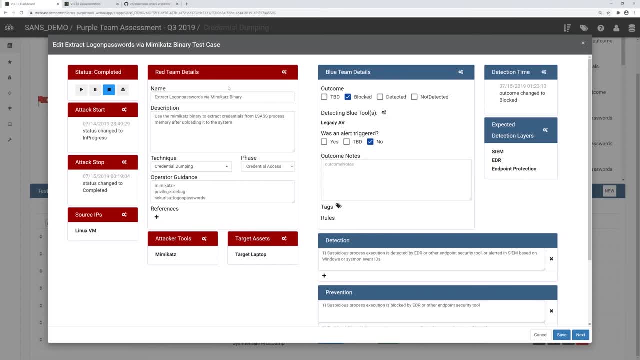 somewhere in your environment. that's what you see here, really the, the core of the test case. this is really the, you know an atomic, that the smallest unit of testing in vector, a description. so this is the unique test case procedure, the test case variation that you're looking to demonstrate, the actual technique in. 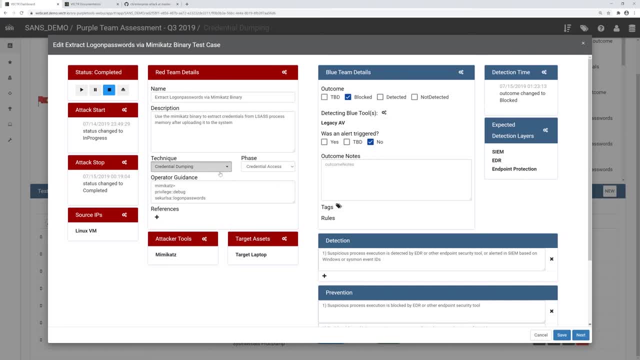 this case credential dumping. this is something where we actually have an autocomplete for MITRE techniques. you know so across the industry and in our own usage we're not calling credential dumping. you know five different things, so a nice little autocomplete there. and the phaser tactic, another important. 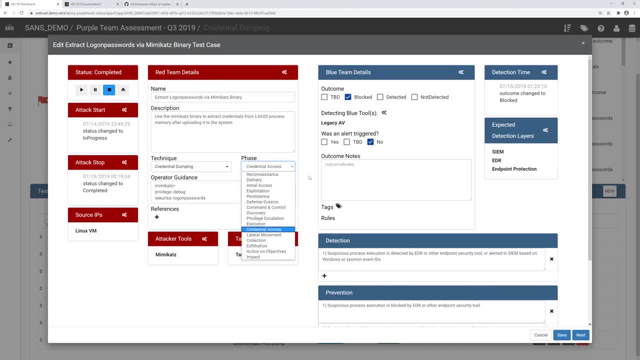 concept in vector. by default we use more of a unified kill chain view. I would say a minimal unified kill chain. so if you're interested in using, you know, more traditional Lockheed style kill chain or a Mandiant attack lifecycle phase or just MITRE tactics, you have the ability to actually create custom kill chains. 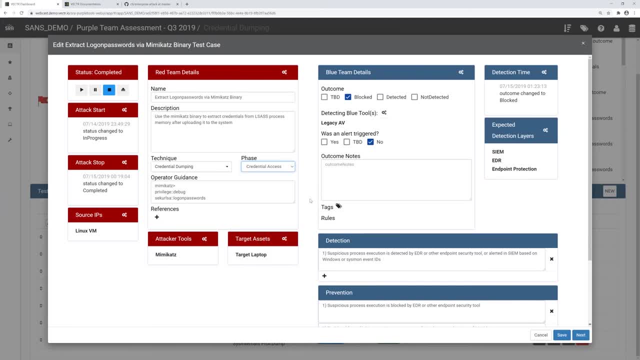 and make those the defaults across your assessments down here. operator guidance. so in this case it might be a use cobalt strike to run this pre-built command that you can launch. in some cases the operator guidance might be very specific command line arguments that you can run and really codify for reuse across your environment. 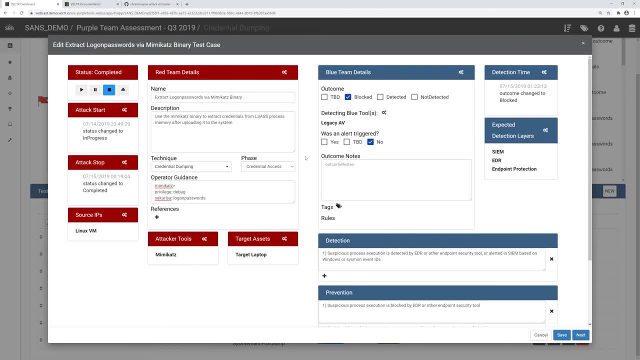 for more continuous controls, retesting efforts over on the blue team panel. you see the basic outcomes. so in this case we've, we've just done something not so stealthy like drop, drop many cats to disk. you can see, we've noted this. this activity is blocked. actually our legacy. 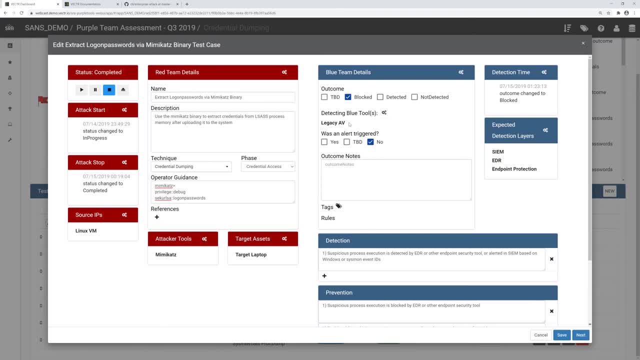 AV product was able to detect this versus the more advanced EDR suite. but you can toggle. everything will start in the TBD status. if something is blocked there. we have some sub outcomes available. so in some cases you know if it's your mail gateway you probably don't want an alert every time you know a bad email is. 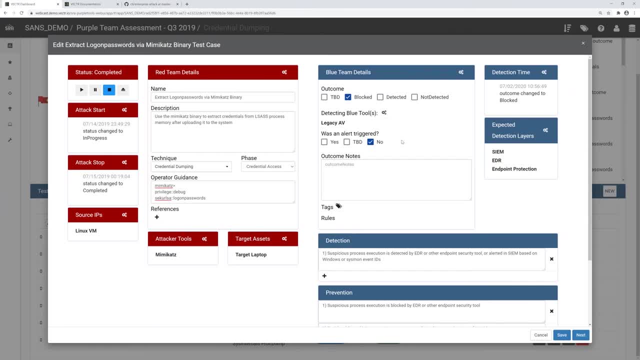 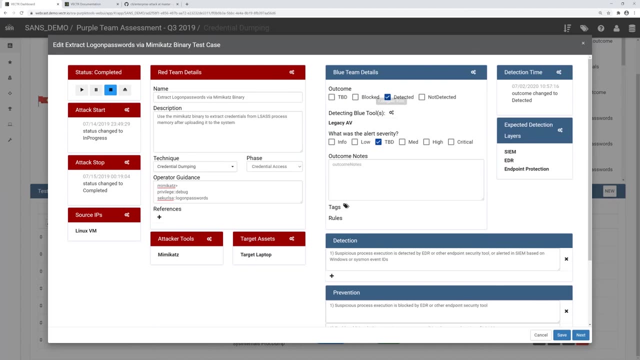 blocked, that would be, you know, millions of alerts. however, you know, in some cases, if something is blocked, if you received an alert that can be very valuable, Intel to to the sock to start an investigation of what was blocked, similar to detection. we have, you know, basically a basic severity level all the way from 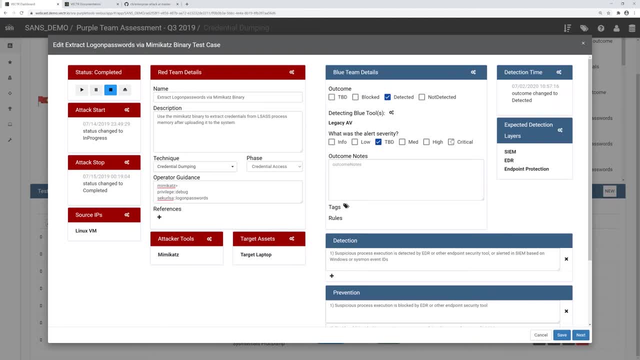 informational up the critical. so one thing that we often find in purple teaming is: you know, oftentimes you know technically a lot of activities might get detected, set off some alert, but only if you know the security admin- this is admin- is actually staring in the sim console. so this is meant to be. 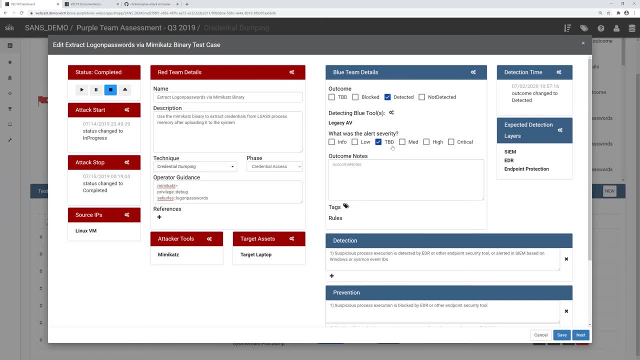 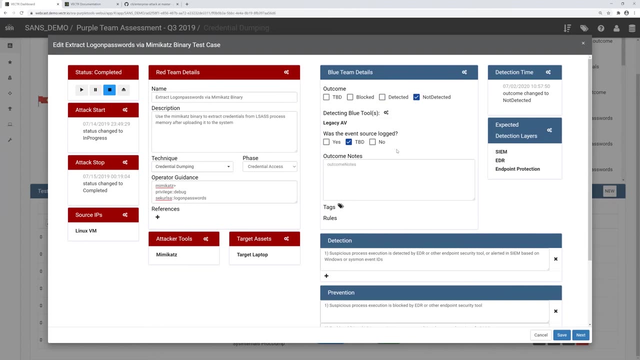 really an honest rating of okay, this clearly should be a high risk, but but was it really more of a low or medium that nobody would have kicked off any kind of incident response playbook for? and was something not detected a useful sub outcome? if it wasn't detected, then hey, do we have, do we have endpoint? 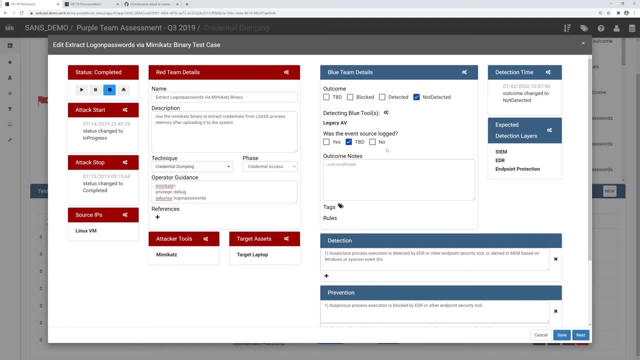 visibility, telemetry logs, for whatever that was. so this can be a very useful sub outcome to further drill down into, especially when it comes to tackling or mediation. for hey, what's the best way to do this, what's the best way to do this? for, hey, we can quickly, we can get some quick wins in our EDR, in our sim, because 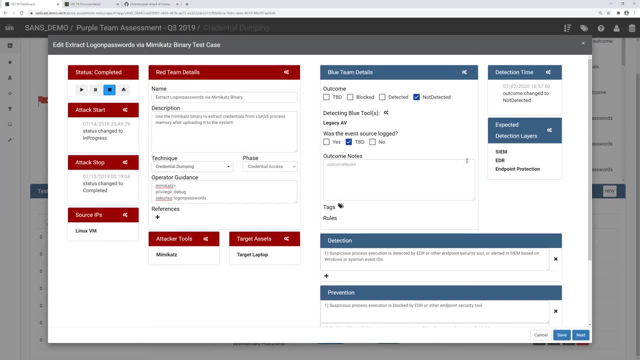 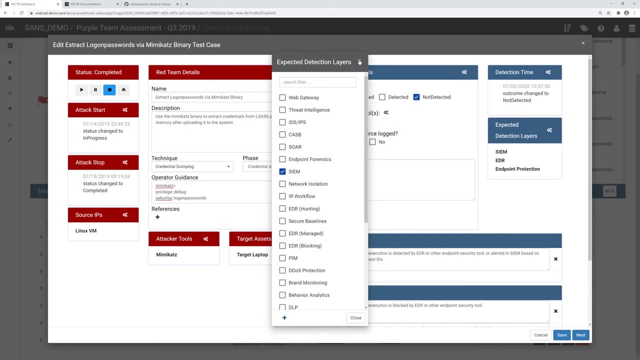 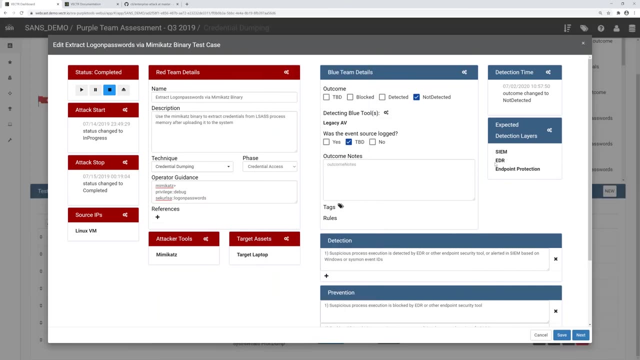 we actually have the logs. we just need to configure some alerts and do some testing over here. just a couple more things on the test case panel. this is really what we expect to be the, the core defense for whatever the the test case might be. it might be a single hey, we really think EDR is the only thing. 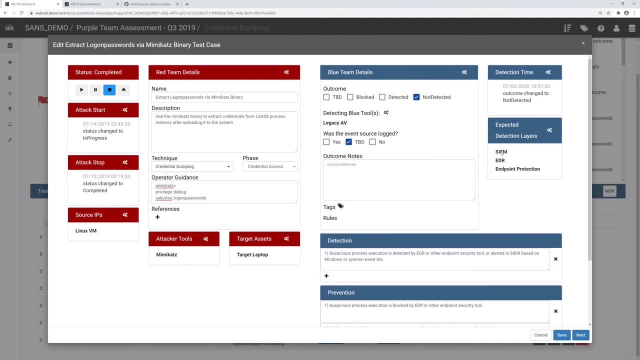 that's going to catch this. there might be a couple tools that that play together. so if you're ingesting your EDR events to your sim, you might expect your sim to set off the right alarm. that would actually kick off the right process with security operations. so all 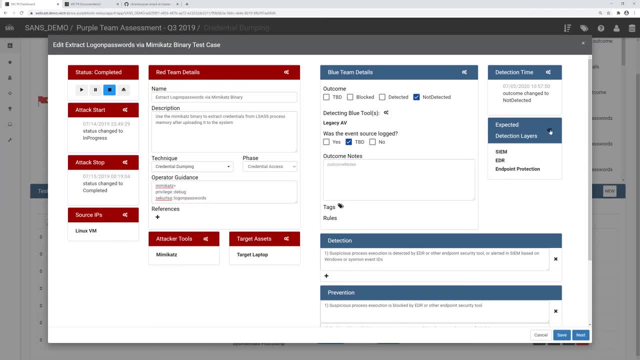 of this, a lot of what you see. all these, these toggles, these are fully customizable. so if you don't like the detection layers- defensive layers- that are in vector, you can fully customize those to two more suitable ones to your liking. and just down here we have some additional detection prevention guidance. 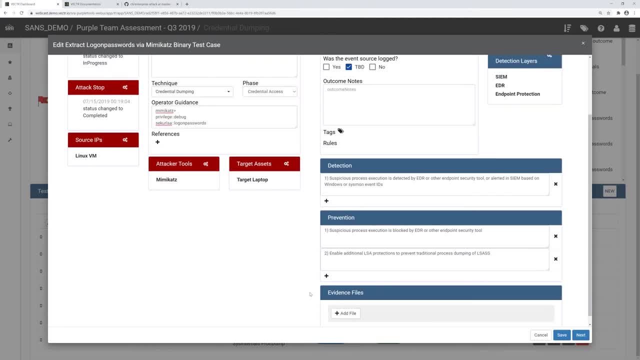 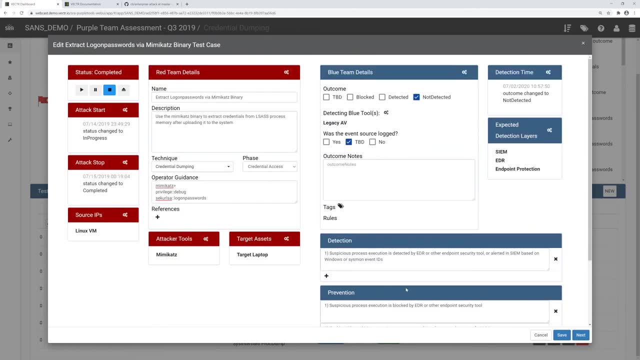 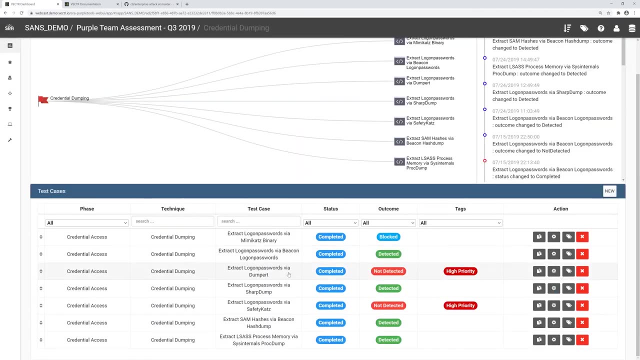 for the test case procedure and also the ability to upload local evidence files if you wanted to provide more formal tracking of alerts and emails and things of that nature related to the test. so that is a test case panel in a nutshell. something else in vector that's that's very useful is the tagging system. so 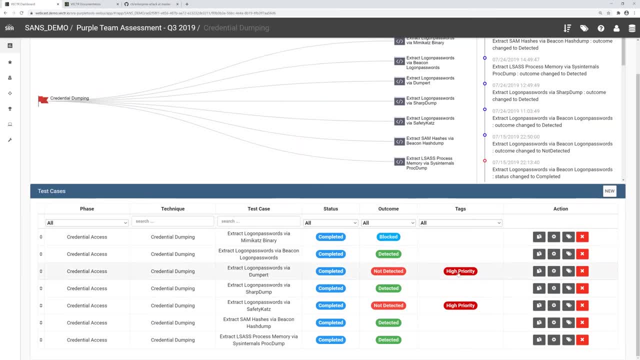 this is something that you also have a lot of control over. tags can be applied at a test case level, so this is something that you can use and come up with your own criteria. maybe it's remediation scales, it could be, threat actor groups it could be. 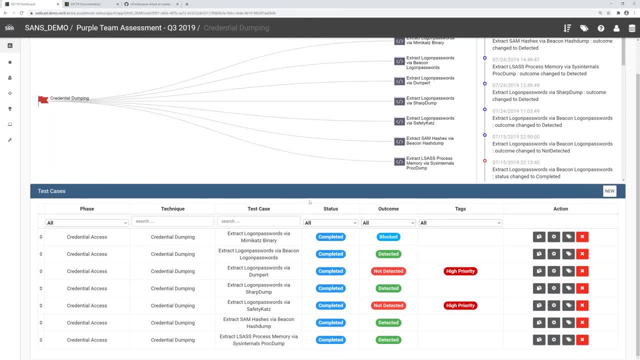 internal teams that are actually maybe responsible for investigating something. so some other features here: you're not going to get into too much detail here, but say you have a test case procedure and and you know, by the nature of adversary emulation and this type of testing, you have the ability to. 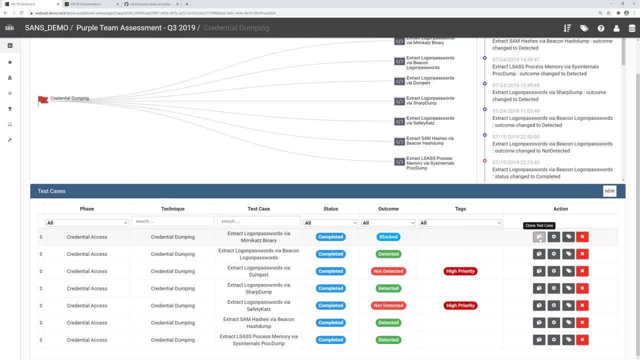 basically clone test cases on the fly and create different variations and save them off, but inherit- you know- most of the base properties of that test, so that makes it easier for teams just to you know innovate on the fly, do additional defensive evasion and try something new and record it. 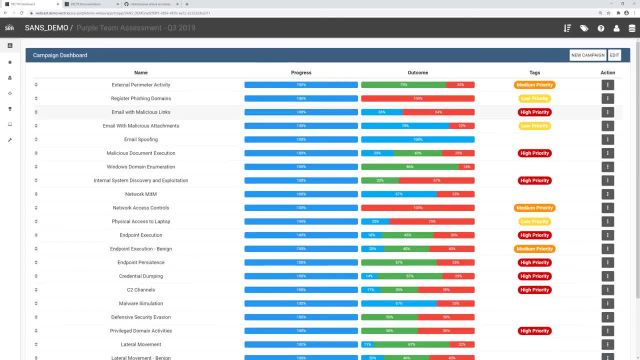 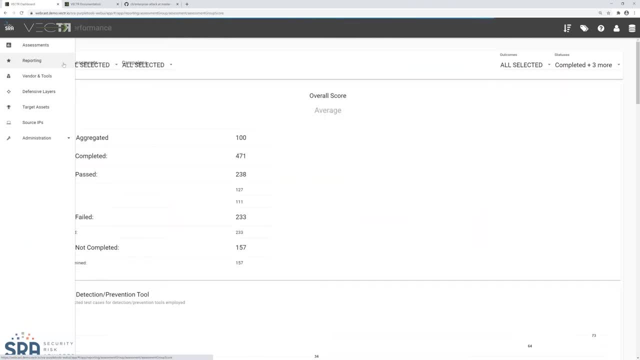 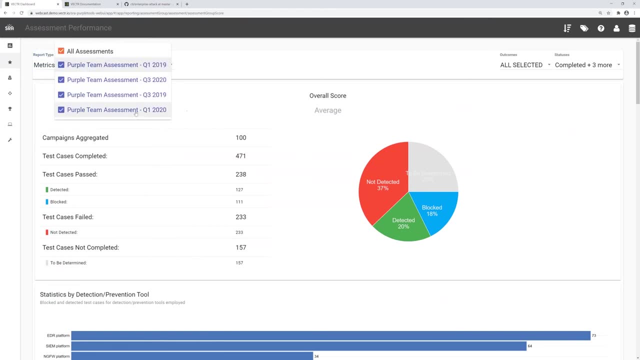 so move on here. so this is the. you have the campaign dashboard in a nutshell. jump back into our reporting view, since it's really more of a unified view and that you can jump around into the different different major report types. you can see we actually have an assessment here. 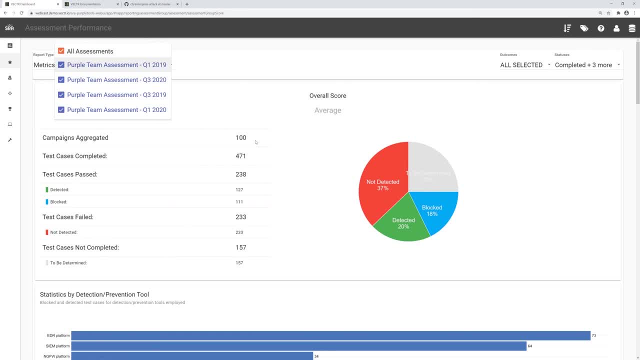 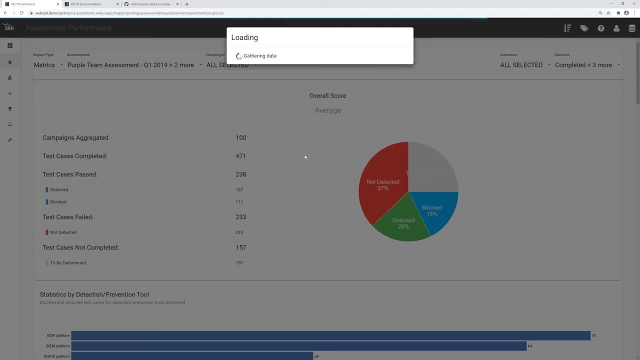 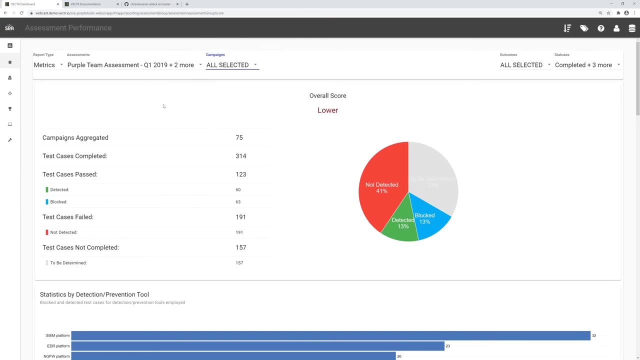 that is queued up and ready to go. we have. we haven't actually run through that test, so everything is still in a TBD status, but part of this unified reporting dashboard gives you the ability to drill down into very specific assessments or even at a specific campaign level, and just see that data. 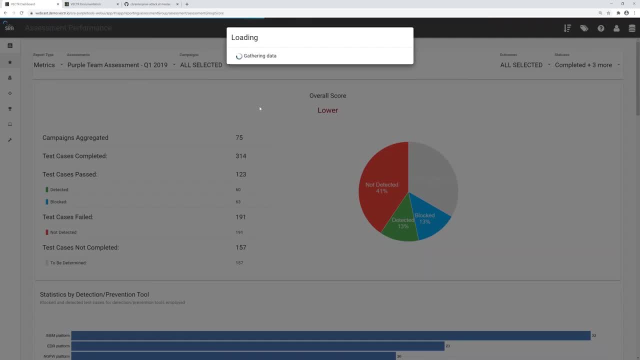 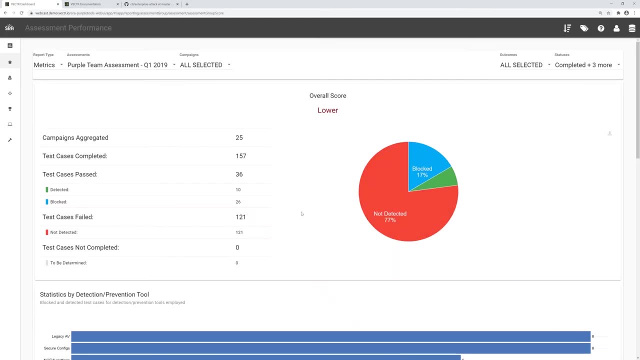 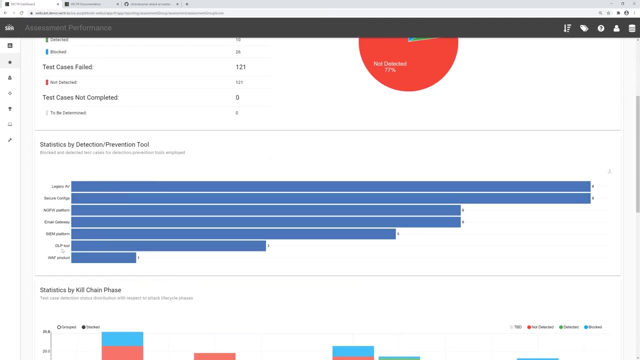 and if I just wanted to see a single result test, I can drill down into just q1 2019. see what that snapshot look like. further down, some high-level stats: these, these actual, these would be your actual tool names that you've configured in vector for your environment. these have been I've 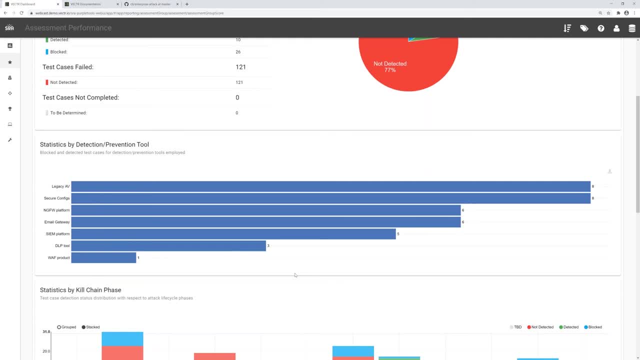 just made generic names for them, but you know your comment, your sim, your EDR, your firewall platform, DLP- if you have one, maybe other other controls that might come into play on the perimeter, like WAF products, your secure email gateway, and so these are common platforms. you would expect to get pretty good coverage on. 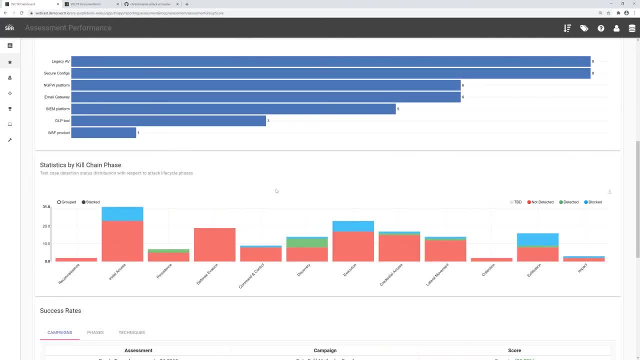 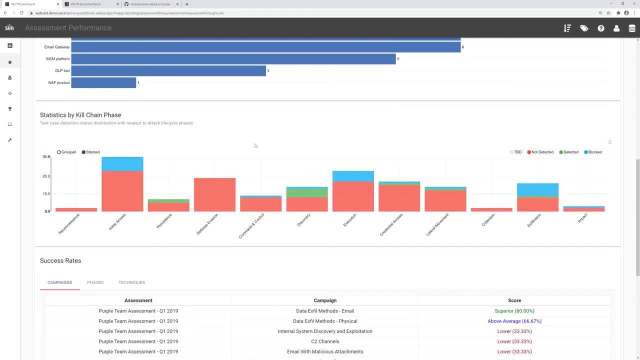 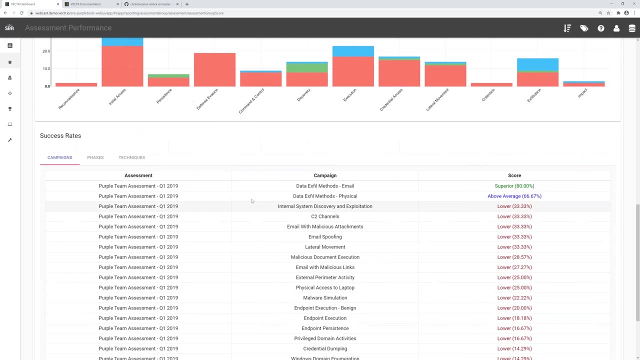 especially if you're doing more, more testing a line to attack. we have other views here, more drill down views, but just at a high level. you know how are you looking across major phases or tactics and improving over time and further down here, just at more of a campaign level or specific phases, what? 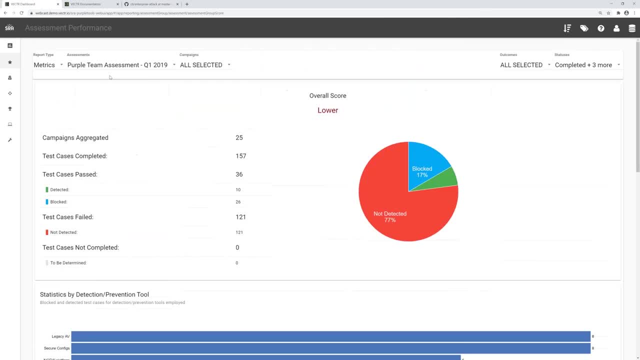 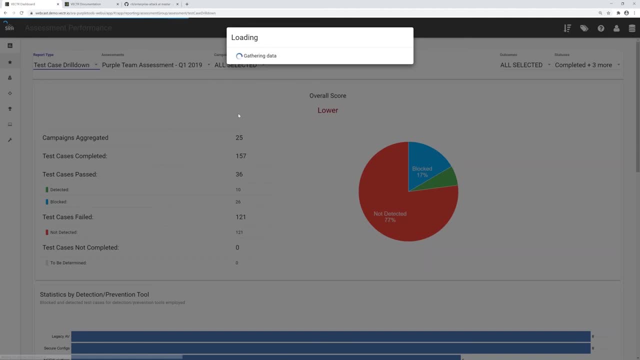 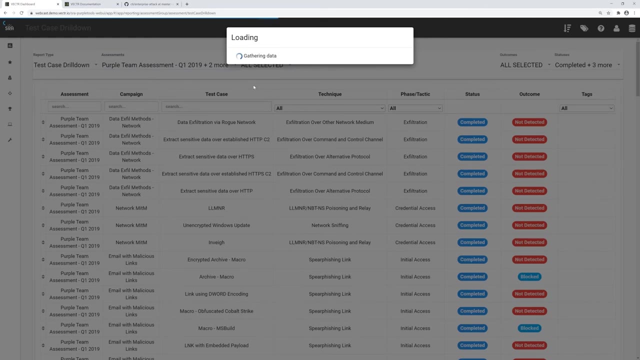 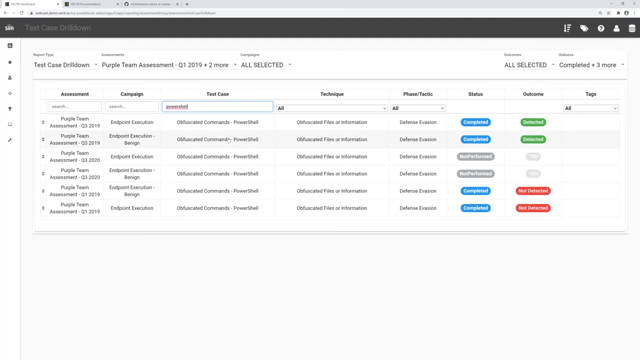 is the relative maturity. looking like some other views that are really useful, this test case drill down view, so this can be really aggregated like like the other major reporting views available. this is more of a power user view where you can search for anything of interest. so we wanted to look for: hey, what have we done around PowerShell in this? this? 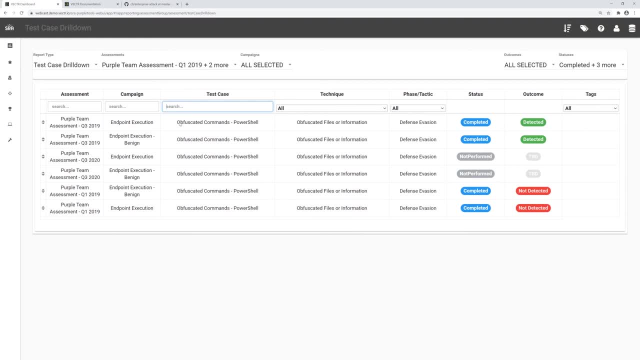 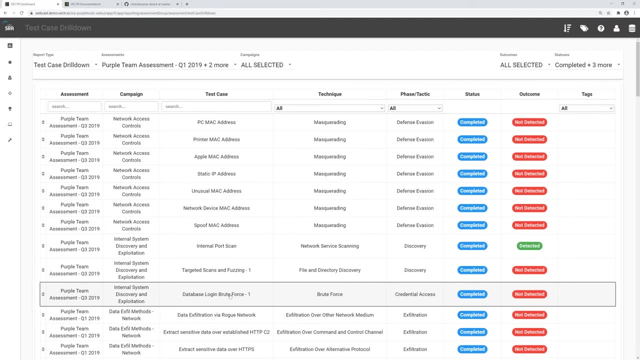 assessment scope. you can do some quick searches here. you can also fully open up any of the test case panels from here as well by clicking, so that's just a quick way to do searches across larger data sets. show you the heat map view. so this is a our version of a mitre's attack heat map. 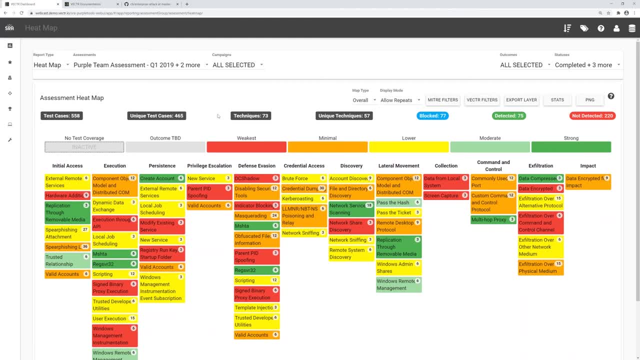 really the the goal of this. you see, we have, you know, the current version of attack, but we also have, if you see, the numbers here. we also have the ability to drill down into these specific test case procedures that we're using here. so you we've run through. so if I click on credential dumping, you can browse. 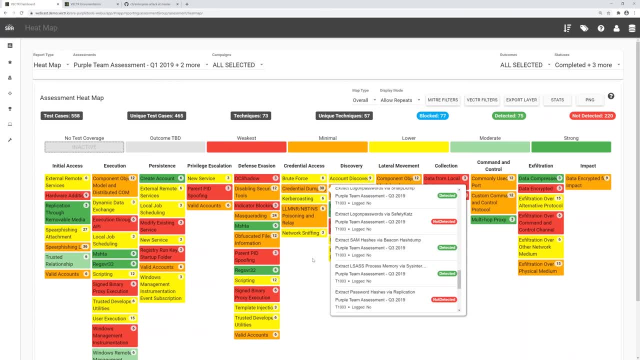 really everything you've done that's been mapped to that technique. so we think this is a pretty powerful to be able to bring in any mix of assessment data that's been mapped to ATT&CK and be able to show, provide a quick answer of what relative coverage you might have. 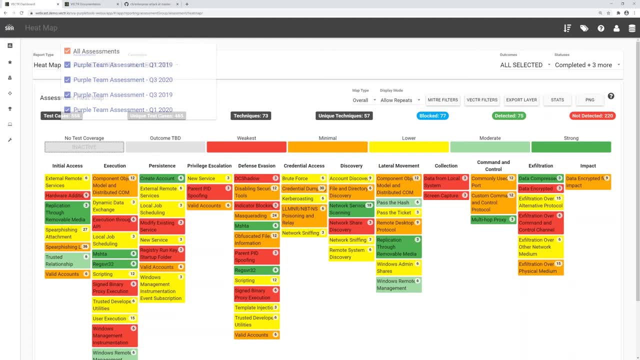 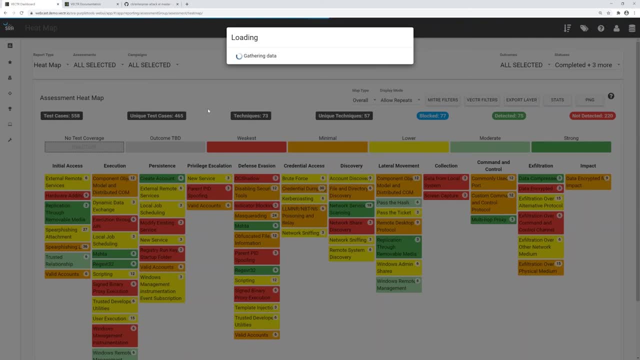 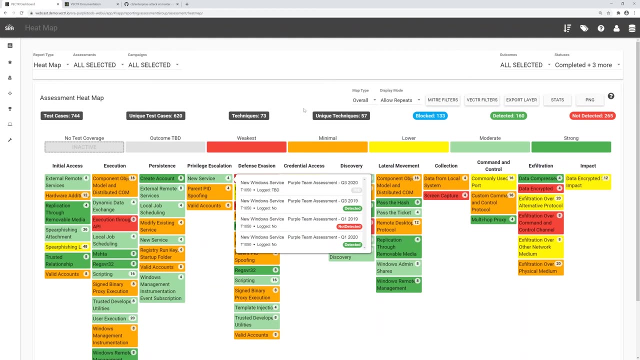 and this will be more aggregate too. so if I introduce the assessment that I haven't actually done yet, you can see we'll have a number of more test cases that are still in TBD status. so there's a couple of useful filters here. we have a way to basically deduplicate some, some more repeat activities that you might. 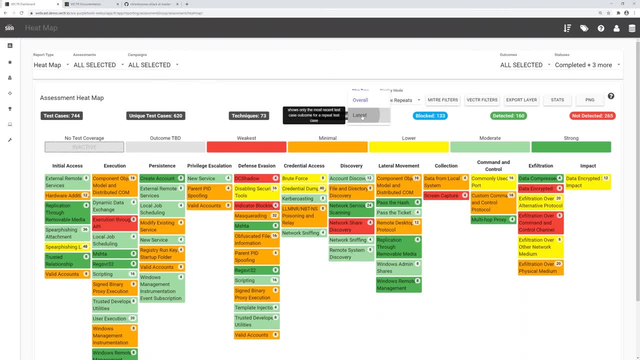 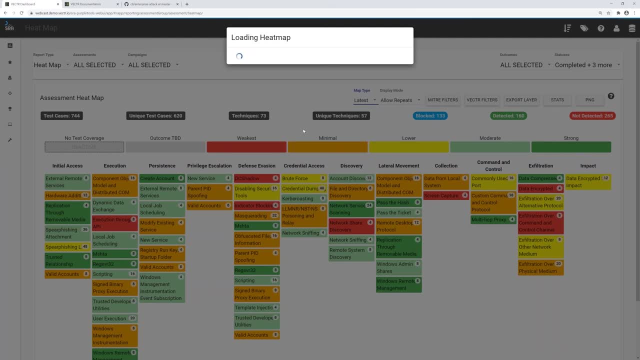 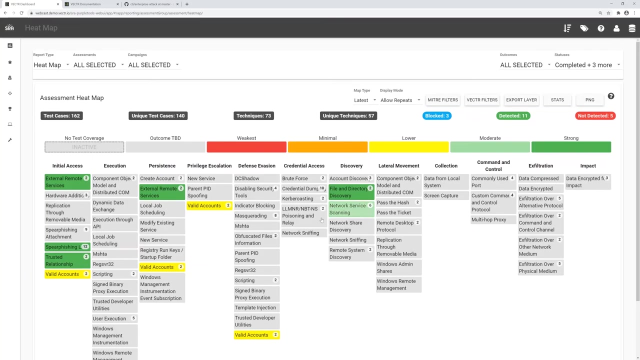 have. so if I switch this map type to latest, give it a second to load here. so you can see we've deduplicated a lot of our tests and we're only showing the most recent status for different test cases that we've run so up here we also. 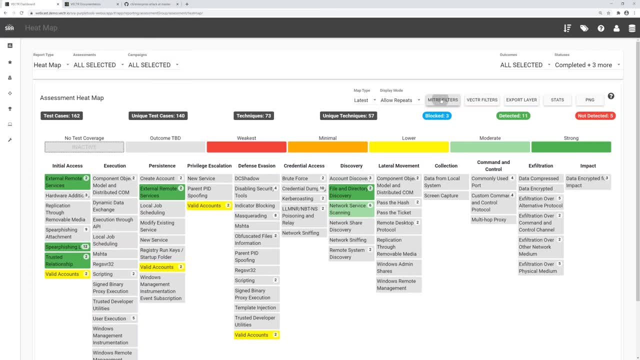 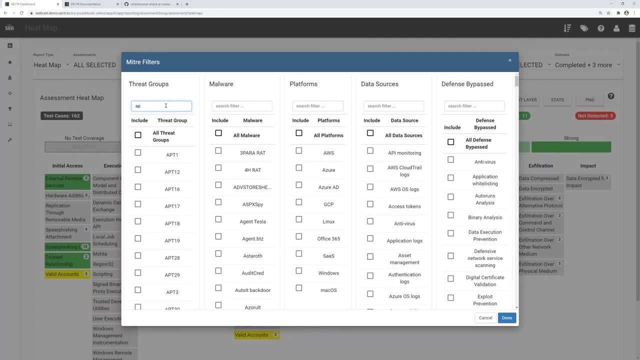 have a number of other filters that you can leverage. so these are the MITRE filters where, if you need to produce a top-down view of, hey, how is our, what are our defenses? current defense is looking like against something like APT 41, I can select that search for that threat group. apply the filter. you see we've applied a. 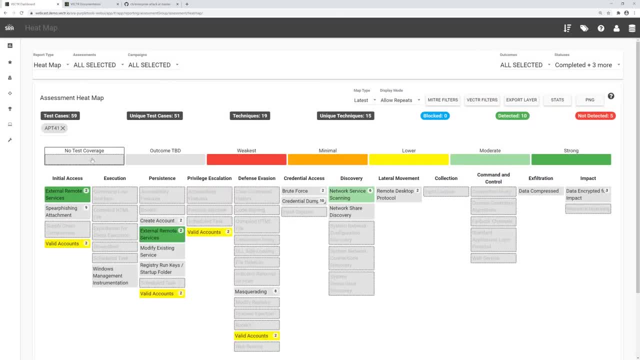 tag here for active filters. this is important concept too. you can actually click on these to filter out different different statuses. so there's no test case coverage means it's a perfectly valid technique that is attributed to APT 41, but we don't have any current test coverage in the system. if you don't, 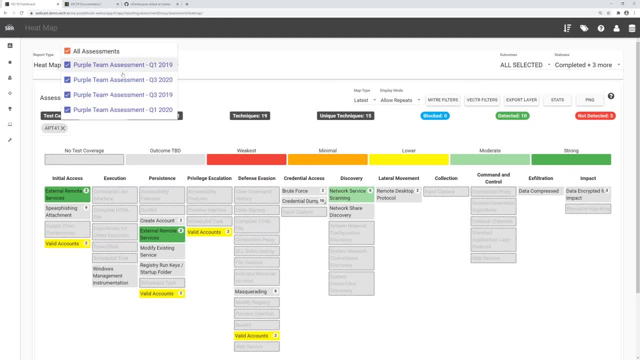 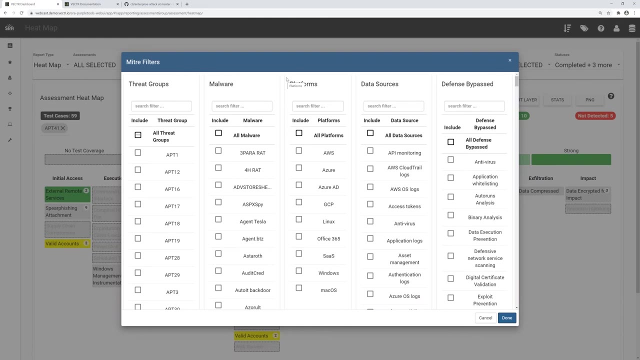 mind. let me give a quick example. if you go back to selecting the different APTs, many of you might have recall in January- feel so long ago- of 2020- um, we started the year off with the assassination of Soleimani, who is an Iranian military, and the first question we got, like January 2nd or 3rd, was: who? 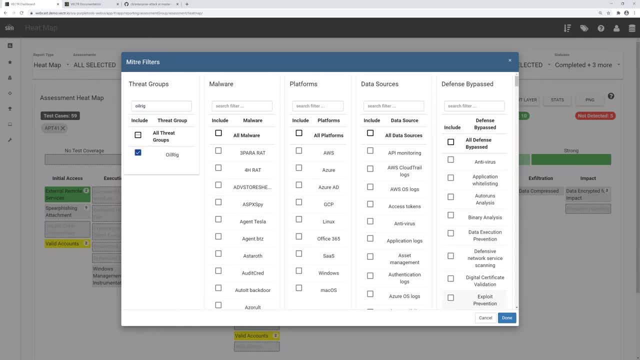 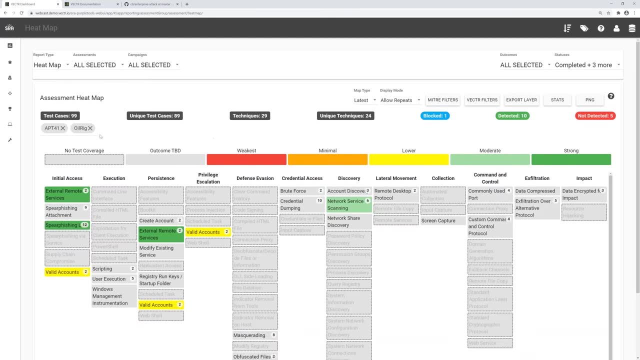 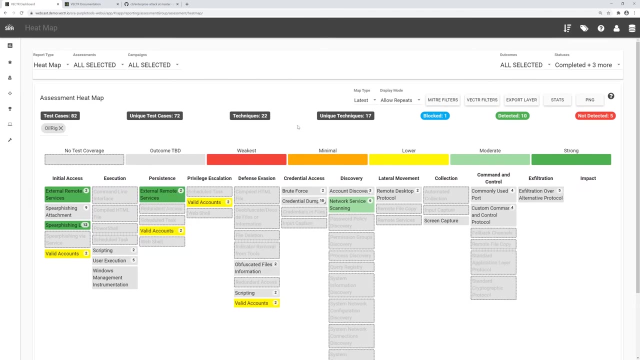 are these Iranian threat actors and what can they do? and we were able to answer this question for a lot of senior level personnel in our organization with vector that, going back to our previous year, was like: oh no, I think you know we can't do it because we're not doing this exact filtering, so we didn't actually have to. 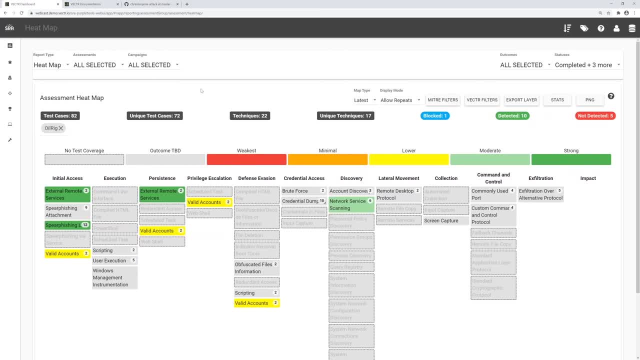 go emulate anything new. we actually had tested a lot of those and we're able to give a quick snapshot of where we had gaps, where we didn't have gaps and allowed our senior management to make a more informed decision as to what the immediate action should be, given this new heightened threat actor and possibility of attack. so just want to give that quick example there. OK, 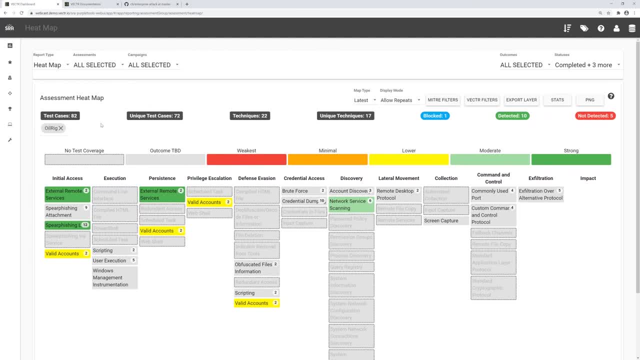 Phil, sorry to interrupt. Thanks, George. Yeah, while you were saying that, I actually applied oil rig, which is one of the more prominent actors part of that group. So that would give you the answer of you know, based on what you've done, what relative coverage do you have? 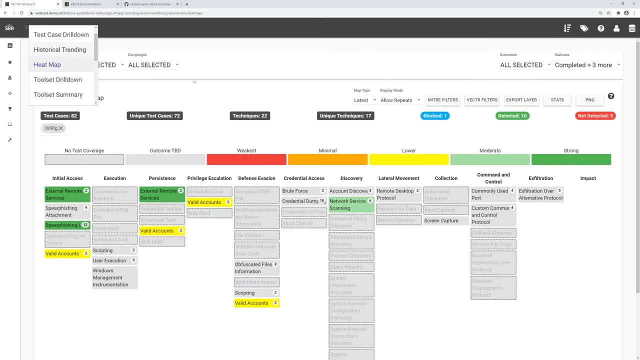 Yep, and what coverage do you need to test as well? Because, as you see on this screen, there's actually a lot that might not have been tested, So you might want to prioritize those tests, given that a particular threat actor now has the intent to attack your organization. 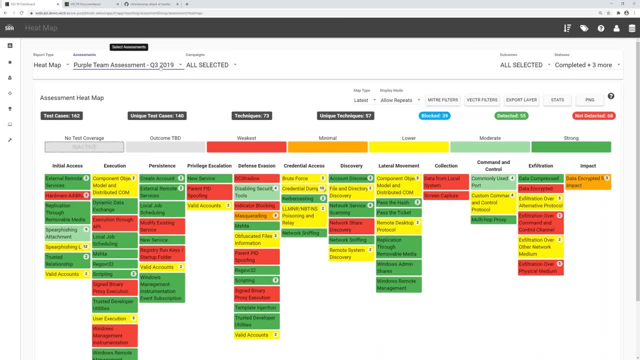 Great. So just to close out the heat map discussion here, I've just zoomed in on the latest major assessment that was completed, Like I said, with the inactive if you don't want to show all of the tech, hopefully you're not trying to conquer the entire framework. 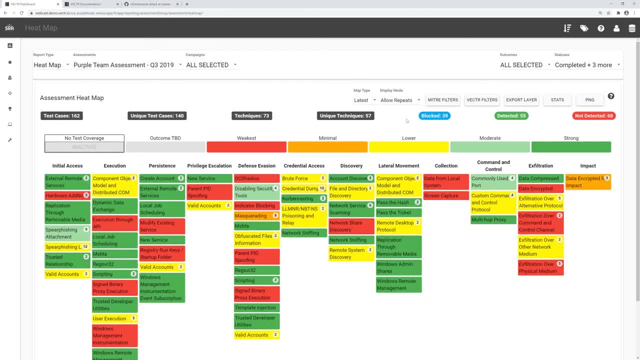 overnight, but just focusing on the work that you have done, This would just be a great way to show that you're not trying to attack your organization. So that would just be a great way to show you a snapshot in time, And you're also able to export. 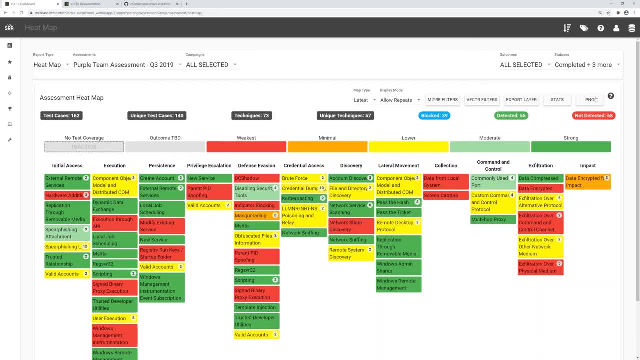 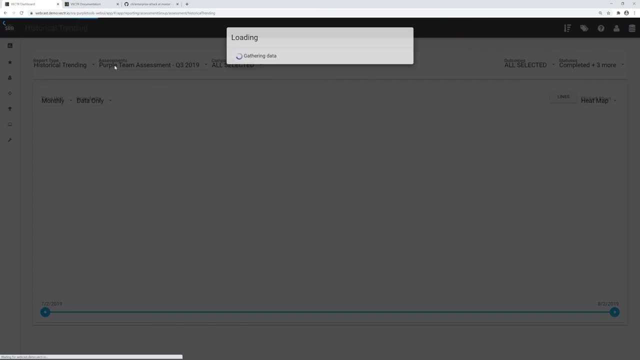 the images as a PNG, which can be useful for dropping and presentations and other uses like that. So that is the heat map. We have a lot of useful filters in here. I want to show you the historical trending view. Let me pick some actual data to trend. 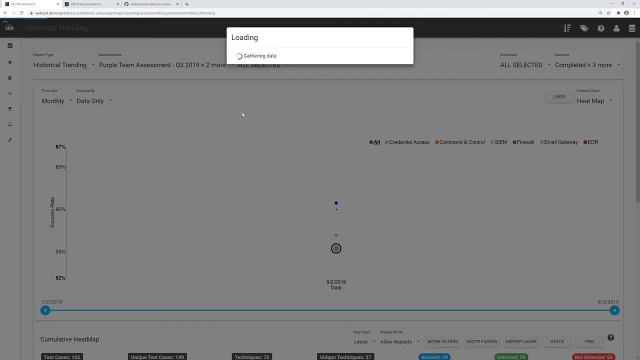 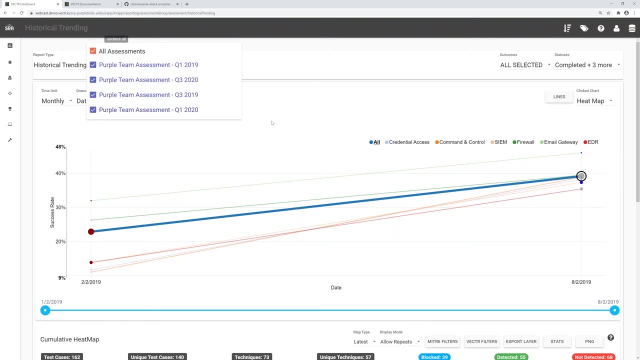 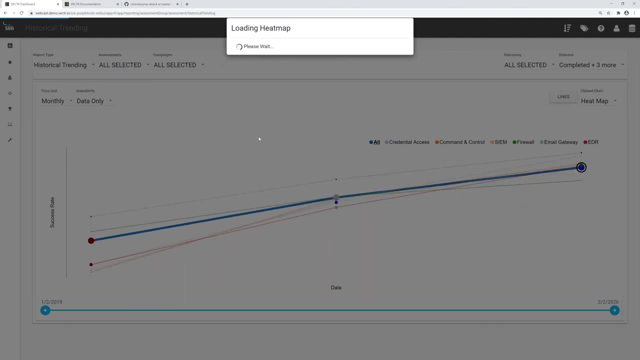 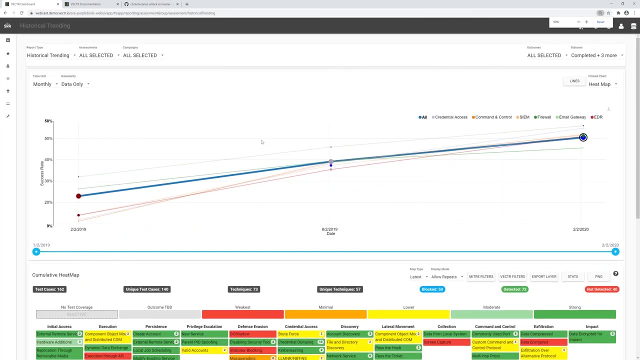 Okay, yeah, and this is the part where you can show. this is um. i put this on linkedin if anyone saw that post. um, about two years ago, my cso at city came and said: i i get this. i get all the value these red team engagements are doing are having on our organization, but i need a better way to show. 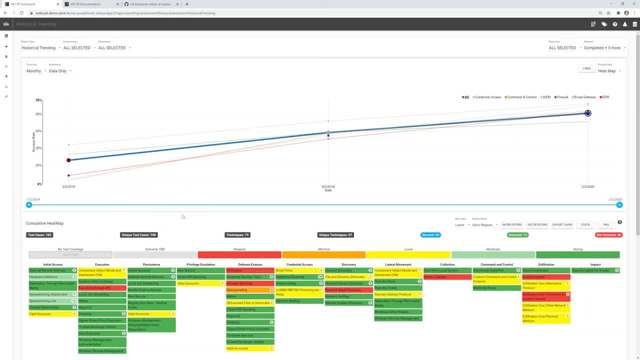 that we're actually improving that by doing more red team engagements and then the soon, uh, purple team engagements that we started doing about two years ago as well. how are we improving? and, uh, if it wasn't for phil and his team and vector, this would have been a lot harder to answer. it's. 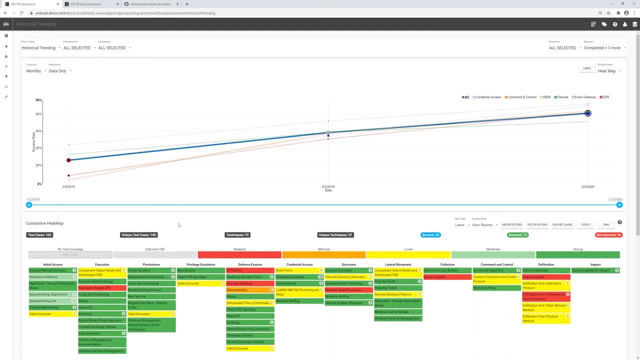 because of this historical, uh trending, he's about to show great, yeah. so what you see here, i zoomed out a little bit just to capture the sub charts, uh. so in this case we have, you know, on the y-axis, major data points over time. uh. so these rep, these basically map to the major assessment activities. 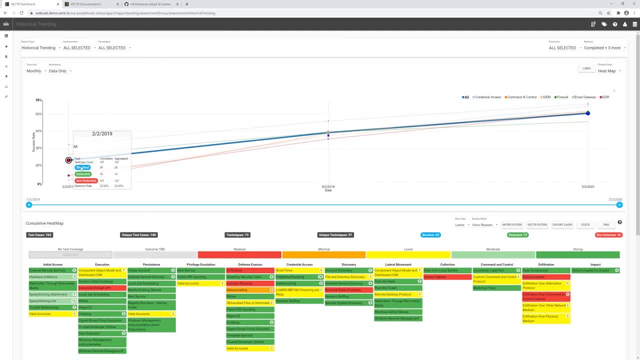 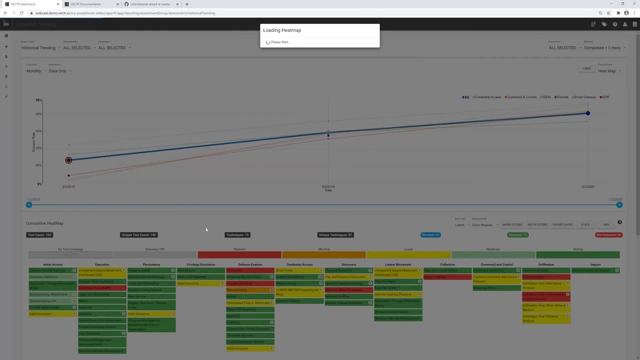 that you saw. uh, you can click on them to see a snapshot in time of: hey, what did? what did our attack coverage look like in early 2019? give this a second to load, okay, so not good is the answer, um, and as you click on the red team engagement, you can see that the red team engagement is. 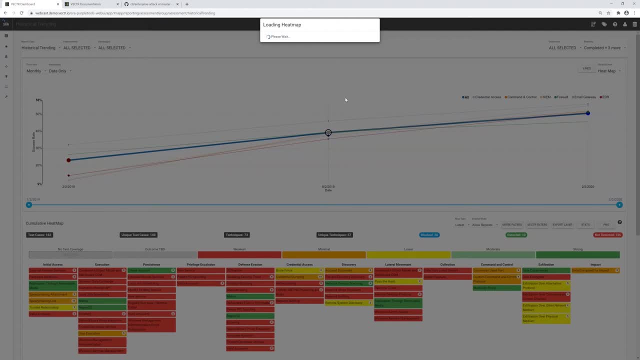 pretty much the same as the red team engagement. you can click say we'll fast forward to two, three of 2019. you can see significant enhancements were made um coverage and fast forward to early 2020 um the coverage of you know, for the exact techniques that were tested has. 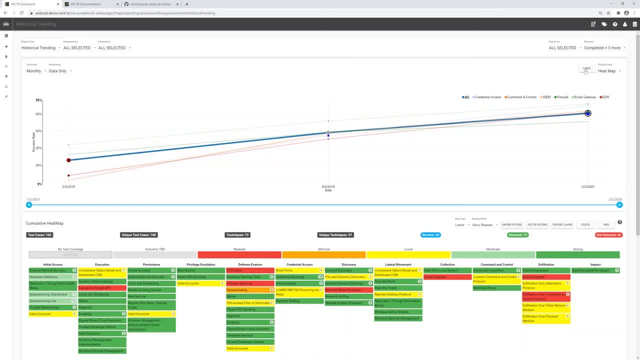 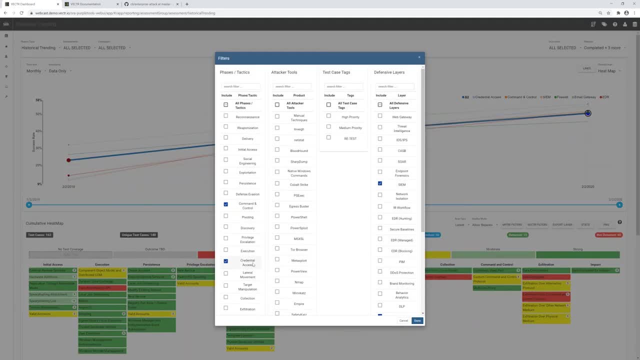 gotten much better over time. uh, so some of these other other filters that you see too up in this lines box you can apply uh different tactics that you also want to trend so is, you know, credential over time? uh, these can be any phase or tactic that you're using. uh, some other filters, like at a 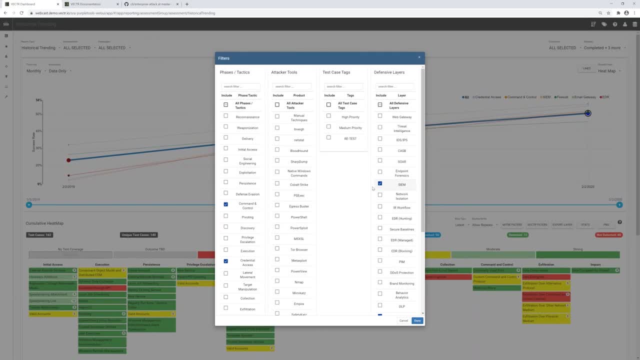 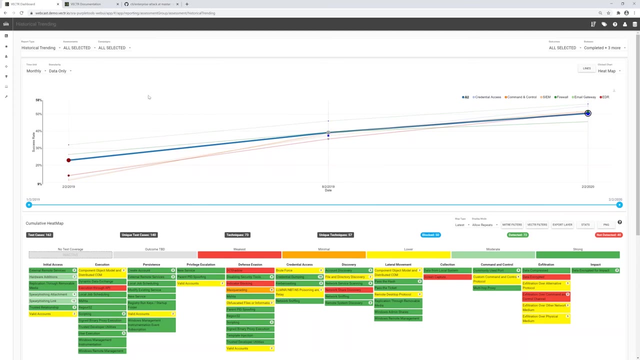 defensive layer. so how is our sim actually getting better over the past few years, based on the engineering work that we're doing? uh, or maybe some new tool acquisitions? uh, so you see, some of those filters have been applied here for a couple of those categories. zoom back in a little bit. 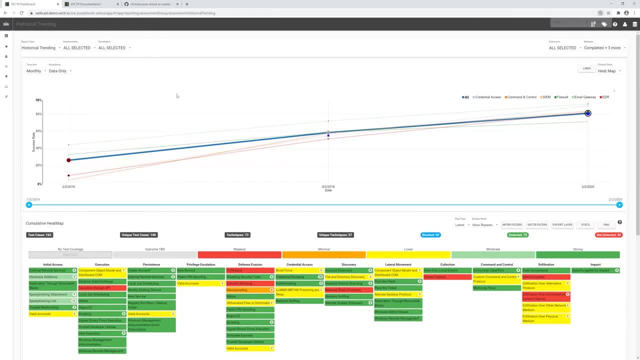 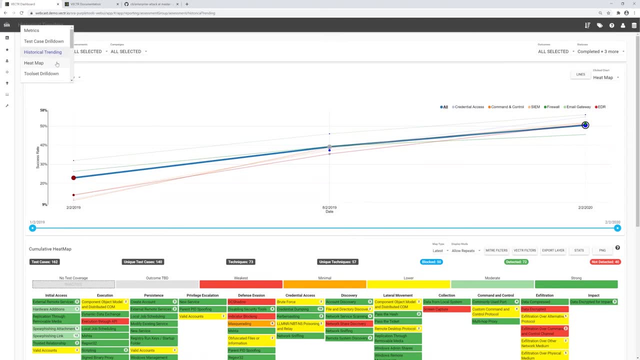 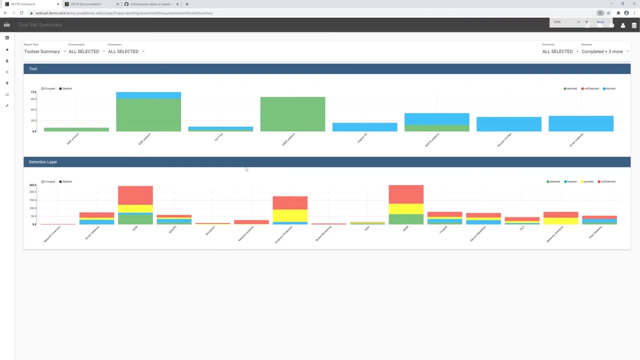 um, so this is a obviously a feature that gets more useful. we have a couple couple larger data sets where you could actually start to show some of the trending. uh, in the mix, show one or two more reporting views here. some others are a little bit more geared towards. 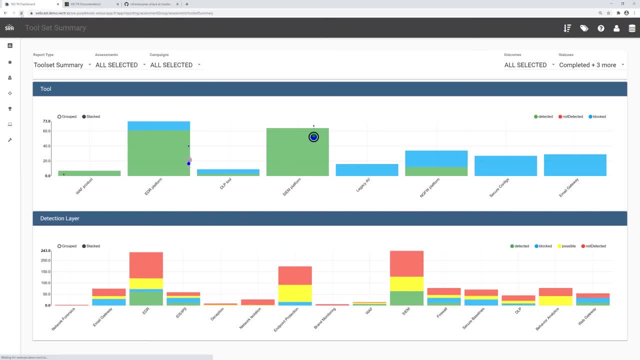 actual tool improvements and detection layers themselves. so you can see at the top says specific tools like EDR and sim. uh, down below the the categories that those are mapped to, you know you might have multiple sim platforms. you might have multiple endpoint protection platforms. you also have a 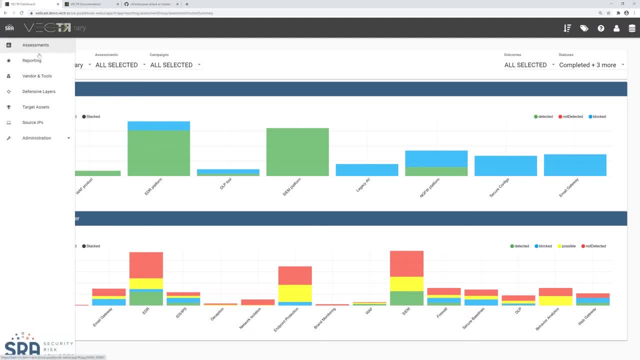 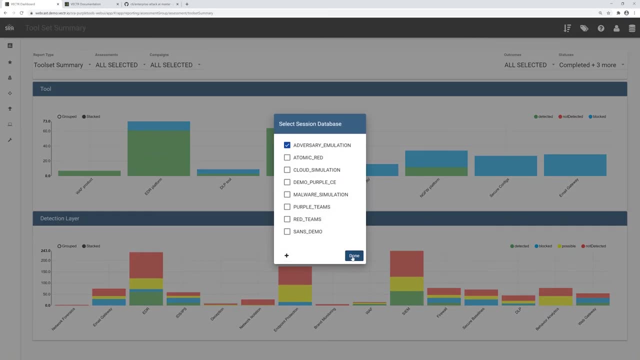 way to kind of see that at a higher level. so reporting views. I know we don't have a time to show everything here. I wanted to jump to another database, though, and show you some some of the adversary emulation capabilities in vector. showing you was more geared towards more typical purple team activities. 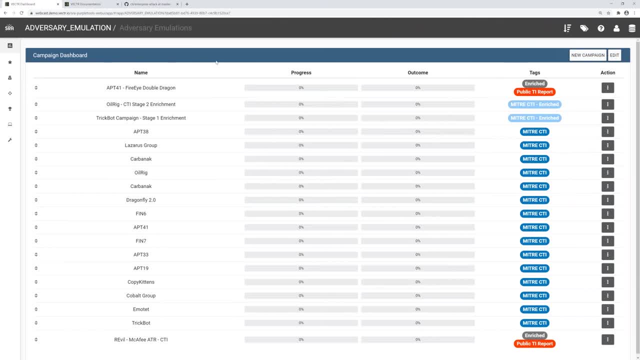 uh, going to this adversary emulation demo database, you can see we've actually brought in a number of campaigns directly from CTI sources. we have, you know, also leveraging the tagging system here to show: okay, we pulled oil rig directly from miter CTI. there's some others that we've actually 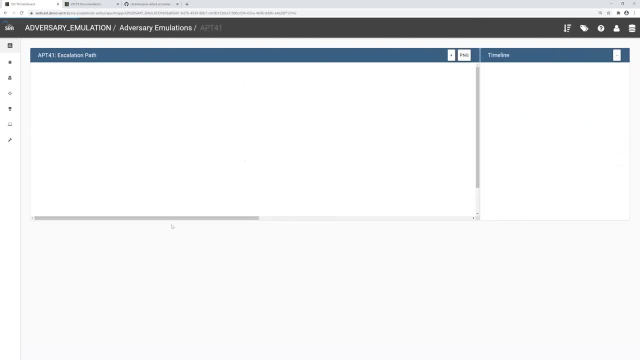 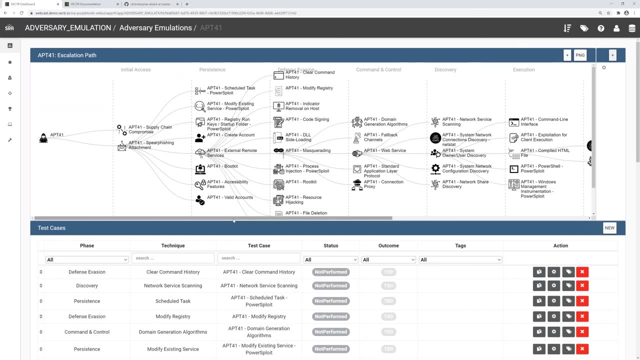 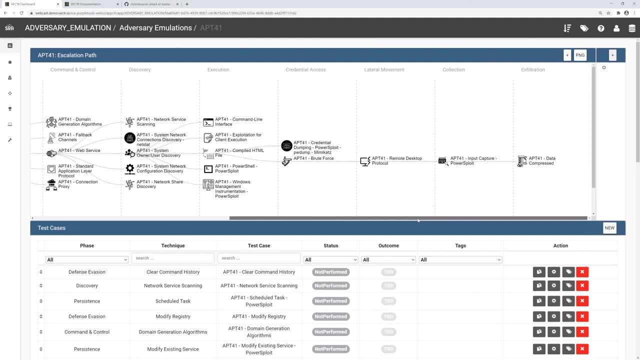 further enriched in the system. look on apt41 as an example. we haven't actually filled out any data here yet, uh, but you can see this is something you can directly just import from biters attack the CTI project on GitHub. uh, directly import this, at least an initial for an initial emulation plan for apt41. 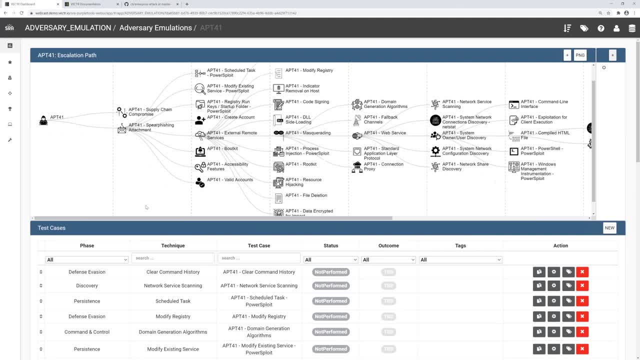 uh, so you can see there's quite a lot here. you know, in our experience this is a really great place to start. um, and George, you can probably speak to this, because I know you're going to talk about this in a few minutes, but I'm hoping to get some answers from you in the comments down here if you have any questions or comments or questions about the project. 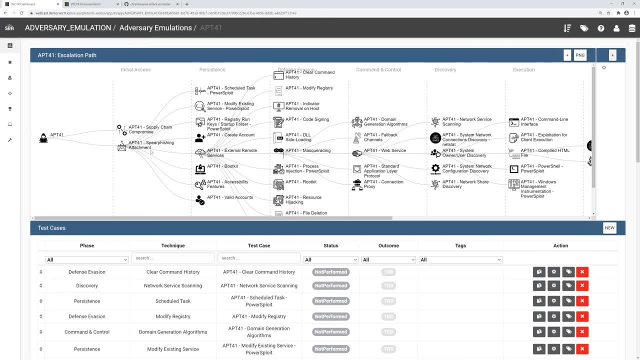 and George, you can probably speak to this, but you know a certain level of enrichment and maybe you know keeping it to really high priority. TTPs across some of these APT groups can be helpful, especially with some of the threat intel gaps or maybe some broader techniques that are good and relevant but maybe you don't want to tackle. 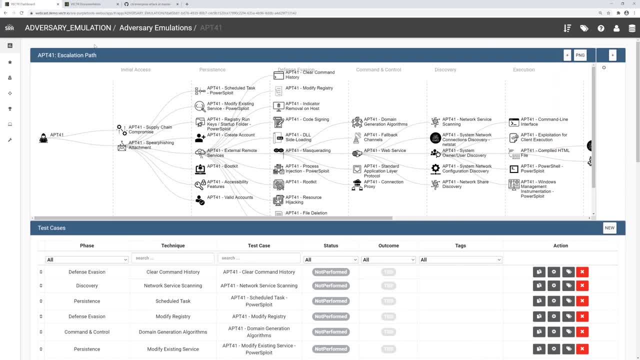 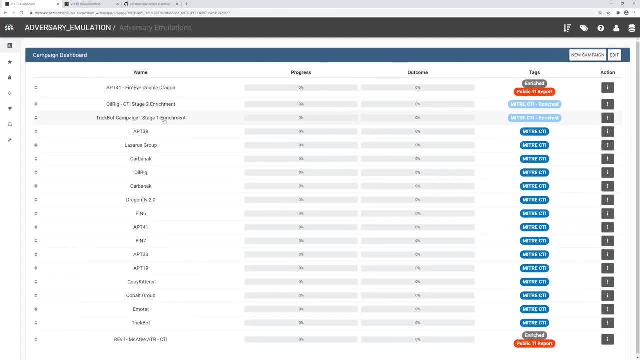 as part of your, your test plan. yep, and we actually got a question about that. actually, a prior student that took 564 was asking: you know you create this adversary emulation plan and do you actually have to stick exactly to it, like if we tried all the TTPs on the plan? can we deviate? and the answer: 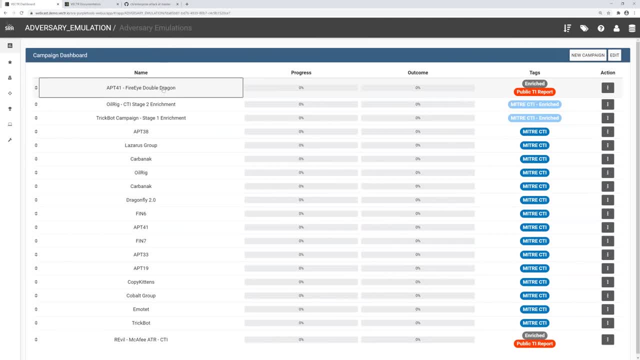 is of course you can, because an adversary would deviate as well. the adversary emulation plan is, before you do it, when you're presenting. this is what we plan to do, and if you go through it and you need to do another TTP, then it's as simple as just adding a new. 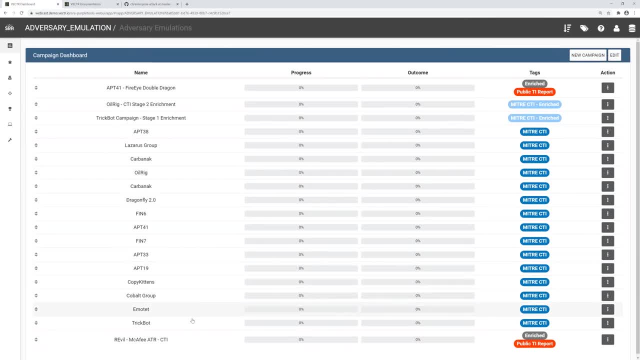 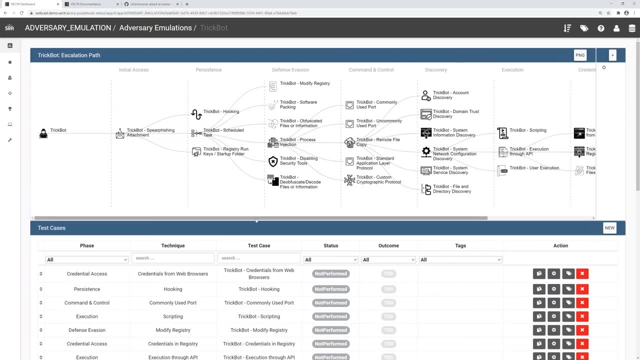 test case documenting it that you're doing this other TTP. that was not part of the plan- and then the result and whatnot, and it will add to this so you can actually have a. this was the plan and then this was the final- actually what we tested all through through here. yeah, thanks, George. yeah, and 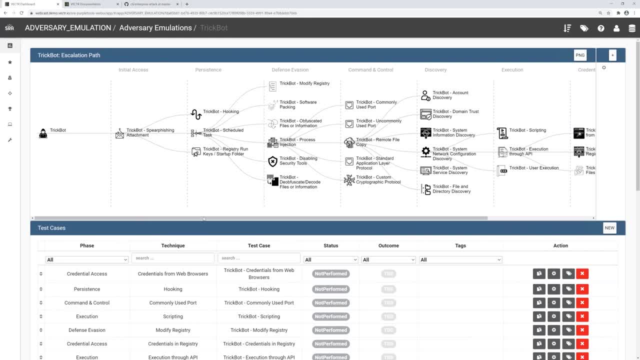 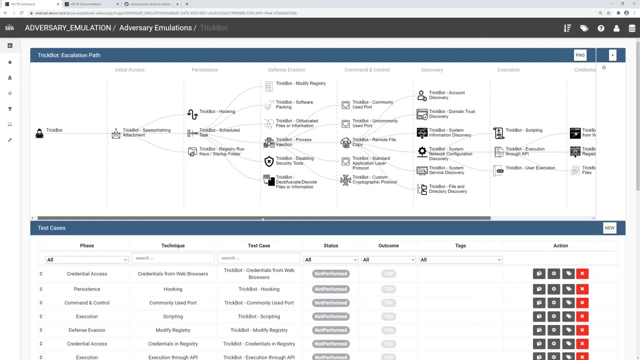 part of this too. what I'm showing now is just a TrickBot campaign that we've imported, so not everything needs to be specifically mapped to a threat group. it might be a very popular malware family ransomware activity where you also want to follow more of an adversary emulation approach to running through, and this is exactly. 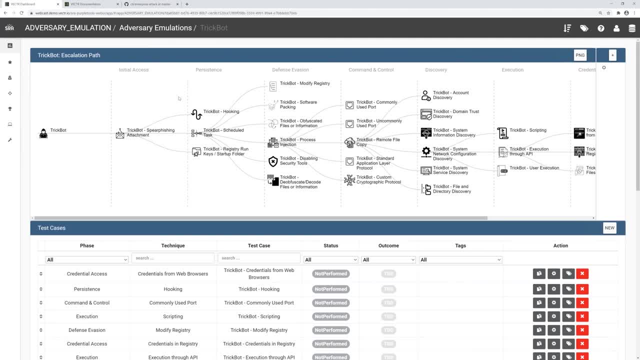 the type of campaign that you know your management might be asking about, especially with ransomware focus. so want to show some other use cases here. and then I want to just show you how to actually import, take advantage of vectors capabilities to import all of the TTPs that you might have. 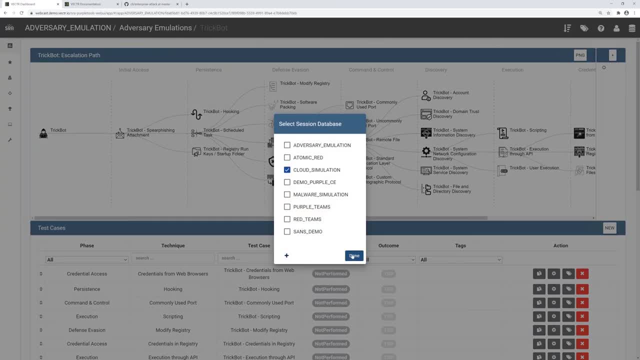 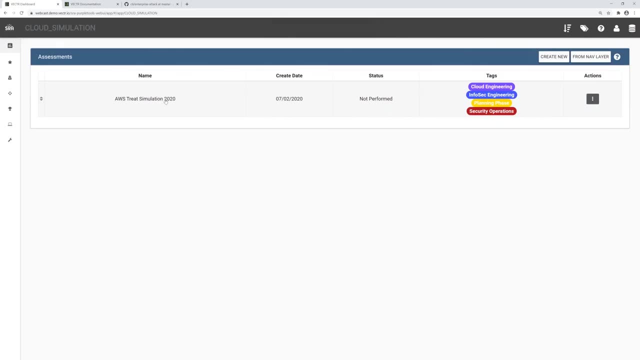 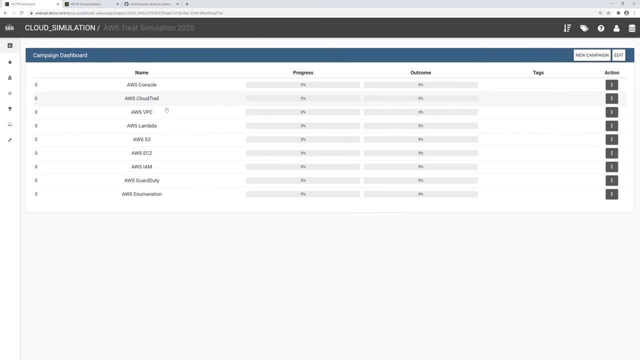 a lot of the CTI. one jump to this cloud database real quick just to show that you know vector is not, does not necessarily need to be all you know- 90% Windows Enterprise focus and attack aligned, but what we're showing here is just something we've created more custom. that is really just doing. 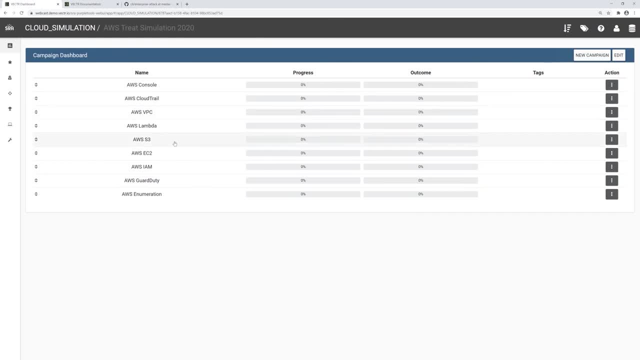 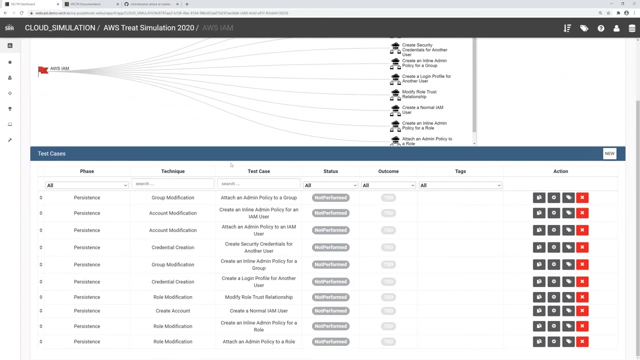 controlled AWS, like threat simulation, insider testing. you know, if somebody open exposed something to the internet would would you get the right alerts and shut that down. so just wanted to show that, if you're not doing direct testing, map to attack vector is a great platform for other types of other technologies, other platforms that you want to develop custom. 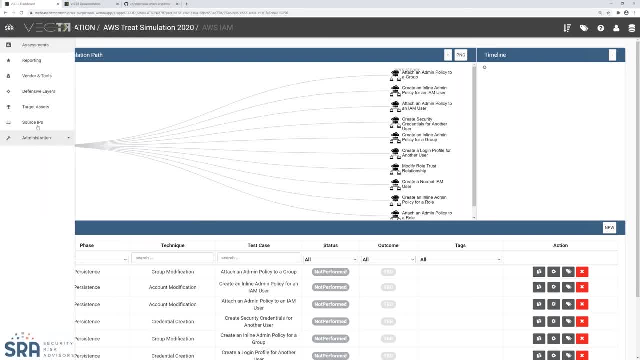 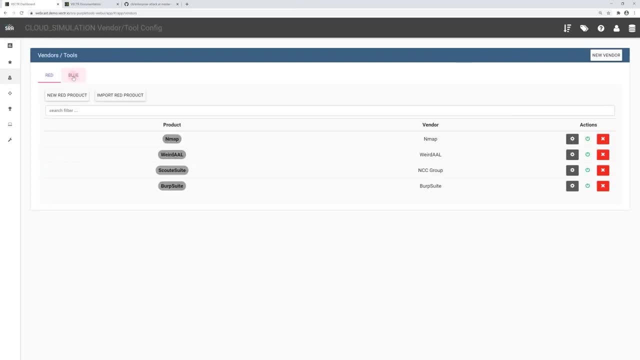 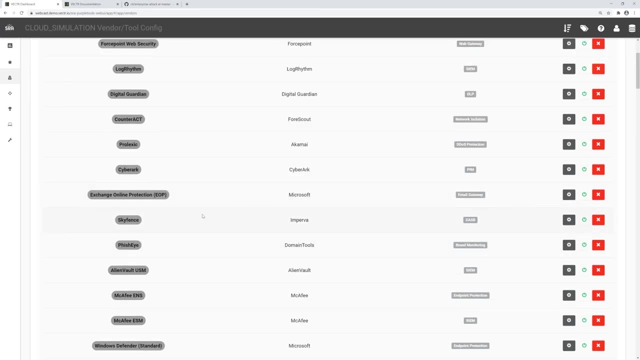 templates for so over here, just some of the things on the menu. vendors and tools won't get into too much of this, but this is basically where you would go in and customize this inventory to the major detection prevention, incident response tools in your environment that would dynamically show up in. 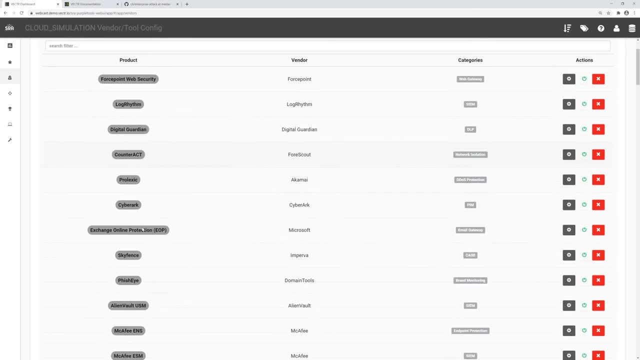 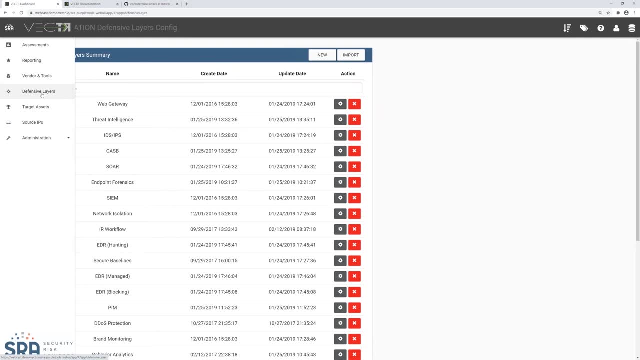 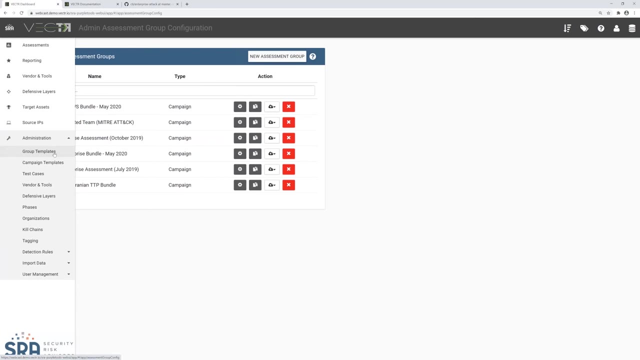 your test case panels. this is more of a kitchen sink version of that right now in our demo instance- defensive layers. so everything here has, you know, full crud capabilities. and then under administration, so this is where you manage those templates that you want to reuse and share with your peer groups. 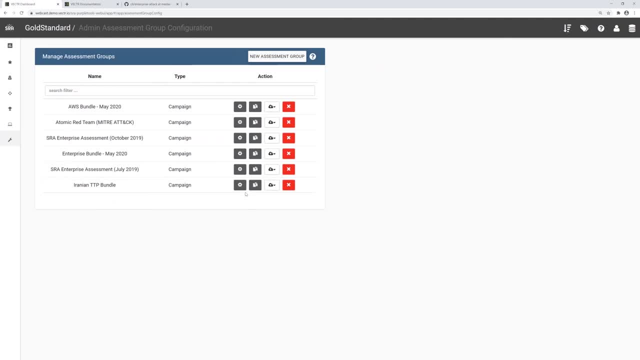 and and with a broader community. so you can see we have a number of George mentioned the Iran bundle. this is something we we actually released up on the, the vector website, on our GitHub. you can see in this Iran bundle we included a number- roughly seven different groups, as well as some US cert. 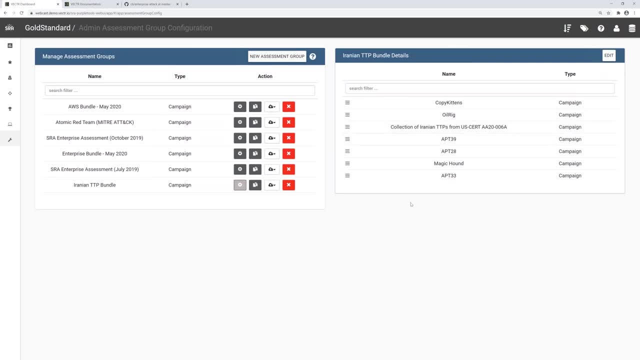 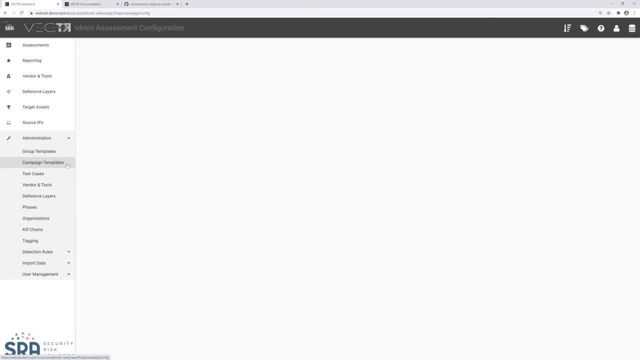 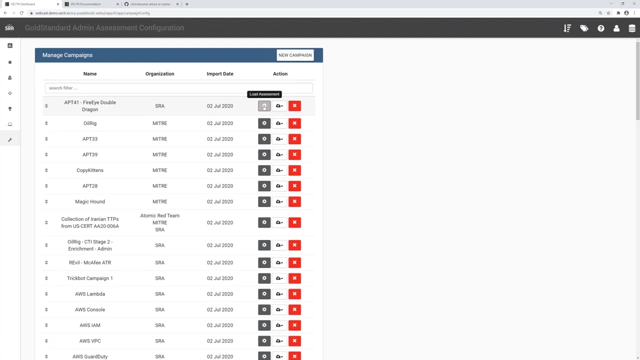 advisory information. it's just something you can grab and start to show coverage against potential TTPs- they're hitting your environment. then campaign templates: so really you can create a major group templates which will house any number of campaigns that you want to add to it. so this is the managed campaigns view. you can see this is just an example of APT 41, Double Dragon that. 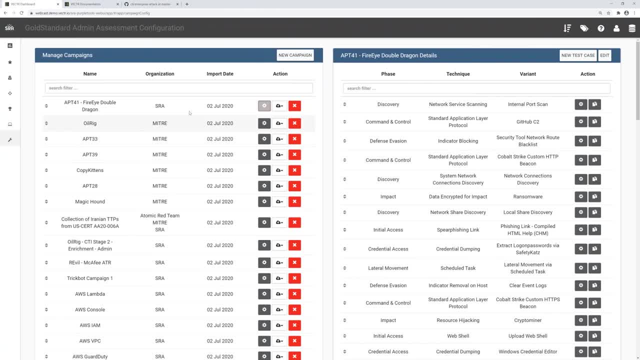 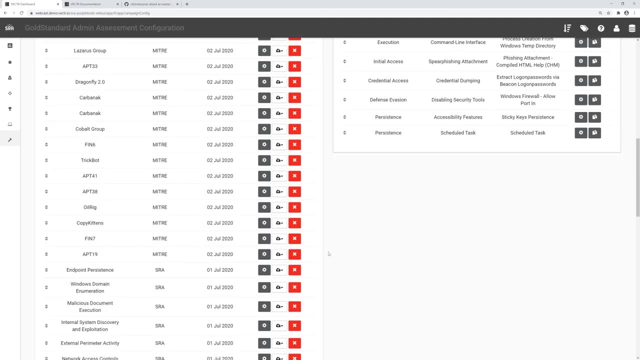 we actually created from a manian threat report. there's also good, good, minor CTI for this. there's different organizational sources for attribution so you can see which org created it. so this organization would probably be yours or you would use wherever you know the source of, wherever the 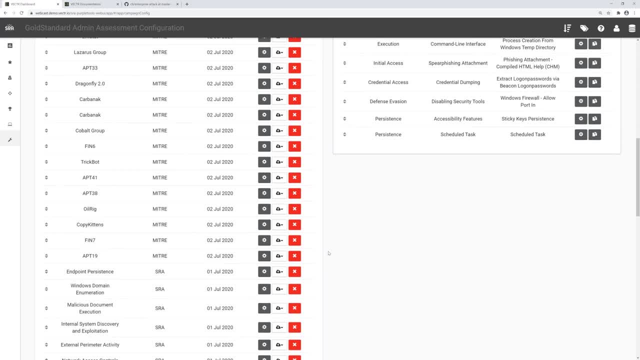 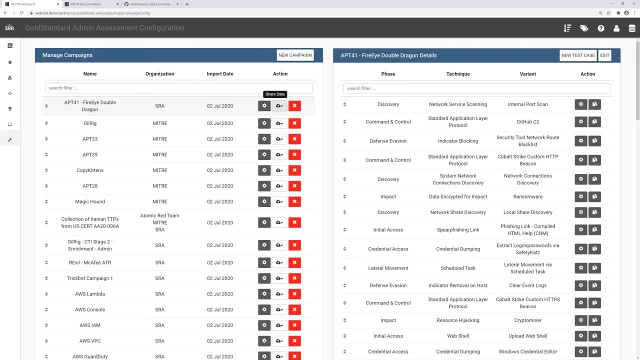 content came from anything. here, though, say something like APT 41, your T, your threat Intel team, your red team, has done a lot of enrichment on on the initial CTI import. this is something you can save off and actually just export as a JSON file and and reuse. so that's pretty, pretty powerful capability to to have that. 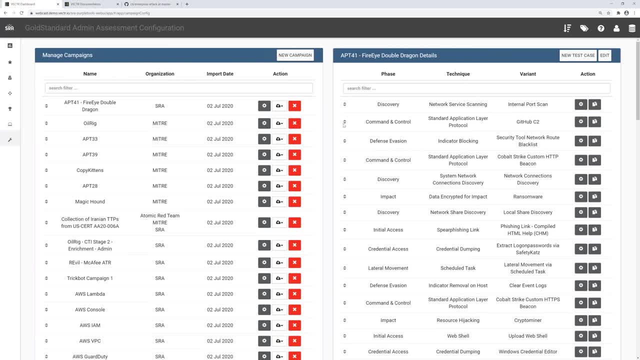 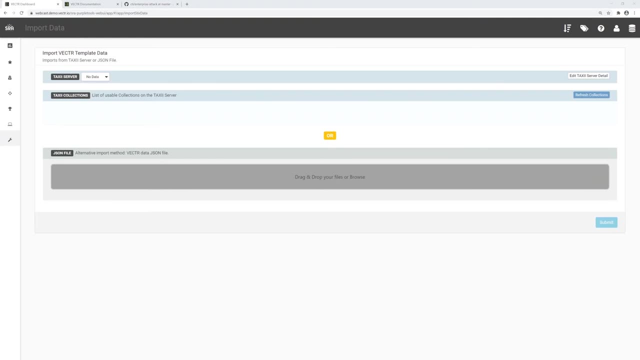 level of enrichment and looking to get a lot more Community participation into getting that and making it shareable via via a taxi server. but I wanted to show you the import data down here, so this is where you can actually bring in really good content. that's out there, so 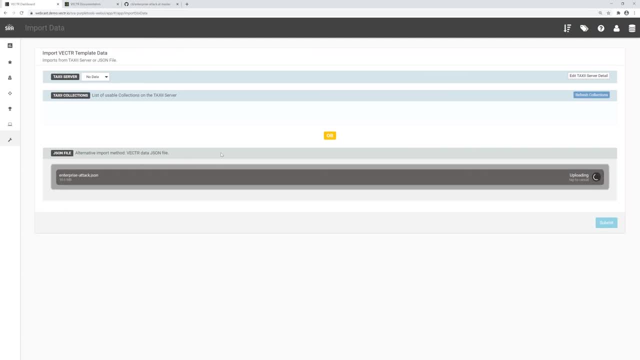 here. I'll just show you an example. we also have this, this dragon drop capability. what I'm pulling in now is literally just what we downloaded from the mitre CTI project under this Enterprise attack, so make sure you get that as well. you download the raw bundle, drop it in, submit. now what this is doing is. 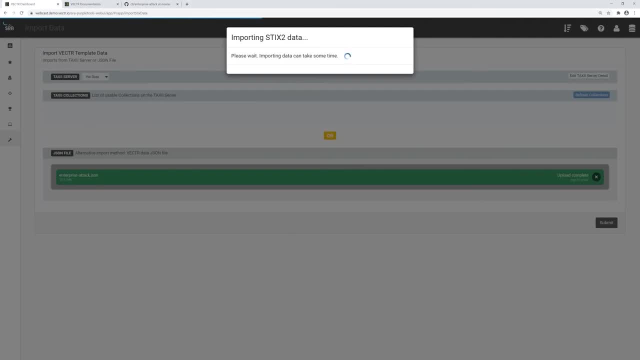 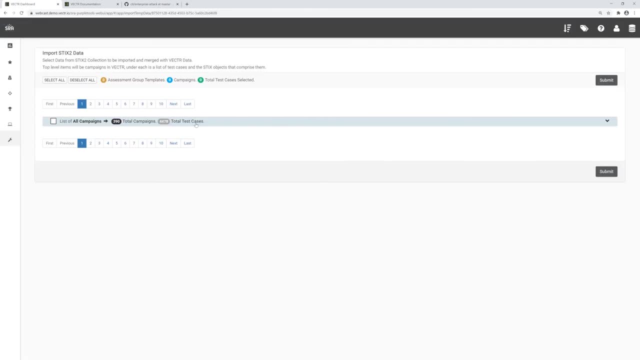 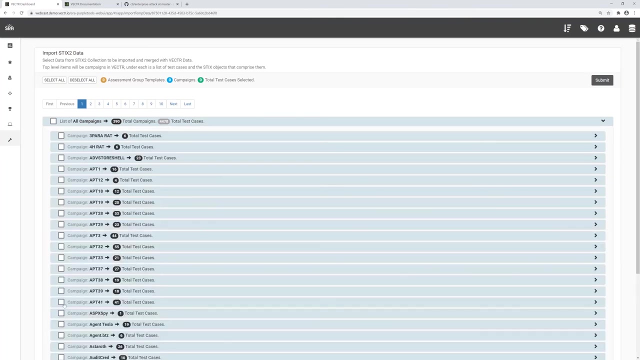 actually parsing out the entire sticks to bundle that MITRE uses to to represent attack through various sticks, objects and relationships. so you can see this is quite hefty. we've parsed this out in the 390 different campaigns and over 4,000 test cases. what you can do is you can certainly import everything if 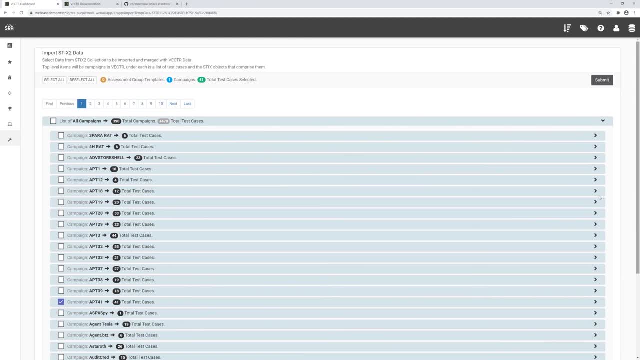 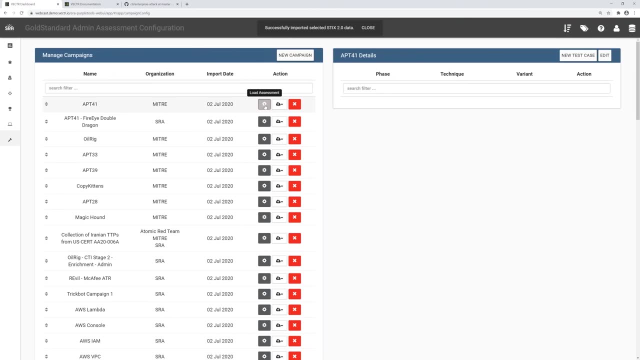 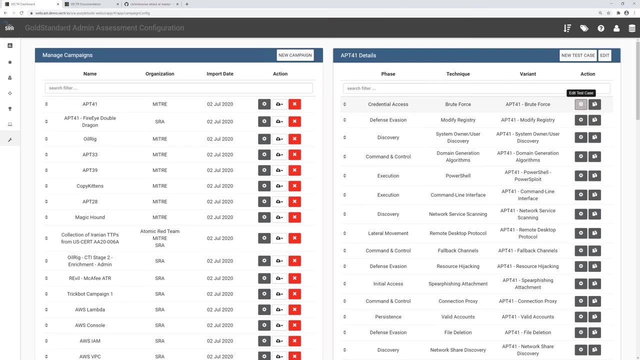 you want all those templates or you could just be very selective. we'll pick something like APT 41. hit submit. here is our new campaign. you have your import date. this was just brought in from MITRE. you're able to just preview it here. this is now a full template that you can create an assessment. add this template. 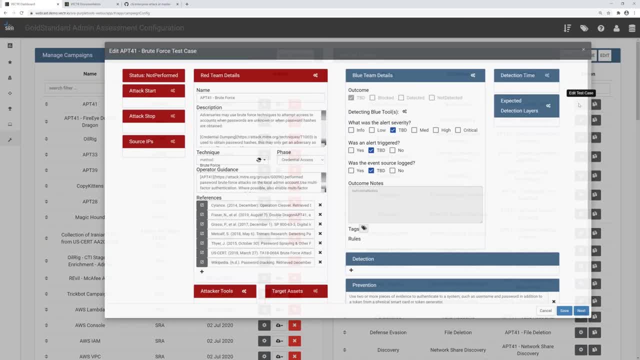 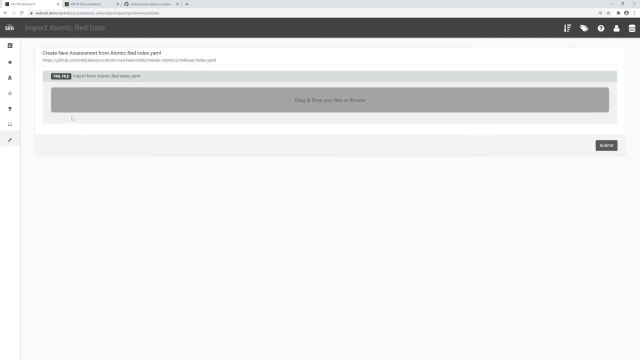 and start with your- your testing and tracking. something we actually recently added is a new template that we're going to be using in the next couple of years. if you've been using vector for a while, we did have like an older atomic red assessment template in there. we've recently made that path much better so. 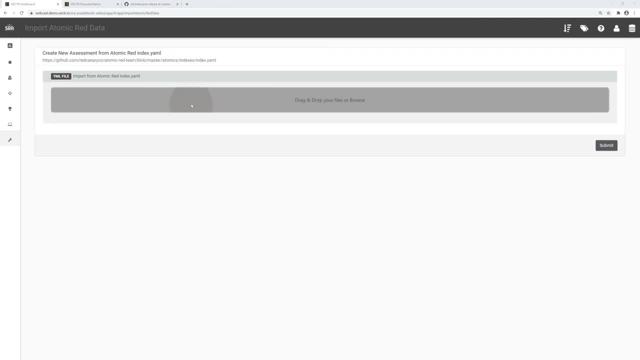 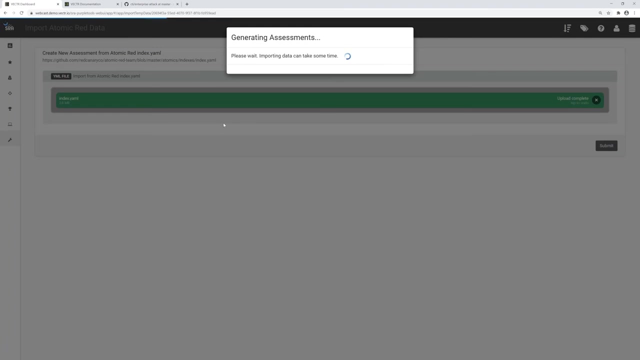 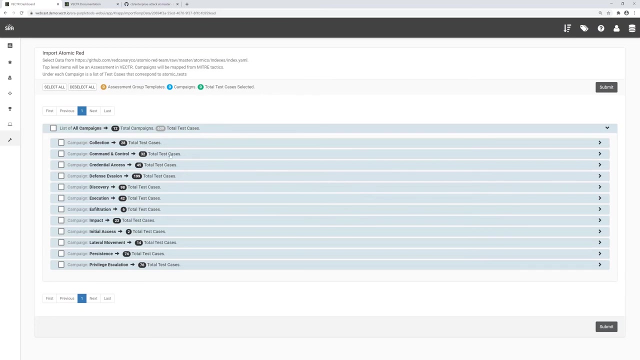 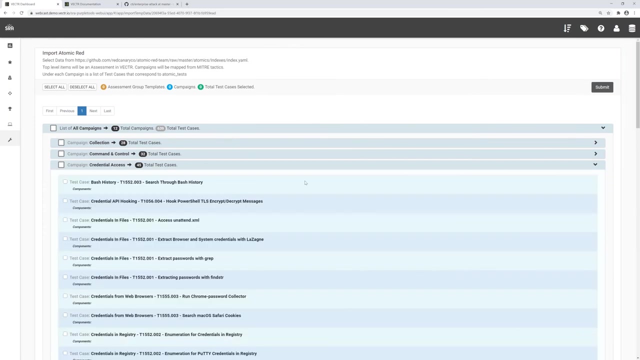 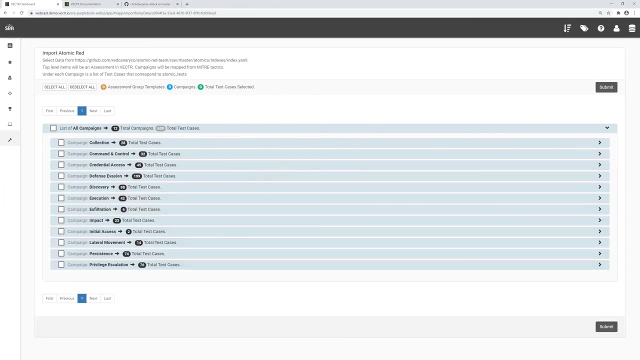 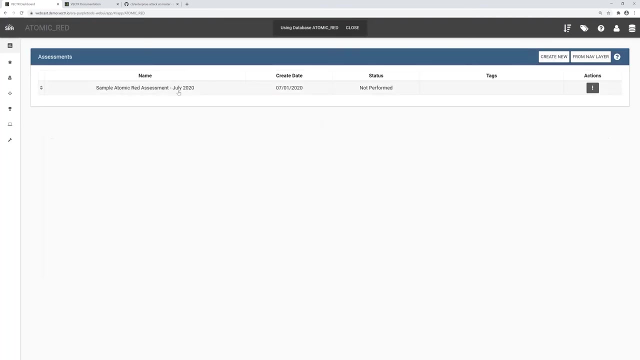 now you can actually download the latest atomic red index from from their github: import it, click, Submit you. I can show you what that looks like. just jumping to the atomic example, I think I have a database here atomic red, so if you're just looking to get started with 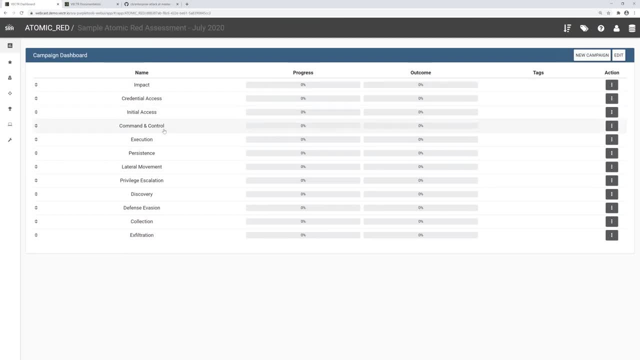 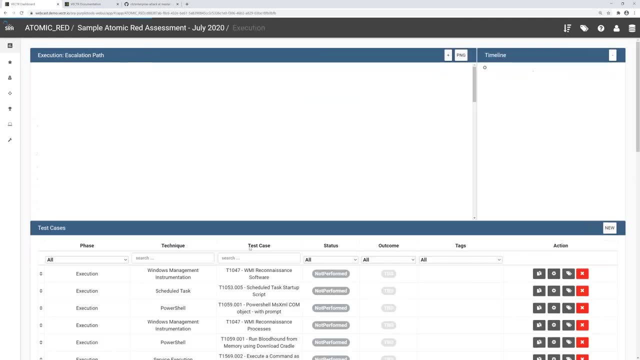 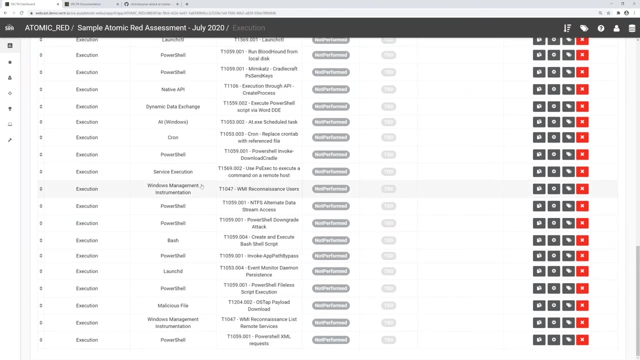 general attack alignment. you can see all these campaigns are really broken out by by tactic for tracking so you can go to something like execution and and you have a very large number of test cases that you can start to run through. but the best part of this is when you know there's great updates to. 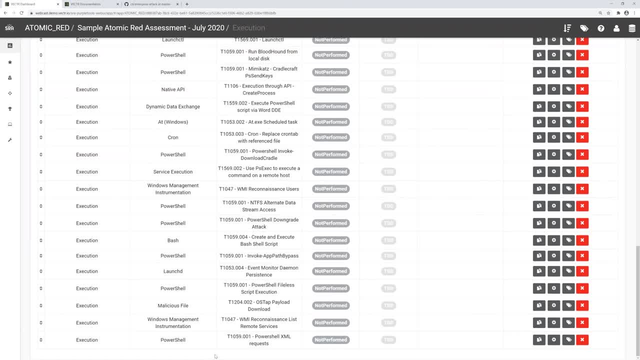 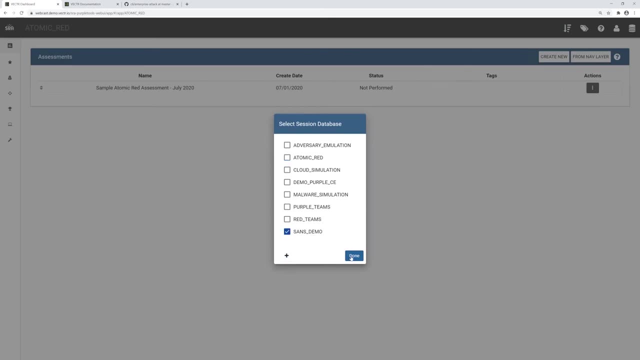 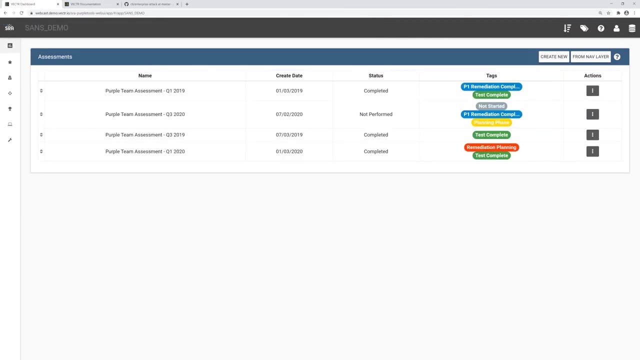 atomic red. a month from now, you can also drop in that template and benefit from those updates in your your assessment data and vector. you, you, you, you. you jump back to our sans demo database and, George, I don't know if we want to do a time check here for about five more minutes. there's a few questions queued up. 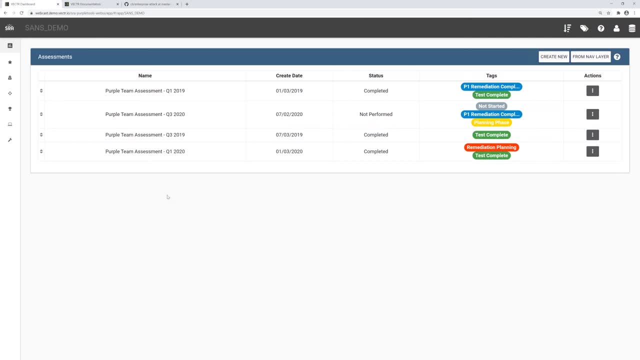 for you and if you have more questions, please post them and we'll answer those in about five minutes. great, and just to just to tie that together. so we're back in our sans demo database in terms of: okay, how do I actually create content from all these great templates that I've? 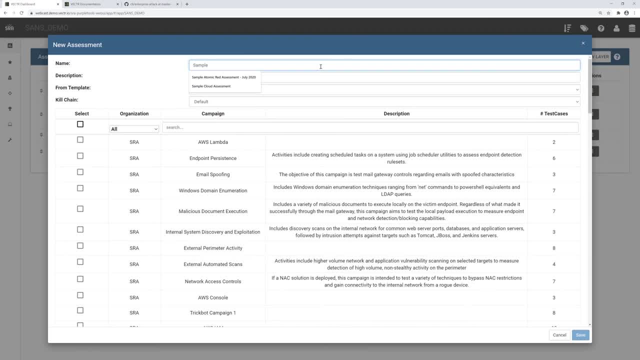 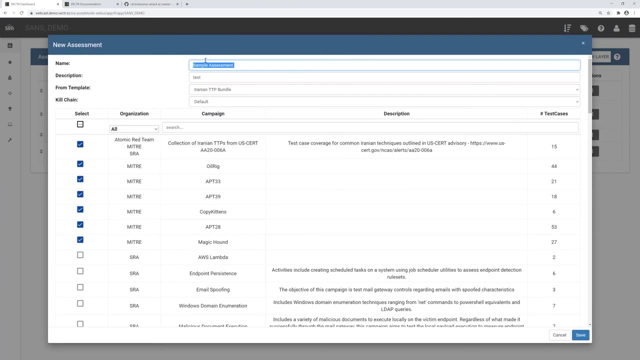 brought in, you can create a new sample assessment. call a test from this template. you can now pick from an existing assessment group. so, George, going back to your example, we'll look at the Iranian TTP's. we have this pre-built template that we brought in. you can see at the top here we have a list of 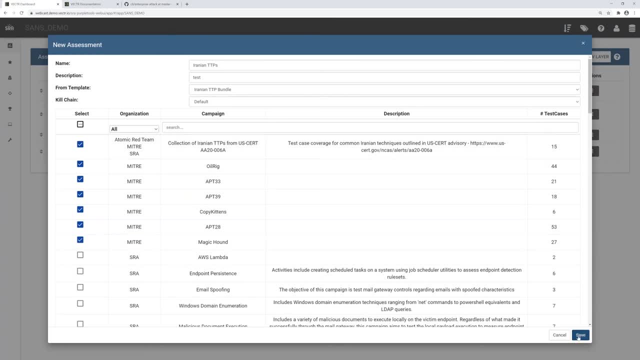 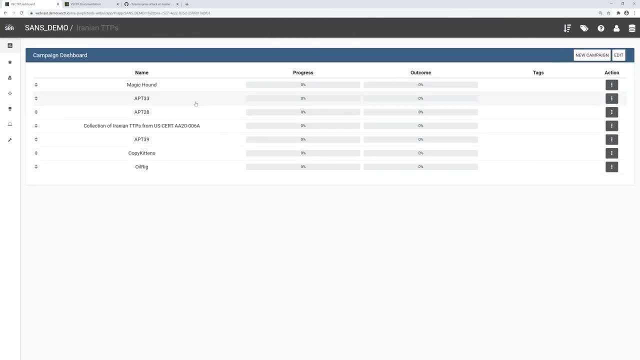 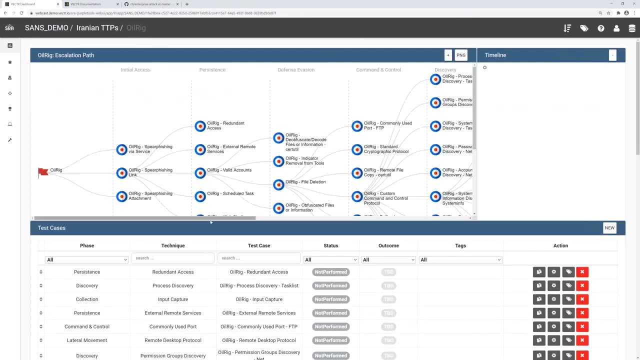 campaigns that are already a part of that group. so it's really as simple as that, and now you have a structured way to start assessing against these different threat groups and breaking it up by by group. we also added a lot, a lot of new icons to the system, so you should no longer be seeing the big, big red. 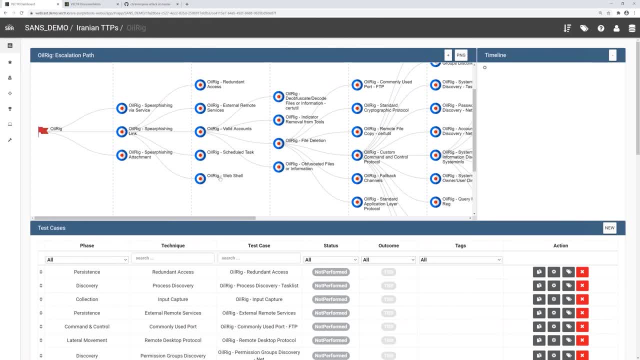 bullseye everywhere. so every, every technique will have a default icon, and we're working on adding some new ones to that as well. but in a nutshell, that's how you would just go from just simply downloading miters bundle, importing in the vector, having some initial emulation plans that you can start to work with. 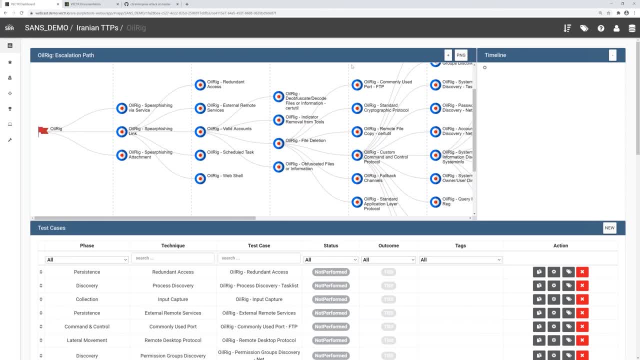 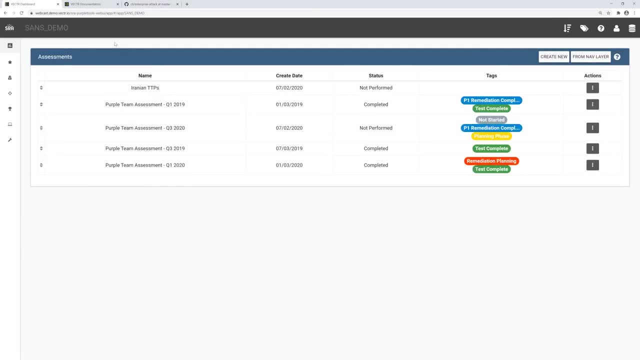 and further enrich. that's awesome. um, can you make me a presenter again? so I show the last slide here and we'll jump to you Q&A again. if you have questions, please post them on here. I think I've answered a lot of them. I have at least two here for Phil, so you will see a screen up. 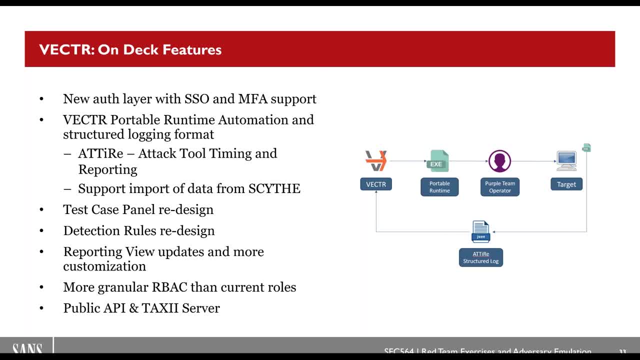 right now one of the questions is around multi-user and I answered it already, but But for everyone else that's not reading the Q&A, the question was: let's suppose you have three red team operators in a cybersecurity area in a company. Do you recommend having this tool installed per operator or have a server? 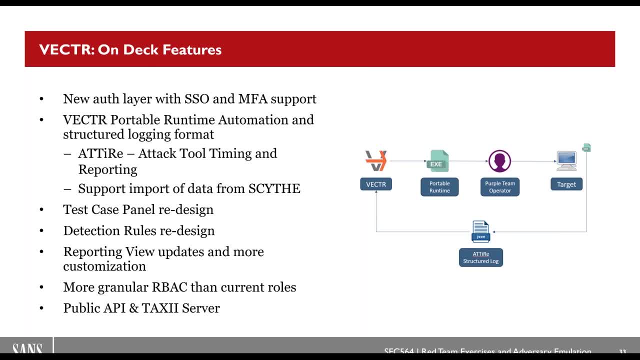 And is there any multi-user and multi-tenancy availability on Vector? Yeah, that's a great question. So we're actually. you can currently create multiple local users under the user admin If you're an admin role in Vector. So those are still local in scope now with some of the RBAC that's built in. 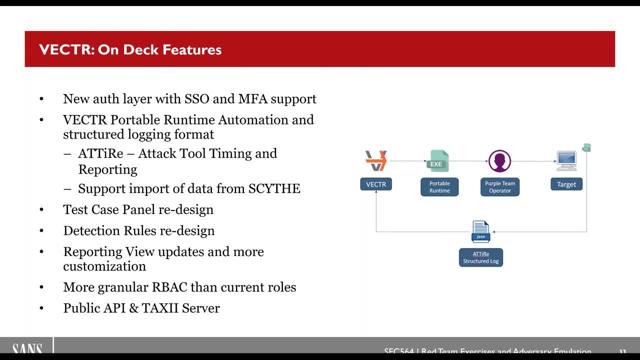 We are very far along on a new auth server implementation that has full SSO, So that will support pretty much OpenID Connect and SAML flows. So it really should integrate with any major IDP auth flow that you're using And that will allow you to come in as a federated user. 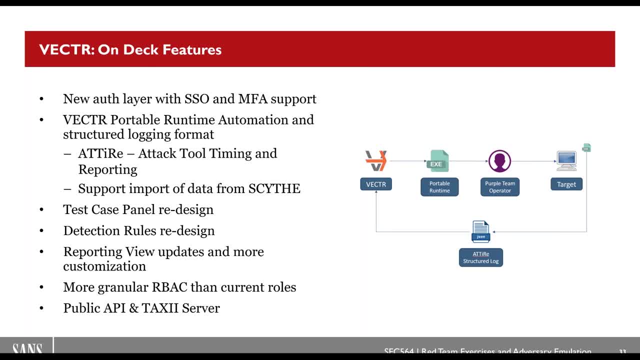 And External versus local user and also, you know, additional role, role capabilities and within Vector itself. So the interesting part about that is we actually have a pretty, pretty rich admin panel to configure the SSO settings for your environment. So we're hoping a lot of folks can take advantage of that to get up and running and 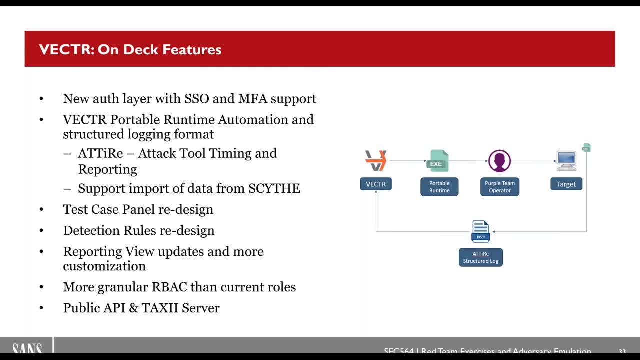 Also, importantly, be able to leverage the multi-factor authentication that's already required from from your IDP, And we're also working on a local MFA solution too, if you prefer to just keep your Vector's local Vector users local, not not have not use all that. 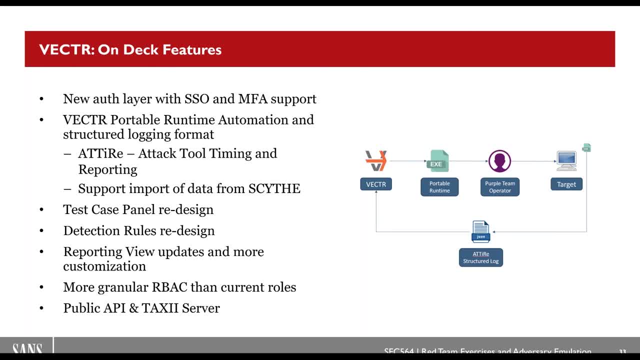 But that's a great question And I don't. we don't have a exact ETA, but the development is pretty far along, Just needs a little bit more testing- Awesome. Another question here is: I saw Vector's listed as free. Are there plans to make it open source? 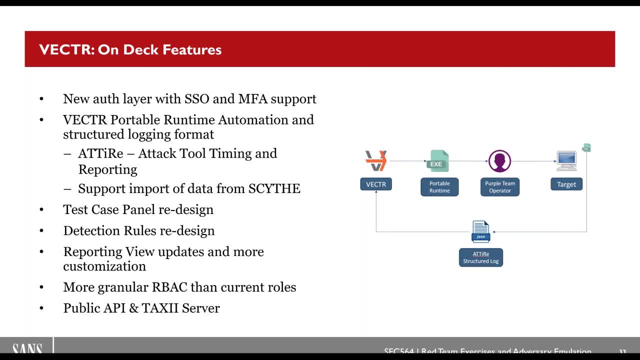 And then, what really is the difference between free and open source? Another good question- And this has come up a lot to the actual Vector- is a free, Free platform. The code is not currently open source. So you know we're we'll debate if we ever want to make. 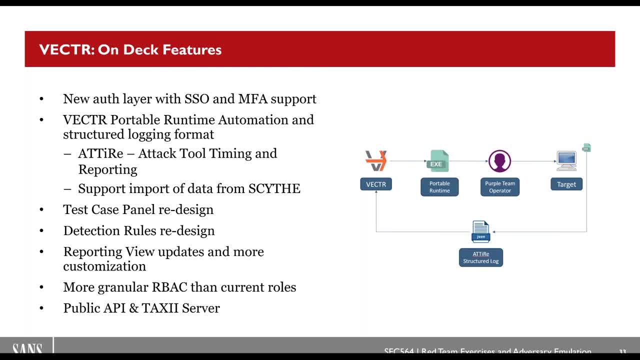 Actually release The source code if that's something we think we can manage: community contributions and and still maintain the software quality that we need with an open source project and stability. But yeah, currently you know we don't have plans to restrict any features of Vector. 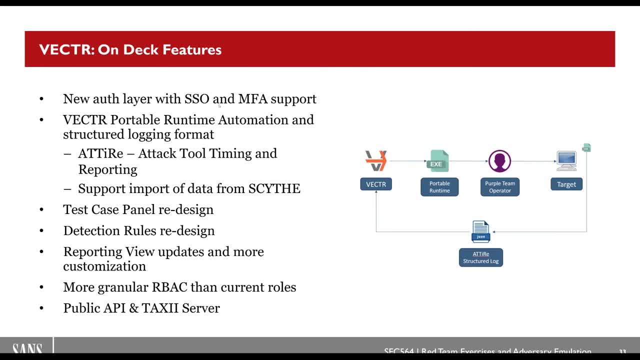 Keep the platform free. use technologies like Docker and things that anybody can deploy, But yeah, yeah, the free platform, not, not fully open source. We can't, We're not going to be able to do that. Excellent, Got another question here. 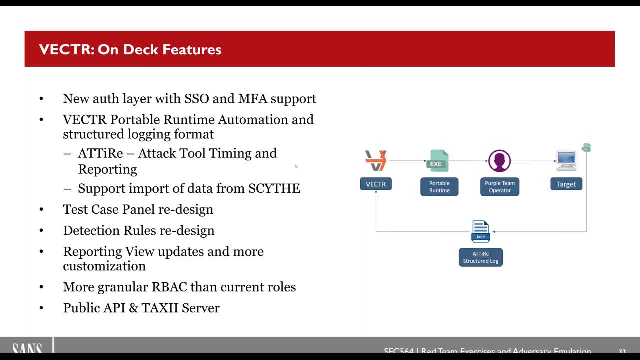 I'll give it to you first and then I'll fill in blanks on my experience. But the question is: do you see using Vector during red teams taking more time than normal to go through and document every step? It seems like a lot of information you need to supply into vector. 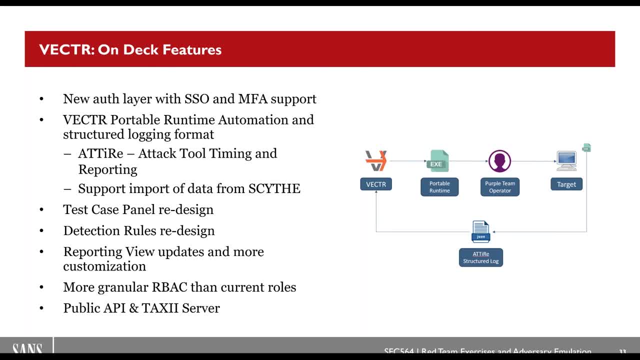 Yeah, that's a good one. Yeah, So we we've used vector in the past to basically import, like transcribe historical red team reports. Yeah, that's a good one. Yeah, so we we've used vector in the past to basically import, like transcribe, historical red team reports. 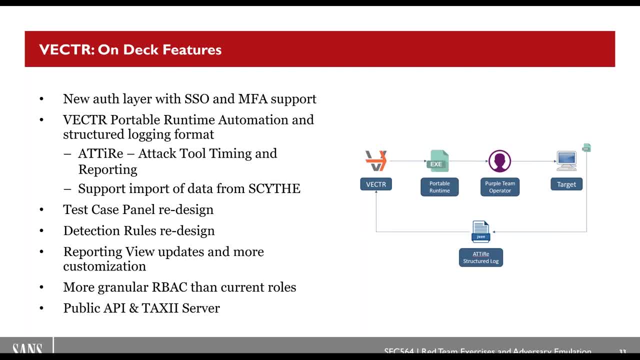 And that's not a super-fast process. There is more work required. So, unless you've already done a significant amount of planning, like put together an initial red team plan, emulation plan, mapped out different phases of the red team which obviously you're going to need to deviate from by the nature of a red team- yeah, that is something. 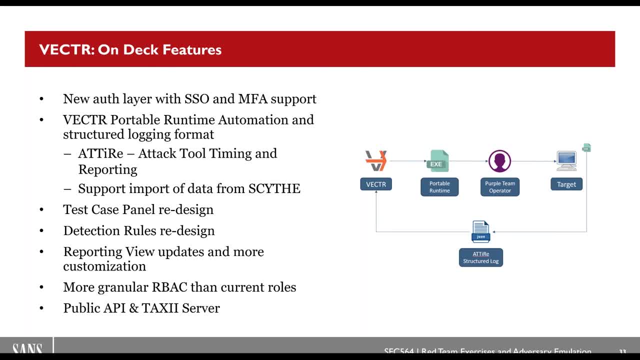 that certainly could slow progress on a true red team engagement, where you might want to – if you can't do it in real time, you should be able to at least capture the summary of TTPs coming out of that that you want to focus on. 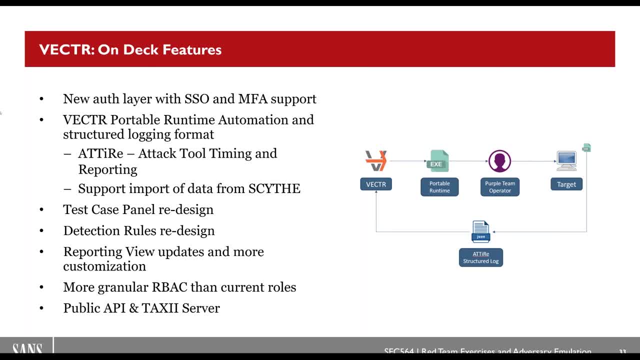 So what we've done, too, is when we've done – our teams have done red teams and we want to bring it in the vector. we don't always exhaustively document hundreds of different activities that we did, But we will bring in key escalation paths that led from, you know, initial access, all. 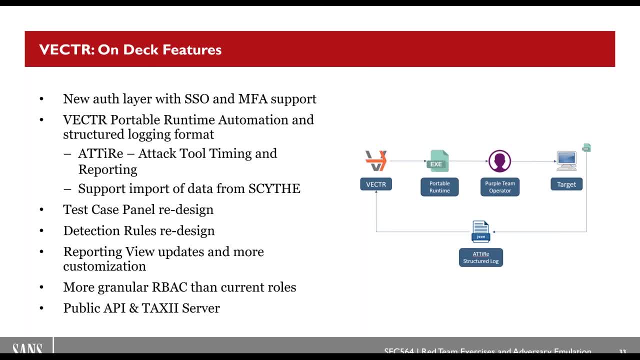 the way to compromise data infiltration, whatever the flag for. So we've been a little bit more selective with- okay, let's really just extract the high-value TTPs that we need to get more visibility into, or just vulnerabilities and defects that 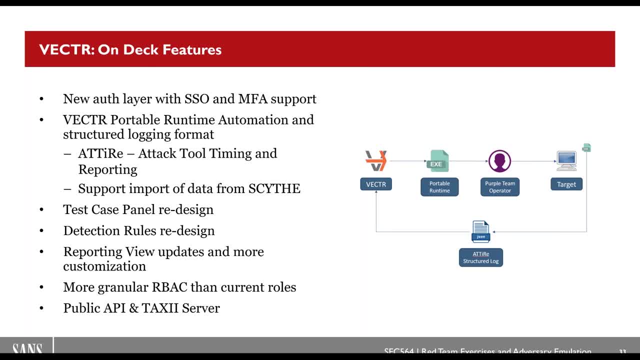 need to be fixed. George, you can probably talk about this for a while. Yep, So great, great question. A lot of red teamers don't like the ending part because of the reporting and then having to go back and looking through everything. you did, right. 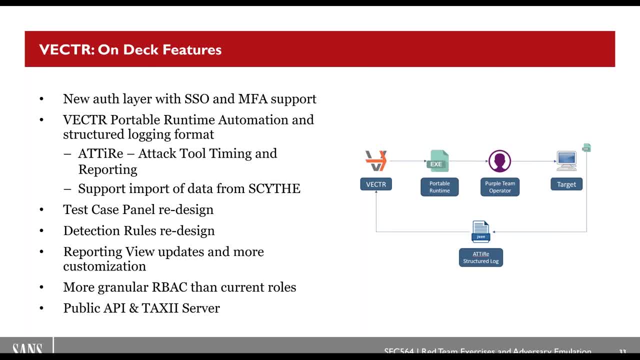 A lot of these C2 frameworks and one of the columns we look at in the C2 matrix is logging right. So personal opinion but I think a lot of red teamers share it is if you spend the time early but in the planning phase – and a lot of people think that red teaming is. 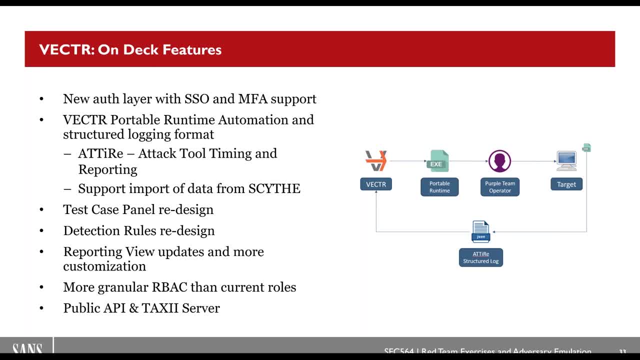 just the testing. The whole planning phase actually sometimes even takes longer than the actual testing, But one, as Phil said, it gives you a good adversary emulation plan that you can present before it gets approved, for example if you need budget or if you need to prove that. 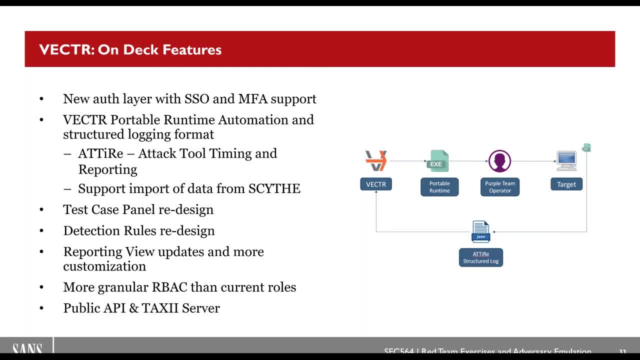 you know, if you're a consultant, that you actually have a plan and you're not just, you know, going to go break stuff. So doing it early is great, especially in red team engagements, but really the value that we found was in best practice. 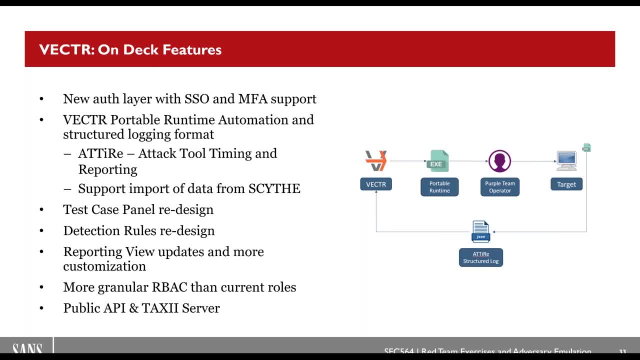 We found was in purple team exercises, Because when you're planning the TTPs that you're going to emulate in the exercise, you don't want to spend time or do TTPs that are going to be blocked or do TTPs that 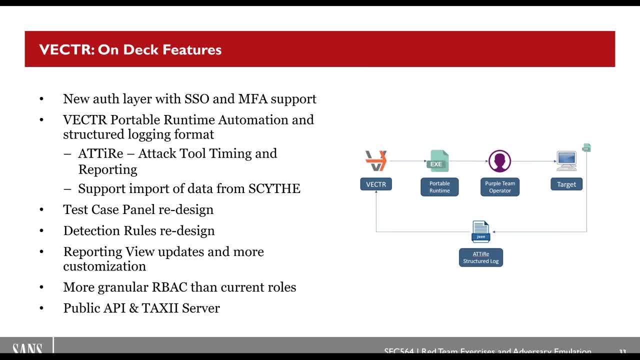 have absolutely no visibility on. So, as Phil showed, if you create the plan, you can have the expected tool and behavior. So we kind of tabletop it with the senior managers- the SOC manager, the incident response manager- As we choose what to do. 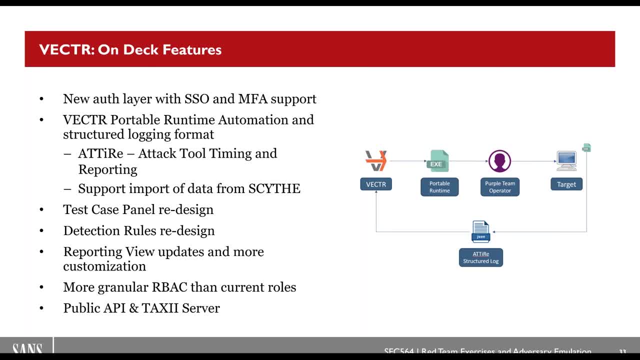 What TTPs we're going to do, live during the purple team engagement, And then that's testing assumptions, right? A core of red teaming is we assume that this is going to get blocked. You have mapped that as such and then you go and test it. 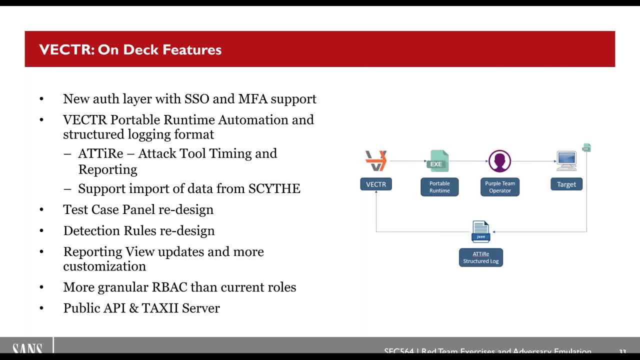 Doing and documenting. the result is much quicker and less time consuming if you created the plan ahead of time. So I would also say always, always, always, do it ahead of time. And with that It is right at the end of the talks. 1130 Eastern here. 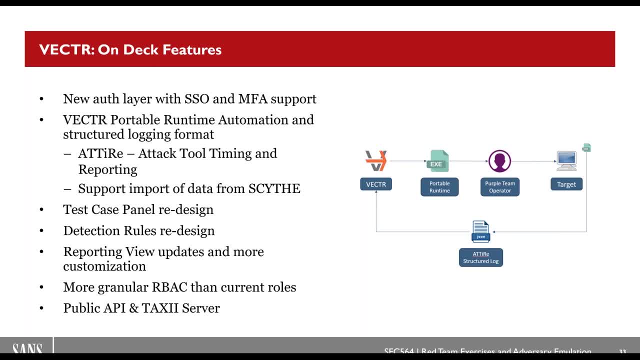 I want to thank you, Phil, for coming on and all the awesome work you've done on Vector and continue to support it as a free tool. We all appreciate that, And I believe Carol's on to say some closing statements. All right, Thank you so much, Phil and George, for your great presentation, which helps bring this. 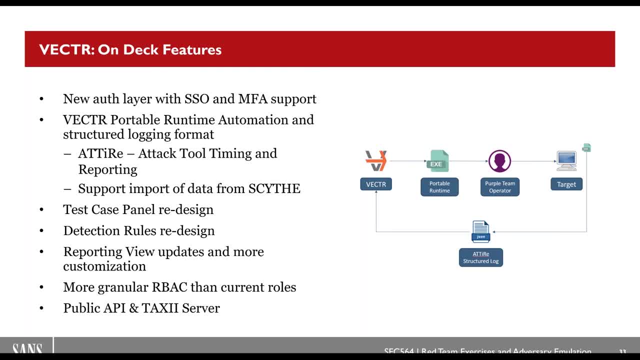 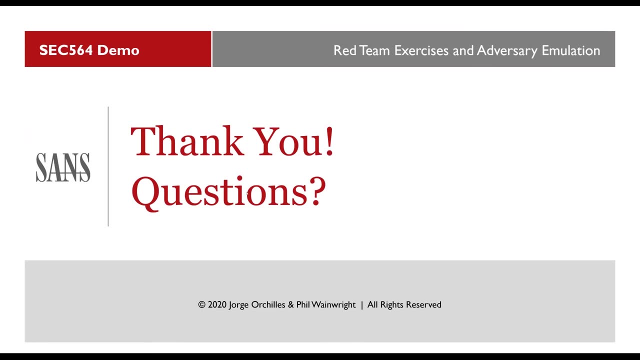 content to the SANS community, To our audience. We appreciate you listening in. For a schedule of all upcoming and archived SANS webcasts, including this one, please visit sansorg forward slash webcasts. Until next time, take care, and we hope to have you back again for the next SANS webcast. Thanks everyone. 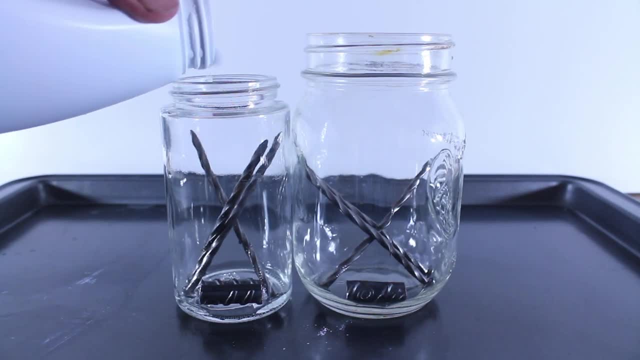 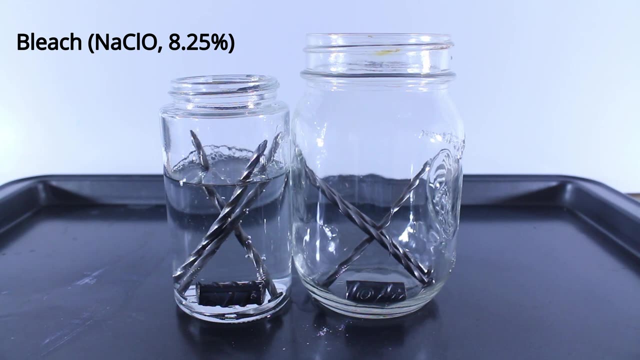 So I wanted to film some iron corroding. I thought it would look nice on camera. So I figured I'd take some iron nails and a piece of steel rebar and put them and react them with some household chemicals. On the left side we have common household bleach, which is an oxidizer. I figured that would work well to oxidize iron and create iron oxide. 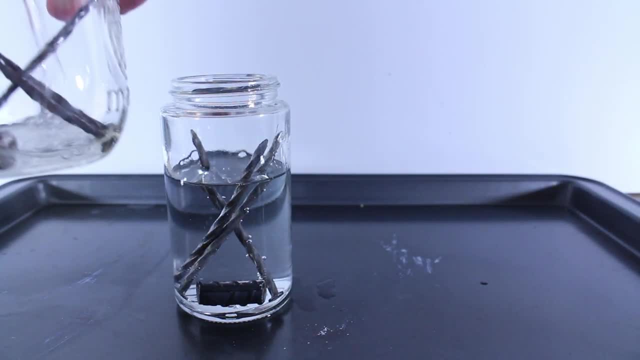 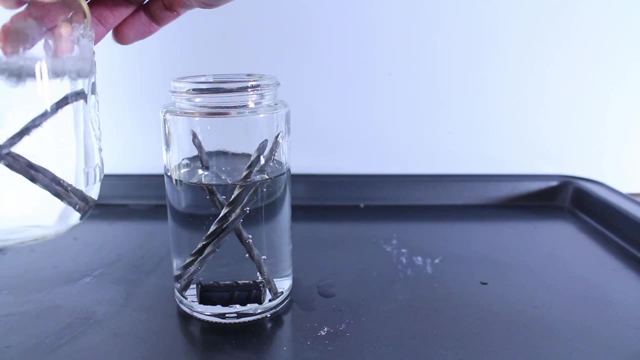 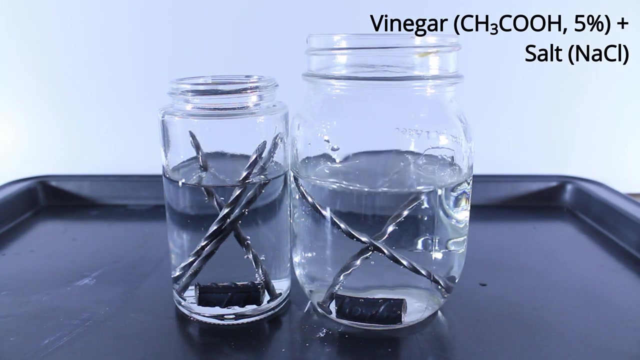 And on the right, I figured acid is a corrosive agent. A common acid I have available is acetic acid or vinegar And I figured salt water also helps corrode iron so I figured that would also add some salt. So the reactions: I don't really know what's going on. I don't have a very strong background in chemistry but it does produce some interesting visuals for the camera. 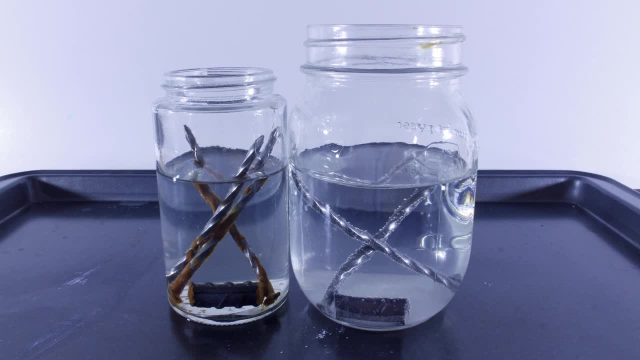 Edited from a blank ikke video. It says on one of the videos that I uploaded in my YouTube channel that I click onto the screen. This was my gloss And I am going to try to directly highlight it in my video because this is tasty hot and it makes me feel closer to an ordinary-suitable Bauhaus regarde. 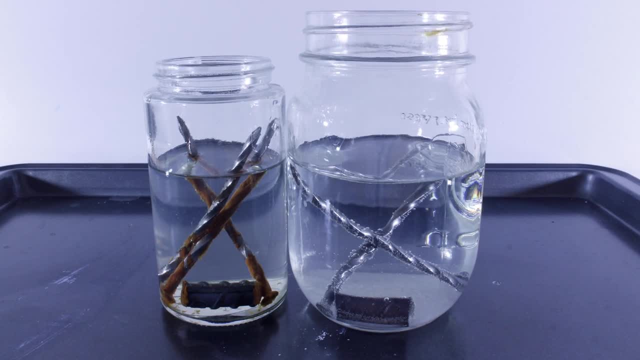 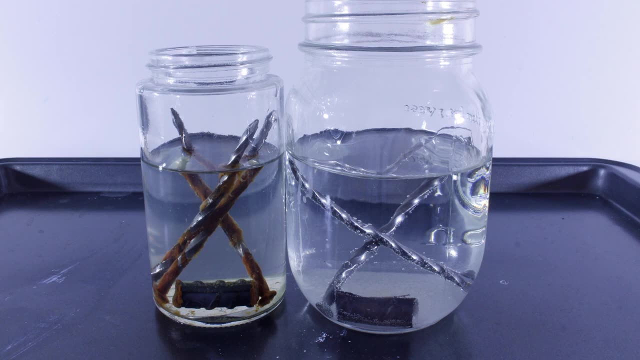 For now, let's go: 3: 1, 1, 2, 3, 4, 5, 6, 7, 8, 9, 10, 11, 12, 13, 14, 15, 16, 18, 17, 18, 19, 23.